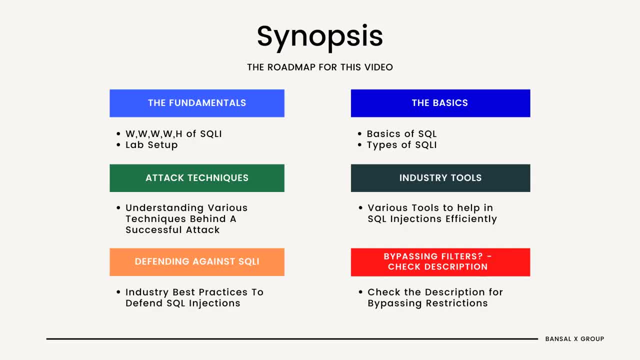 Let's see what you are going to cover in this course. So there are five sections in which this course has been divided in: The fundamentals, the basics, the attack techniques, the industry tools and defending SQLI. In fundamentals, I'll cover the what, when, where, why and how of SQL injections. 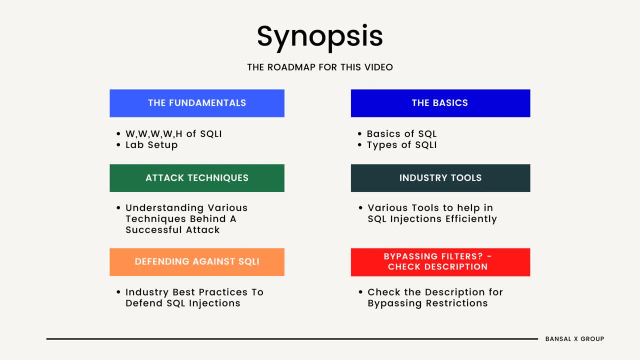 And I'll show you the lab setup that you will need for this course. The basics will cover the basics of SQL. Again, it's not basics of SQL injection, it's basic of SQL And then types of SQL injection. After that we'll move on to the attack techniques, where I'll show you various attack. 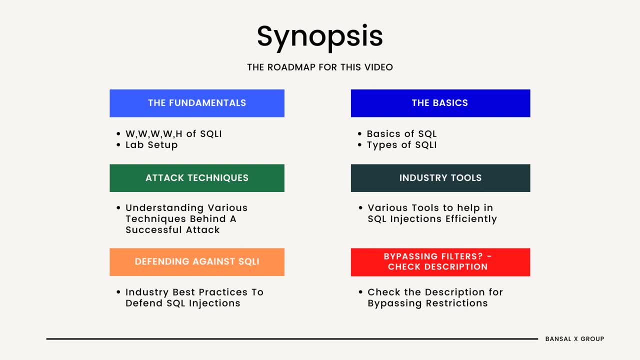 techniques that you can implement in this world and it's completely hands-on. Finally, I'll show you how to use industry-specific tools to use SQL injections and to leverage them efficiently and effectively, And we'll wrap up this with a lecture on defending SQL injections. 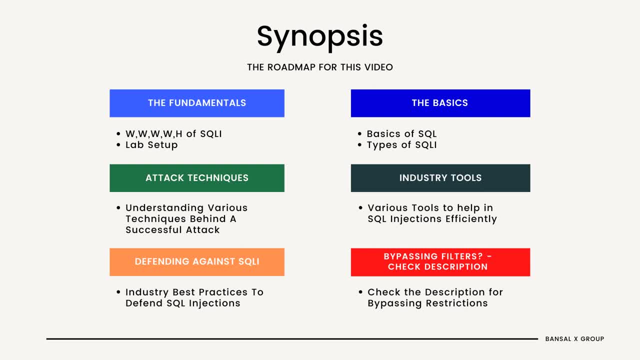 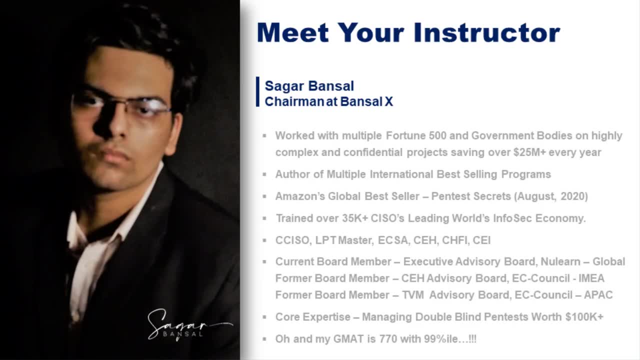 where I'll show you the best practices that you should be following. And again, I'm not a programmer, so don't worry, I'll not show you the coding practices. I'll show you what the real stuff is. Let me go ahead and quickly introduce myself. 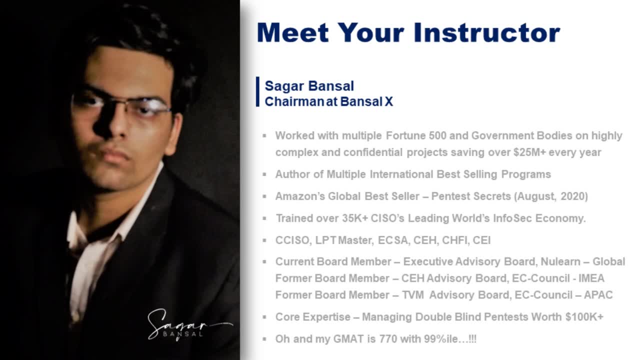 Experience-wise, I've worked with multiple Fortune 500 companies and government bodies on highly complex and confidential projects, saving them over $25 million every year. Last year, we saved over $72 million if we combine everything. I have authored multiple international best-selling programs as well, as I am the 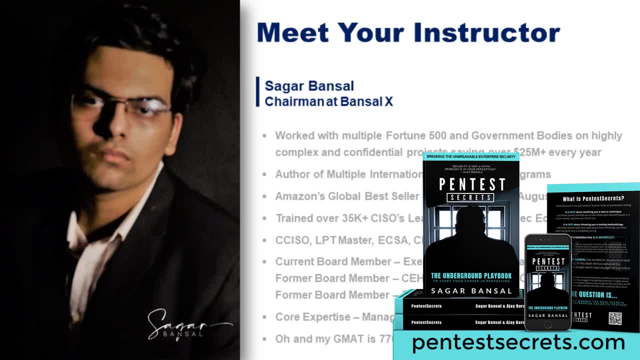 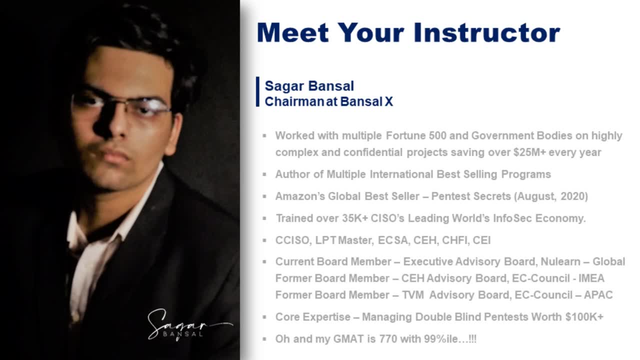 author of the book called Pentest Secrets, which is an Amazon's global best-seller. I have trained over 35,000 CISOs who are today leading the world's infosec economy. I hold the CISO, LPT, Master, ECSA, CEH, CHFI, CEI as some of my EC Council credentials. 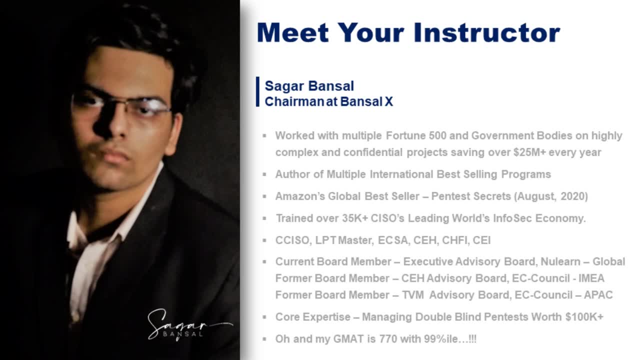 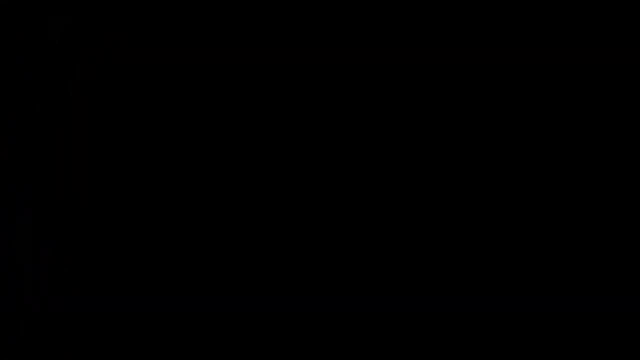 I have been a former board member for CEH Governance Board for India, Middle East and Africa region and KVM board members of EC Council. I also have a PhD in implementation and UX course in Asia-Pacific region. My core expertise is in managing double-blind penetration tests. 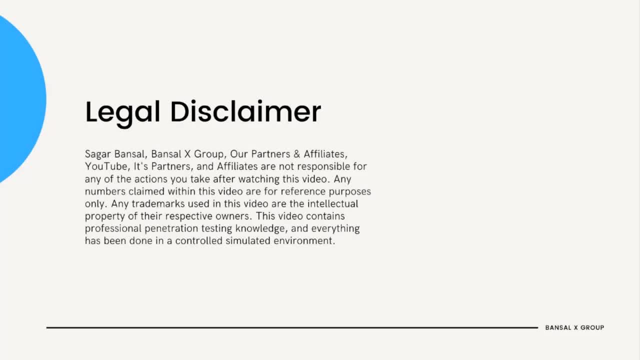 which are budgeted at least $100,000 or above. Here is the disclaimer: Sagar Bansal. Sagar Bansal Group of Companies are partners and affiliates. YouTube. its partners and affiliates are not responsible for any of the actions you take. 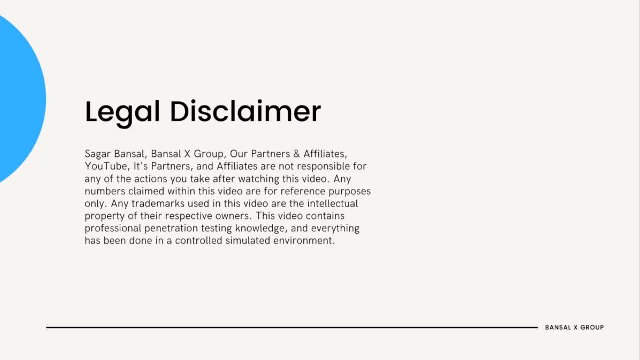 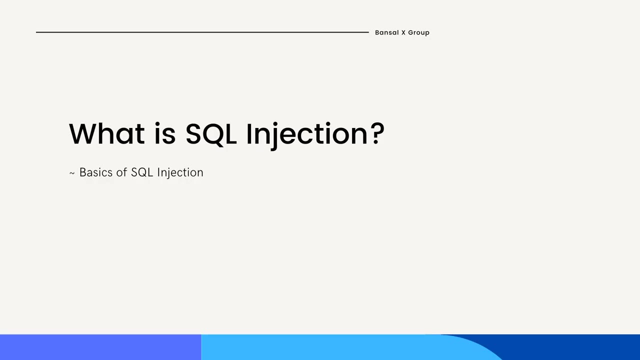 after completing this course or watching this video. Any numbers claimed within this video are, for reference purposes only, intellectual property of their respective owners, and the video contains professional penetration testing knowledge, and everything has been done in a controlled simulated environment. What are SQL Injections and why do they occur? 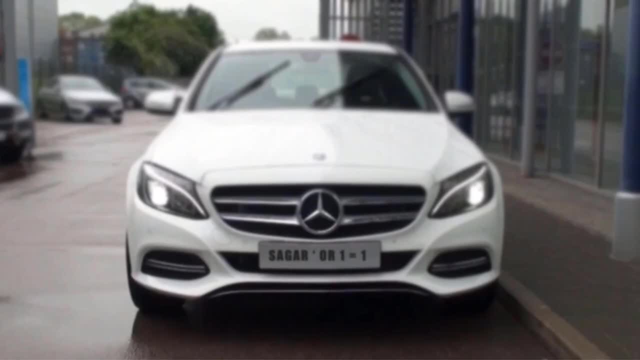 It's an interesting question because SQL Injection is one of the top 10 vulnerabilities as per OWASP, and it's been there for years and still we see it. Let me tell you a story before I get started. So this year in February, we bought this car on my birthday. 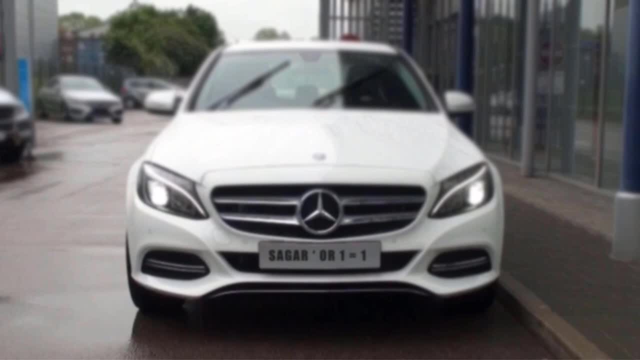 Now it's a Mercedes-Benz C-Class and there is no bench showroom in my city, So we had to take the delivery from another city. However, when we were taking it out of showroom, there was a checkpoint. On the checkpoint there was a camera which scans the number plate of the car. 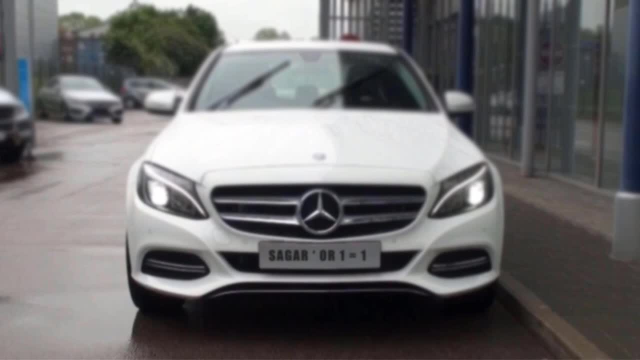 On the number plate. it scans that number and compares that number in the database and if the car is involved in some kind of fraud or if there is some ticket pending or if there is some criminal charges, It will knock it out. However, we just bought this car 5 minutes ago. 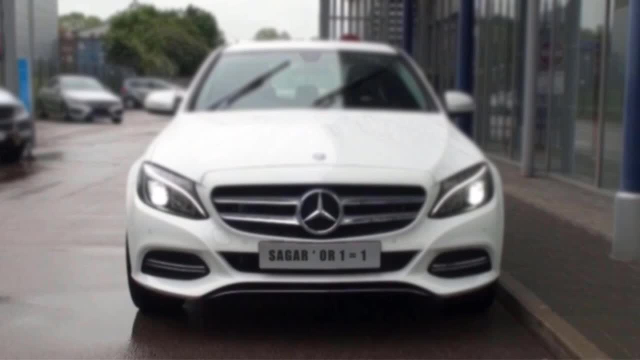 It doesn't even has a number plate. That was completely blank. Now here I have two options. I could even wait there for a whole day, get a number plate, maybe a temporary one, and then pass through that checkpoint. or what I did is I wrote this special characters which 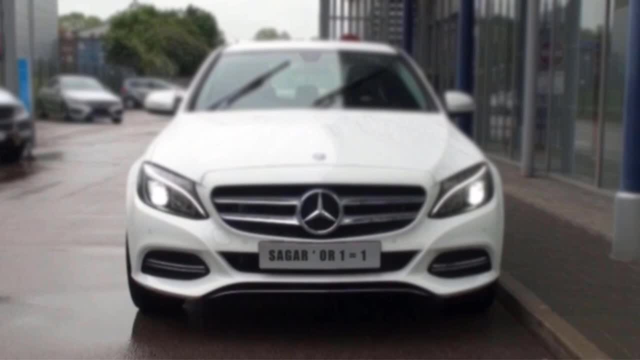 is SAGAR or 1 equals 1.. Now, this is a special query. When you put this in any database, It will always return true and the checkpoint compared this thing in the database and checkpoint said, yeah, allow this car. and it just opened and I took my car and that's how I passed. 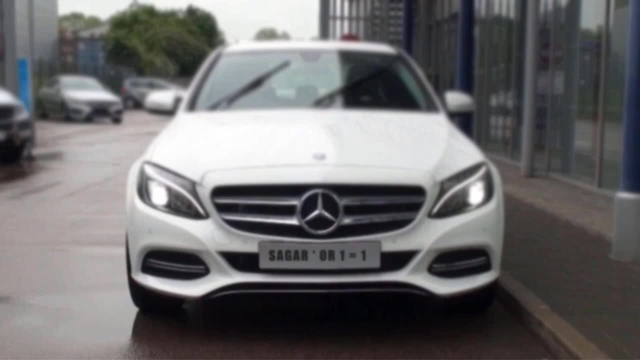 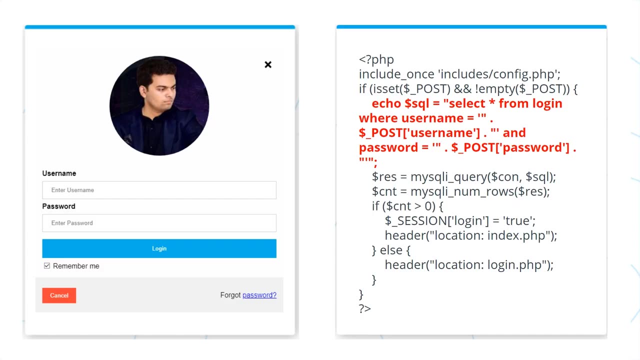 that checkpoint by putting in a skill injection. Now let me explain how this statement bypasses any checkpoint. You see, think about a login page. How does a login page looks like? There is a username, There is a password and there is a login button. 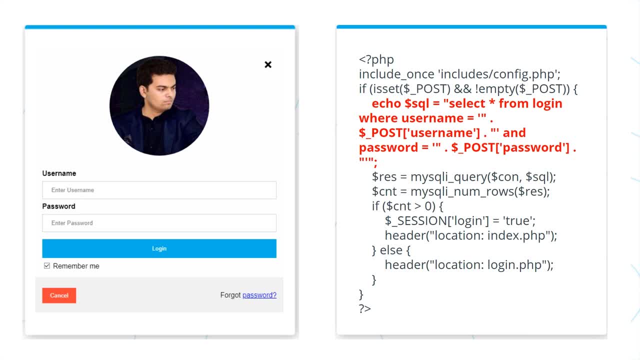 Right, That's the front end, That's the back end. Think about the back end. In the back end there is a lot of code, as you can see on your screen right now. You don't need to learn coding, but try to focus on that red part of the code. 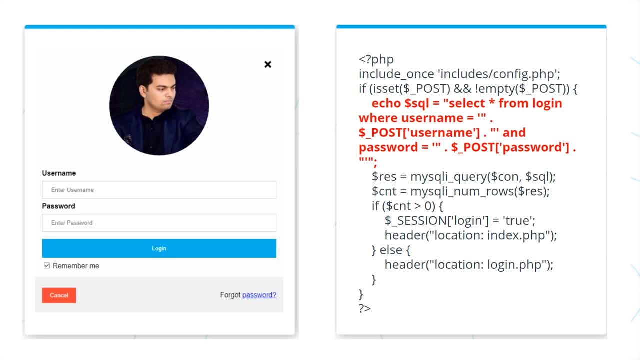 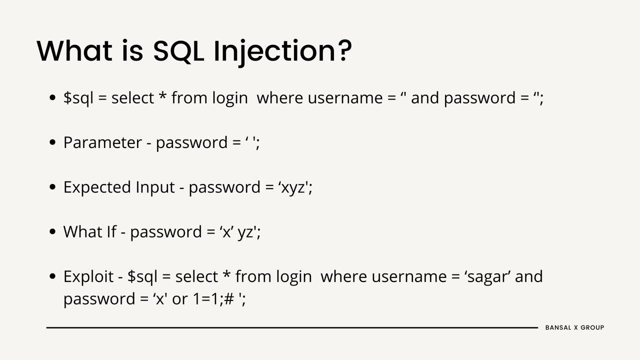 That is the code which is responsible to check if your password and username is true or not. Let me make it more easier, So this is the simplified version of the code. In this code it's asking select, start from login where username equals something: password. 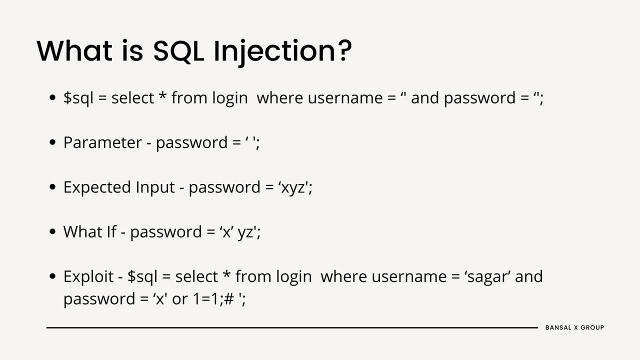 equals something. So there is the field username, There is the field password. In a login form you fill these fields and it goes to the database and it checks. hey, is there any user in the login table which has the username of Sagar and password as? 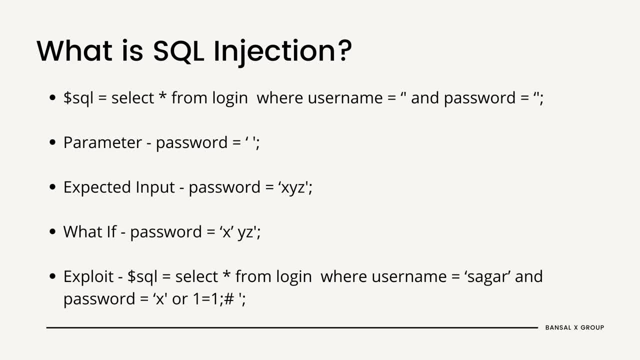 Bansal. If there is, it will return a result. If there is not, it will not return a result. So the parameter here we can choose any of these. let's say password: This is the expected input. password equals xyz, But a hacker like me will not give xyz. 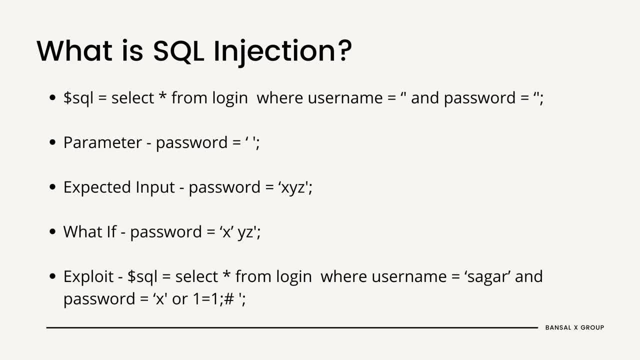 I will give x, single quote, yz. Now do you see what just happened here? That x was supposed to be closing with xyz and then that single quote. However, I just added a single quote and now I have two statements: password equals x, and then there is another statement which is yz, and single quote. 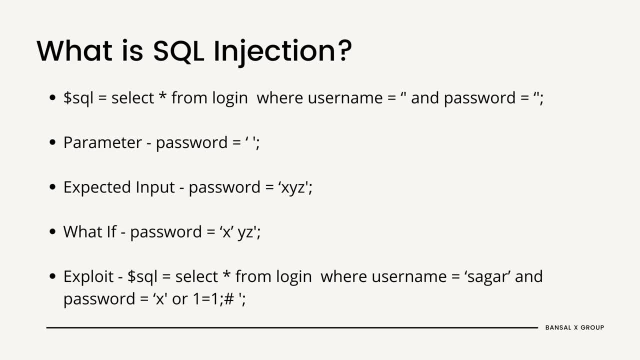 Now, once I am able to do that, I can write an exploit like select star from login, where username equals Sagar and password equals x or one equals one. So the system will check. okay, is there any user which is Sagar and is the password x? 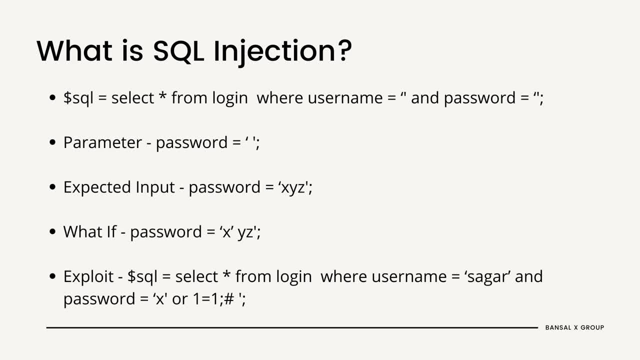 or just check if one is equal to one, which is always true. that is a tautology: one is always equal to one, which means that the result will be true and it will return a true statement and I will be able to log in. This is the reason. 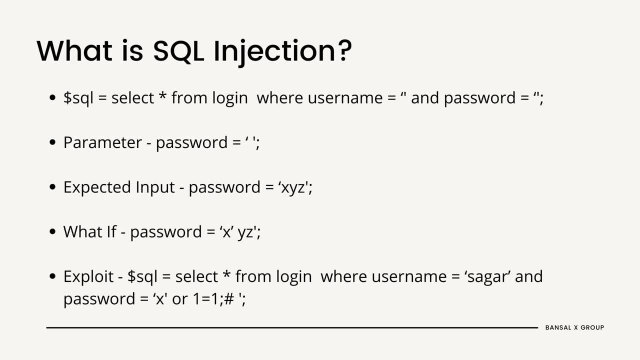 SQL injection occurs when you are able to control the database, put some data and manipulate it according to your wish. that's a skill. injection becomes so deadly. Of course, we'll be talking about how to make these queries, how to write this code, in later lectures, but this is the concept. that is how SQL injection works. 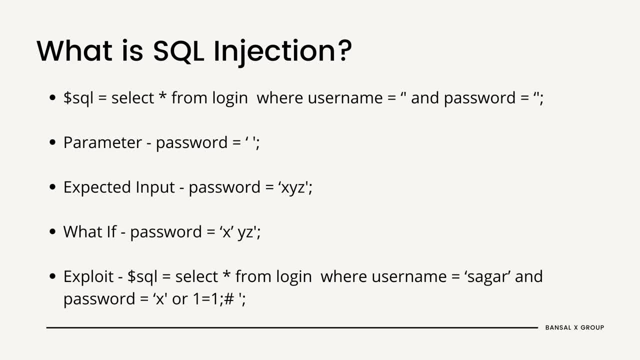 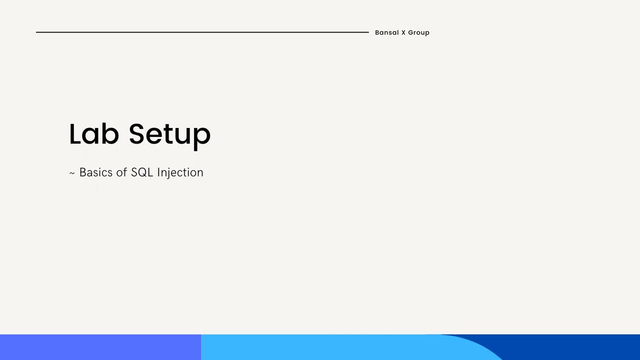 This is the reason of SQL injections to exist. when user is able to give certain data and control the database with that data, That is where an SQL injection comes into the picture. In this lecture, we will go ahead and configure our lab, which we'll be using for this course. 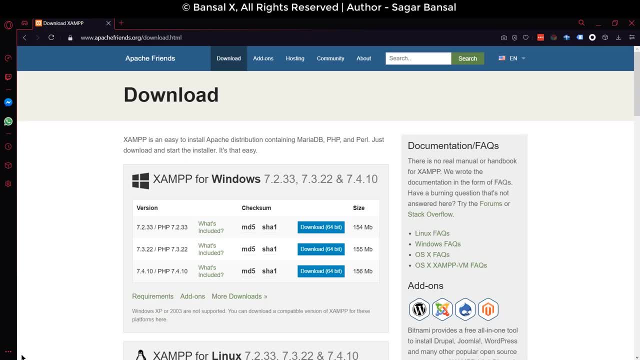 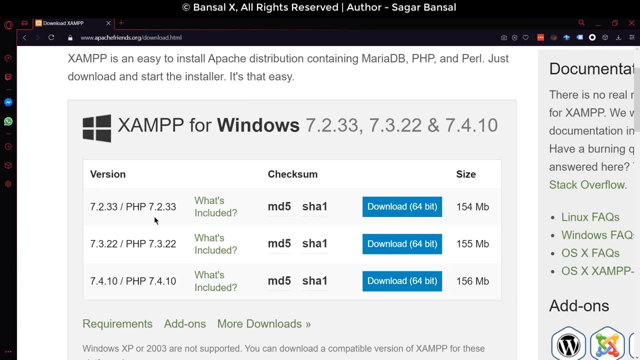 For that, I want you to download XAMPP for Windows. If you're using Linux, then download XAMPP for Linux, or if you're using OS X, then use XAMPP for OS X. The PHP version which I would recommend should be 7.2.33. just go ahead and download this. 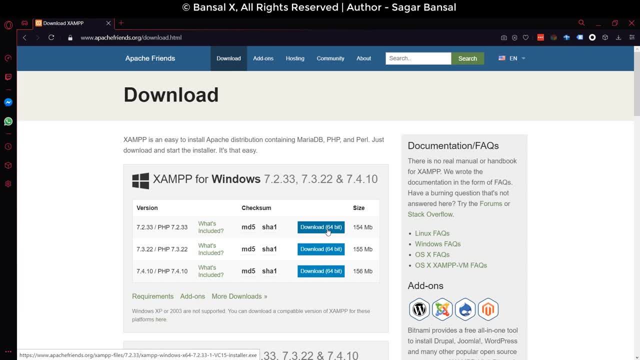 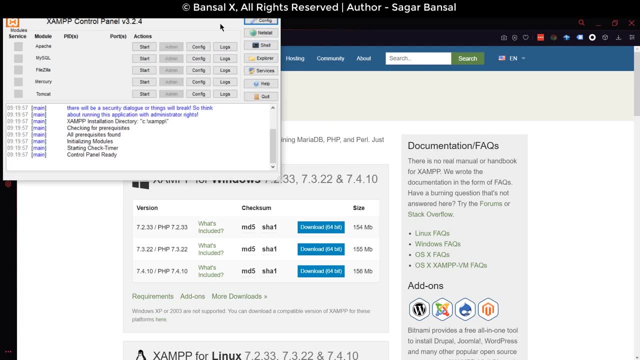 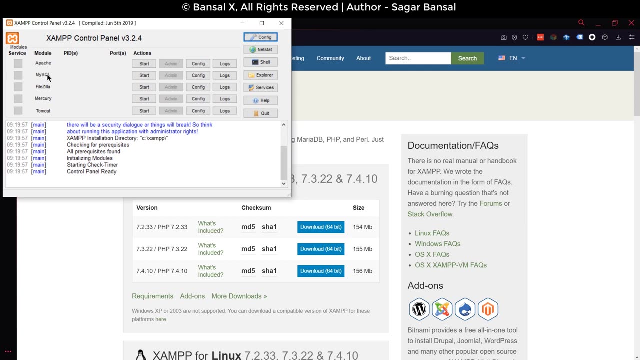 and install. It's a simple next, next, next install, so I'll not show that right now. Once you have installed this, just go ahead and search for XAMPP control panel. That is the software which you will use to control this. Now here you have Apache, which is your web server, and MySQL, which we'll be using as 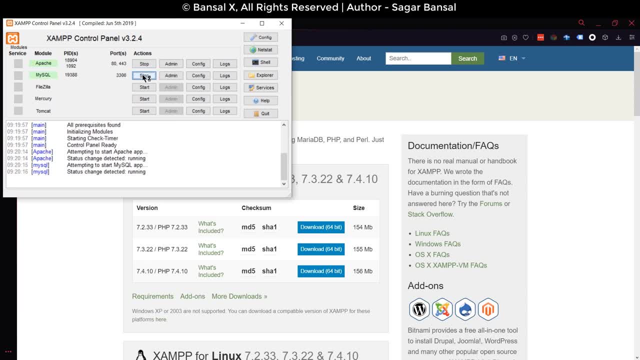 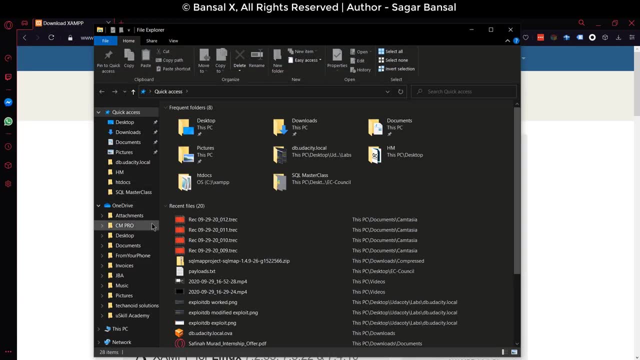 a database. So go ahead and start both of these processes. Once you're done with that, you can close this window. you don't need it And now go to your installation folder of XAMPP. In my case, that's installed in C drive. 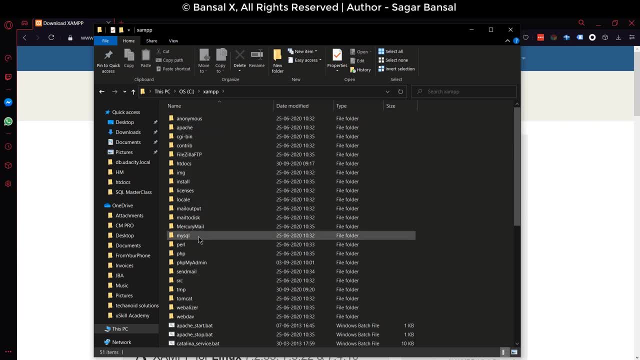 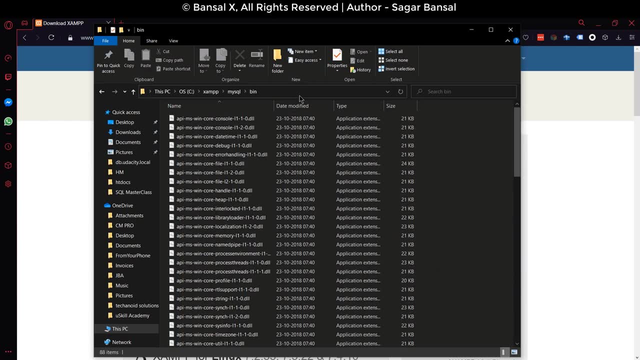 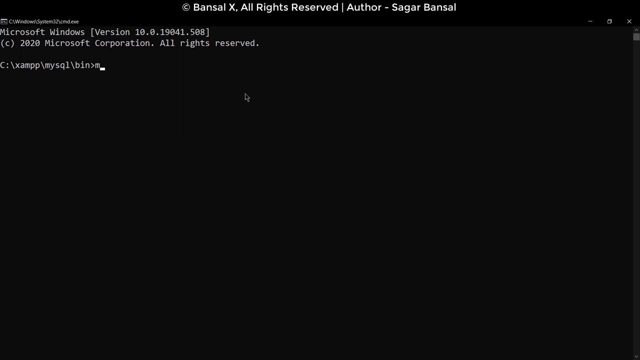 Here you'll find MySQL. In MySQL you have something called bin and here you have all the files for MySQL. Open the command prompt or a terminal window in this location and type MySQL dash U, space root. We want to log in as root and there is no password by default. 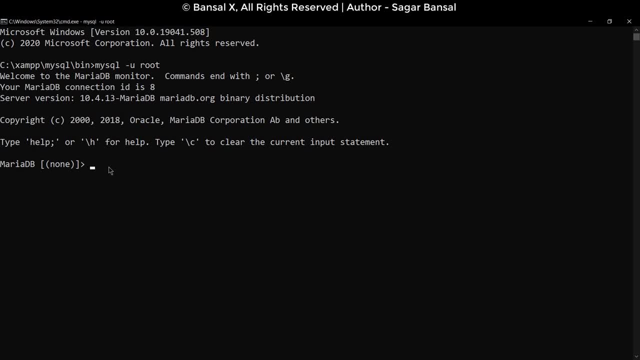 Once you do that, you'll be able to log into the database. Now here you have to create a database. So say, create database and give it a name. The name should be SPVA. Once you do that it should say: OK, query one row affected. 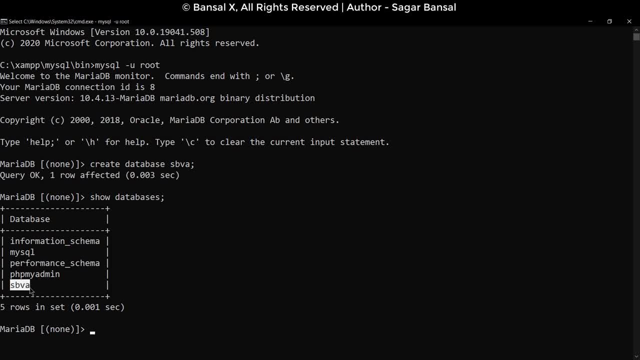 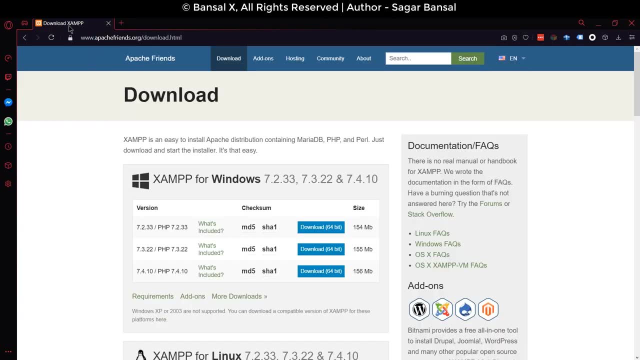 You can run show databases query to see if the database exists or not. Once this is done, you can close the terminal. and now you need the web application. You can download this web application from my site, From my website, Sagarbhansalcom. Here you can go to SPVA, which is Sagarbhansal's. 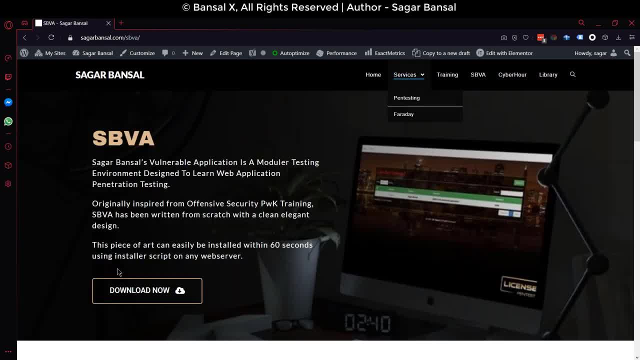 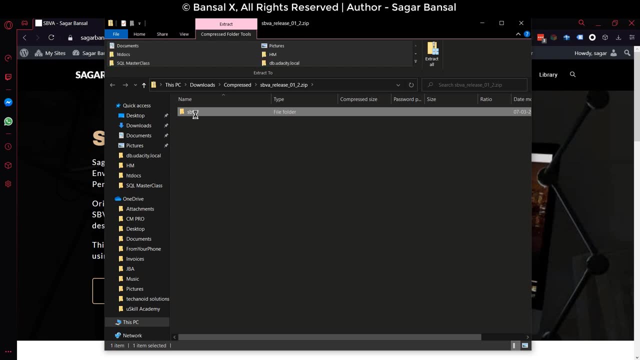 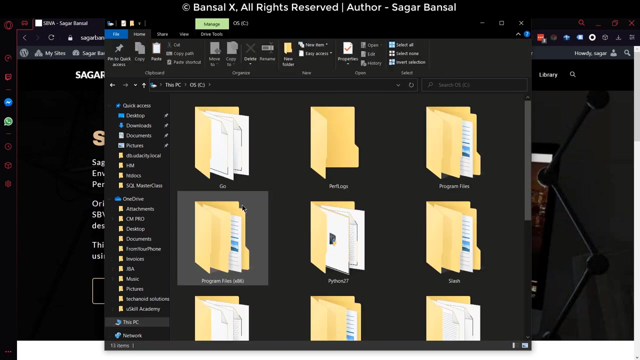 vulnerable application and you can click on download now to download this application. This is the SPVA folder. Let's open it. Copy everything Again. go to your XAMPP installation folder This time. find a folder called HTTdocs- This one. 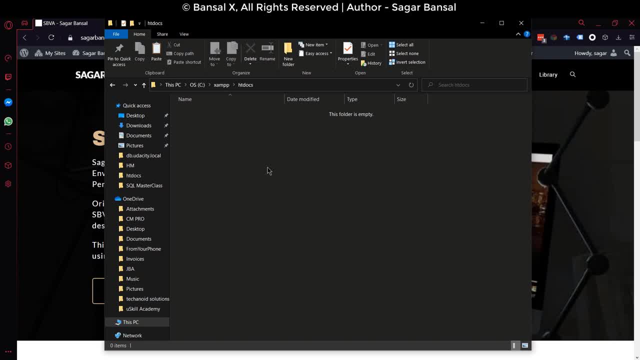 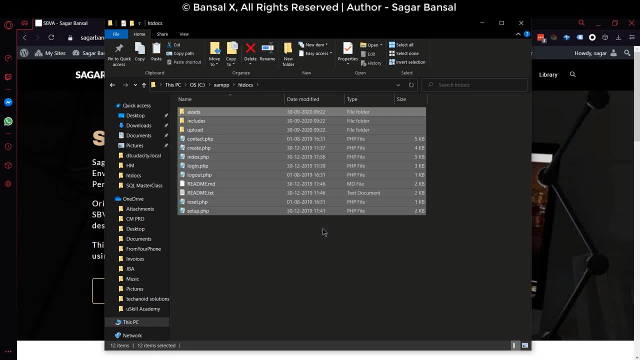 By default. if there are some files in this folder, delete everything. That's all good. If this folder is empty, just go ahead and paste this. It's the same thing: You delete it. make it empty and paste all the files which you downloaded from my website. 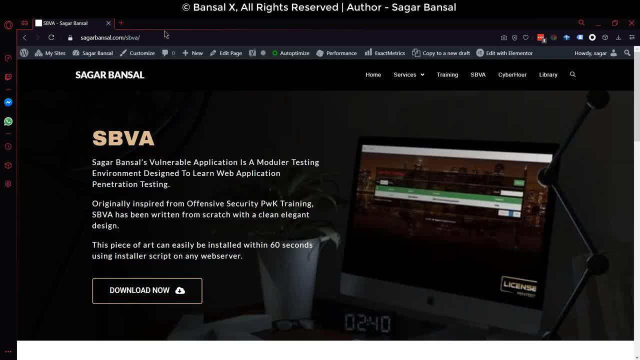 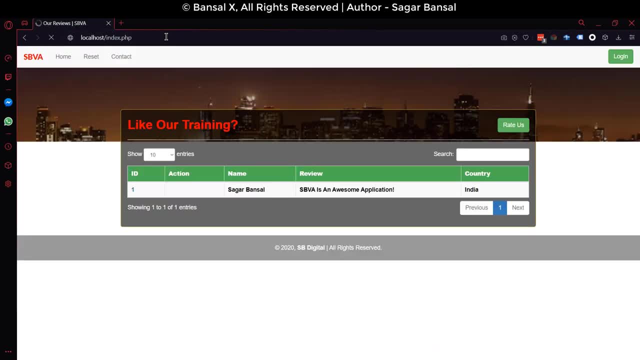 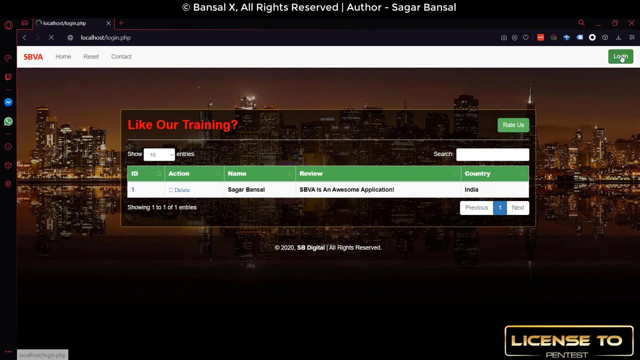 Now, once this is done, you just need to go ahead and open in your browser Localhost slash setupphp. Once you do that, the application will be ready to install. You don't have to do any other configuration. You can go ahead, click on this login page and try to exploit this login page. 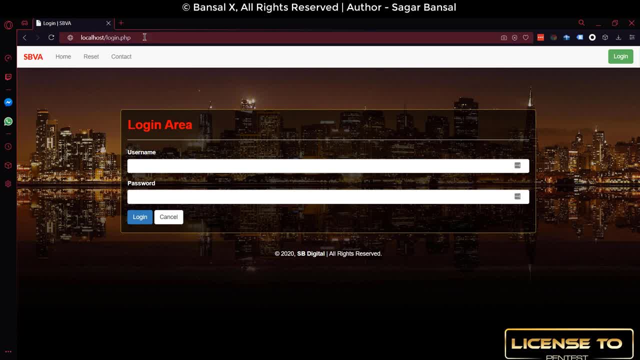 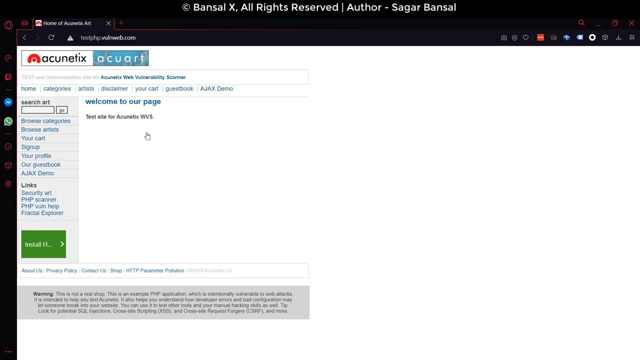 That is how you set up this environment. However, in this course, I will also be using an online application called TestPHP. Once you search TestPHP on Googlecom, It will say home of Acunetix R. This website is owned by Acunetix company and it's a testing. 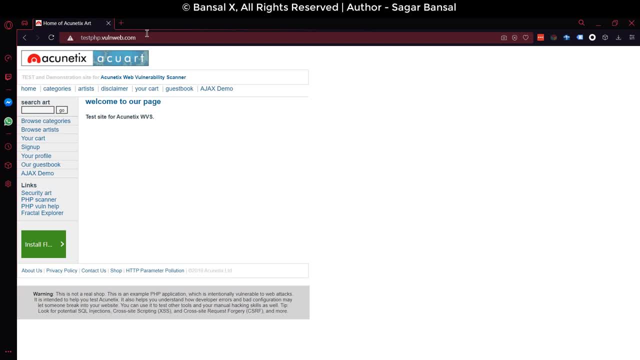 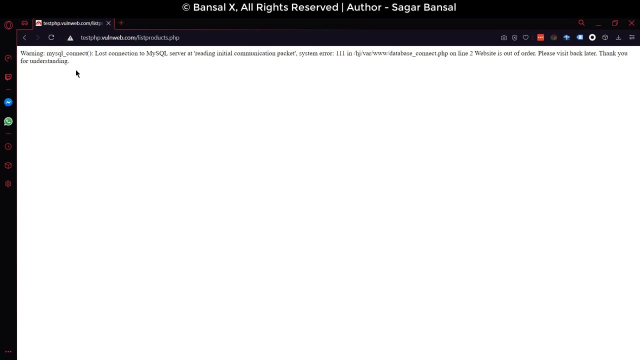 website. As you can see, testphpworldwebcom. On this website there is browse categories, In that there is paintings. This sometimes gives you an error because someone else in some other country is trying to hack this website, as this is made for hacking. 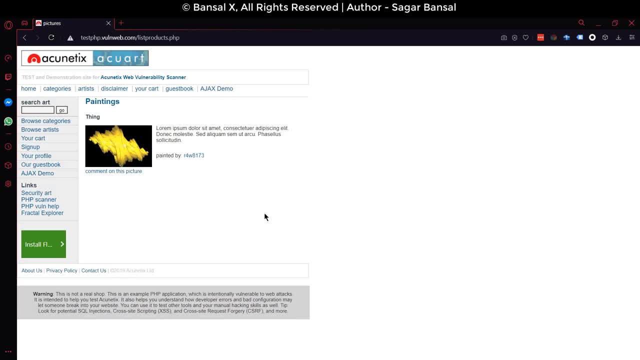 That's all good. Just refresh the website. It will load eventually, And this is the page which we will be exploiting in the course. So this page and SBVA application, Both of the things that makes up our lab, The basics of MySQL. 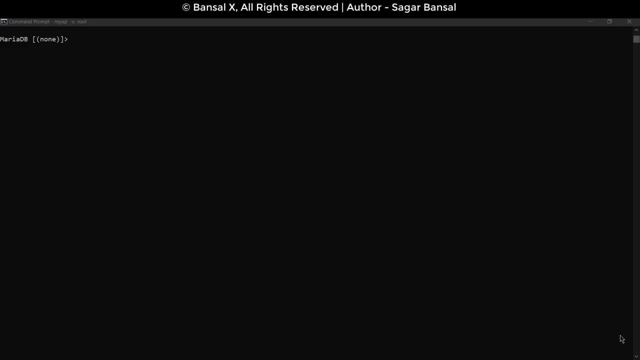 It's really important for you to understand the basics of writing SQL queries. Of course, I will not be teaching you all the SQL language in one shot And of course it's not an advanced SQL class, But you need to know very basic language. 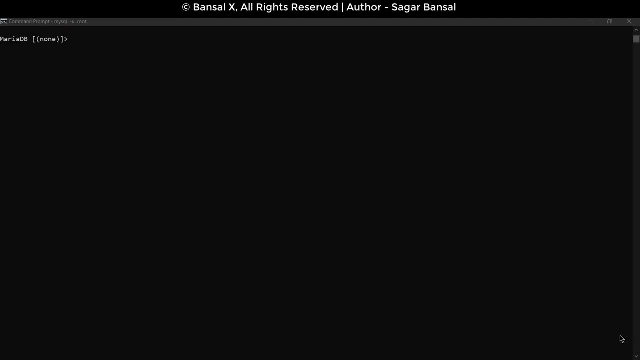 So let's get started. You need to know the language so that you can use them to understand the SQL injection queries. For that I need you to login to your MySQL console Now. the first command is show databases, Which will give you all the databases that you have. 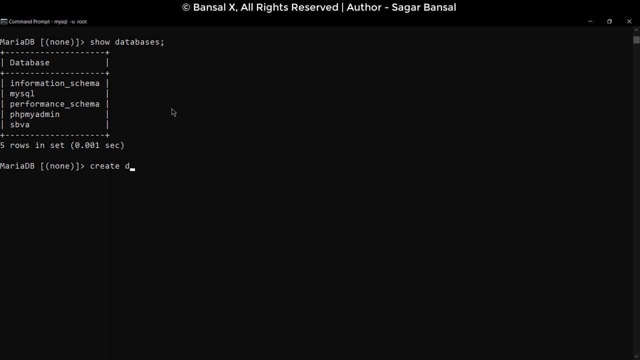 Next command is create databases And you can create any database. In this case I'm creating a database called x And you see it's x And you see query one row affected. If you run the show database again, you will see you got a new database. 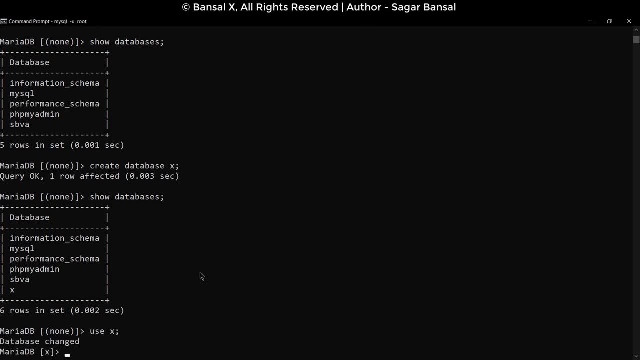 Next command is to select the database. So you say use and the database name, which is use x. Now we are in the x which is determined by this column here. Now let's see if there is any table in this. Show tables for that. 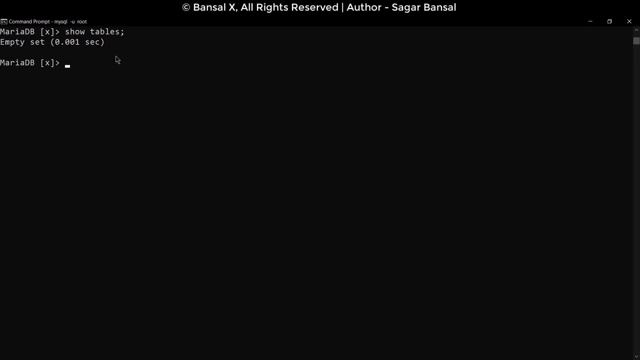 However, it's an empty set Because there is no table. Let's create and table them. So I'm going to create a table called users. Now, the reason I have these braces here is because I will be putting what kind of data will be stored in this users. 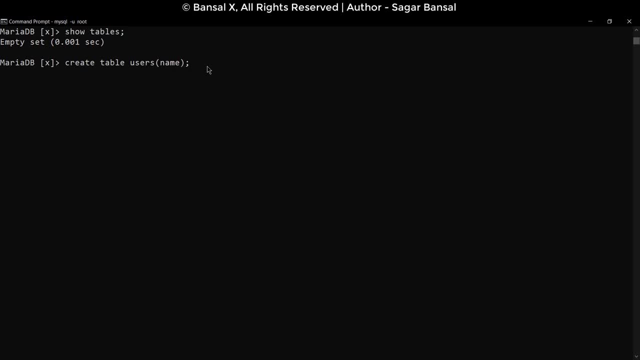 The data will be, first of all, name. Now the name is the name of the column. Okay, The name of the column where the data will be stored, But what type of data? There are certain types in SQL And it depends on the product that you're using. 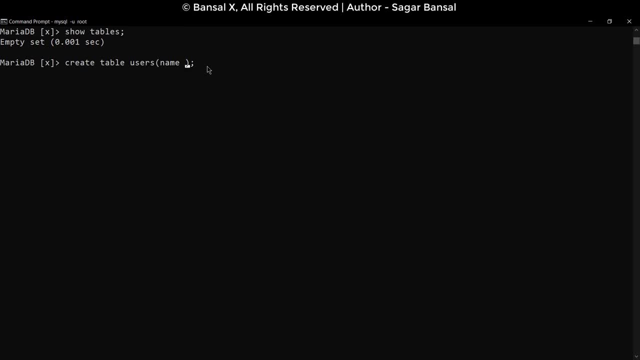 In my case, I'm using MariaDB implementation of SQL, So the type which I have to use is varchar, And in varchar I have to tell it how many characters the name can be. Let's go 100 characters, So someone can type a name which will be stored in the name, which will be of varchar type, which 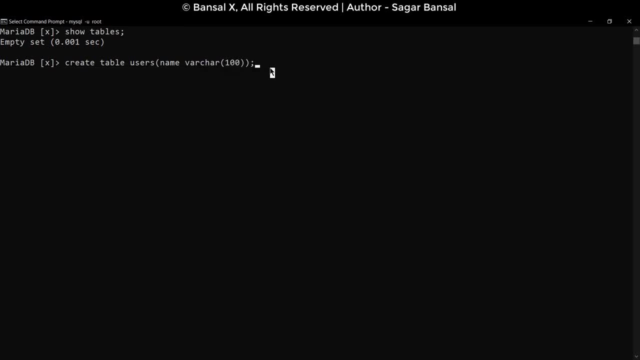 is characters And that will be 100 characters. Let's press enter and you see query. okay, zero rows affected. Let me show you the tables. now You can see we got a table called users. If I select everything from users by using the select query, where star means everything, 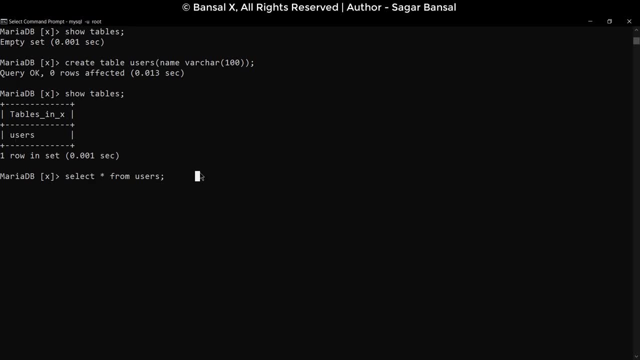 So select everything that's there in the user. Show me everything that's there in the users. You will see it says empty set. However, I can go ahead and add something here by putting insert into values, So I can use insert into table name, which is users. 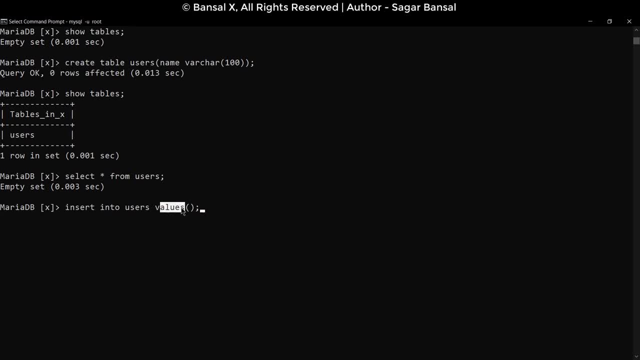 I can insert into this users table values and I need to give the values. Since I only have one column, which is name, I'll give the values here. If I'm using name, I have to use double quotes and I can give a name like Sagar. 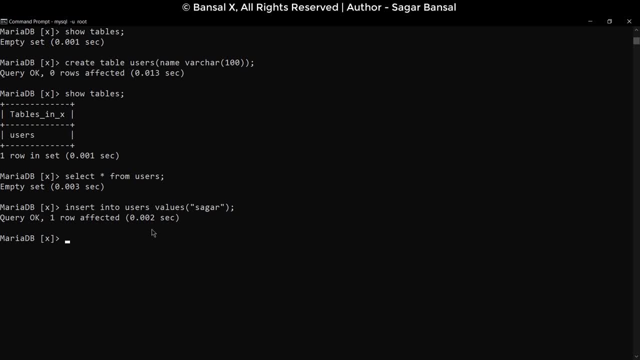 I can press enter and you see one row affected. If I do select star, you will see there is a column name and there is a value which is in Sagar. Similarly, I can add more users by using the same query and saying second user as Alice. 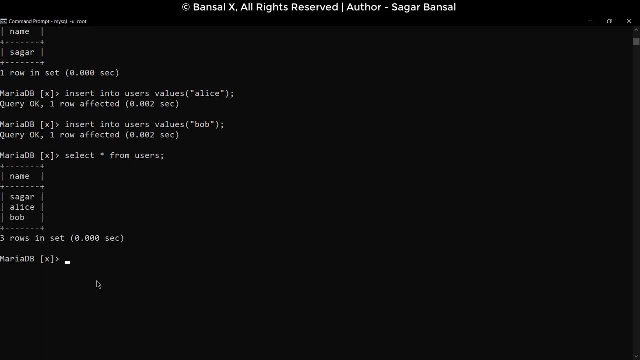 and third user. as Bob, And if we try to see the users and you can see there are three records which are these, which are in the column of name, which are in the table of users, which are in the database called X, I can delete some stuff, let's say the whole database, by saying drop database X. you. 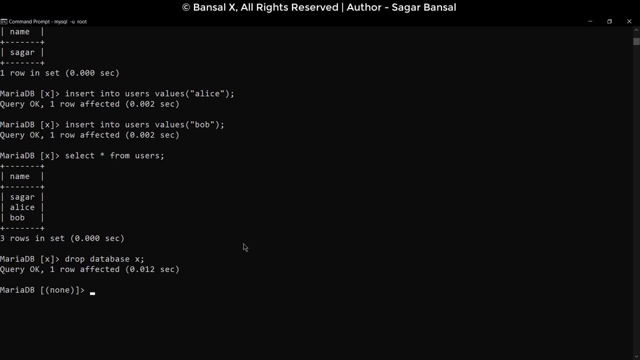 can do the same for tables as well. drop table and the table name. as soon as I do drop database X, you can see it is none here and there is no database now. so if I just show you the databases, you can see we don't have X anymore. that's how. 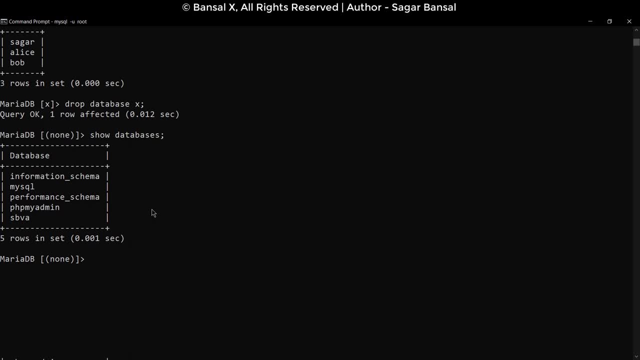 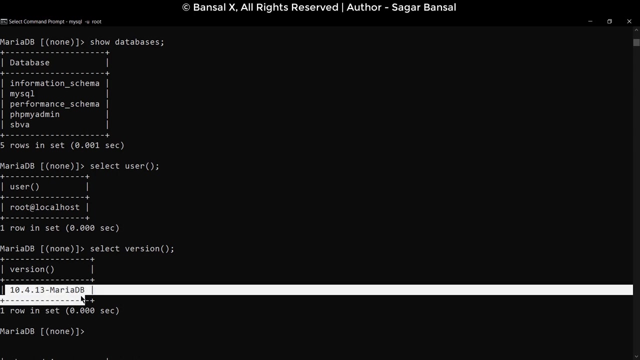 you delete the database. now there are three functions that I want to explain. the function of user, so I can say select user. you can see it gives us the output of user running on the server. so we are running this as root. there is another function called version, which is going to give us the version number of the 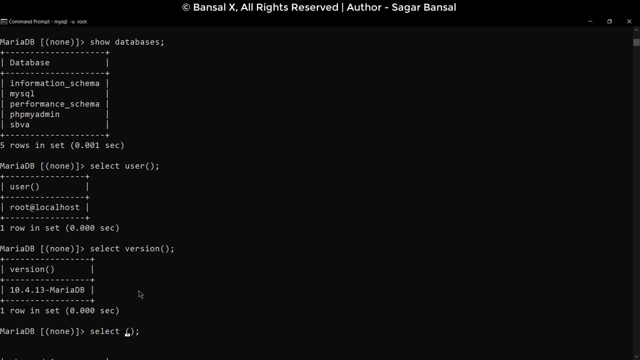 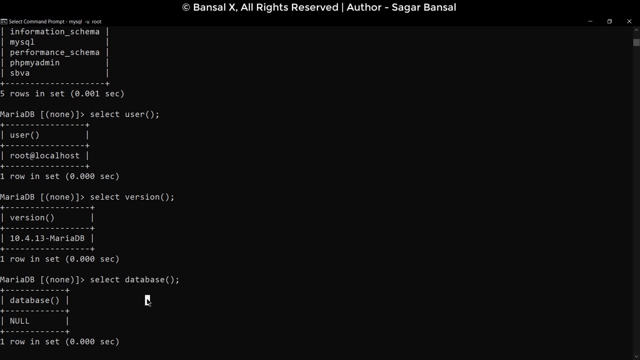 database and there is another function called database, which will throw us null because we are not using any database. however, if an application is using a database like use SPV a. now my application is using SPV database. if I do select database, you will see that it gives the database as. 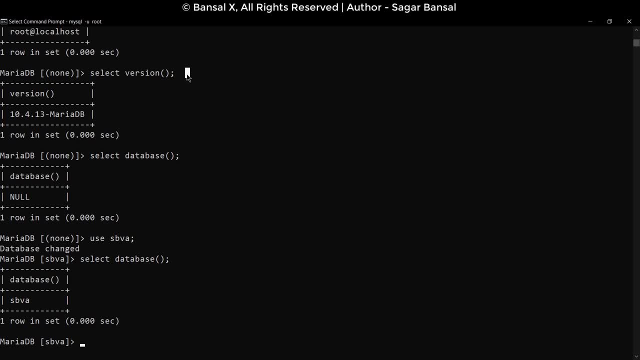 the result. so these three functions can be really helpful while gathering data in SQL injections. this is the core basic that you need to understand. there are many things like or and where, order by group by, but this is not an SQL class, though. I will be explaining all of these things in the course whenever I can, but you can always. 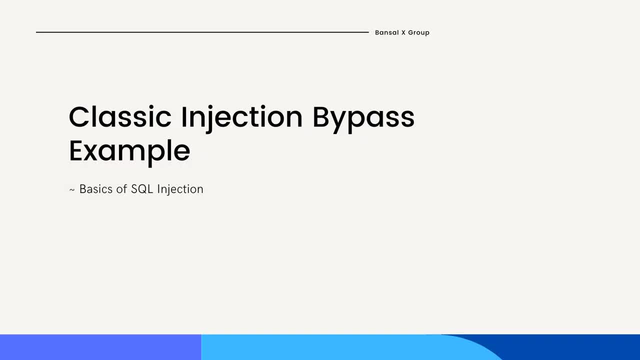 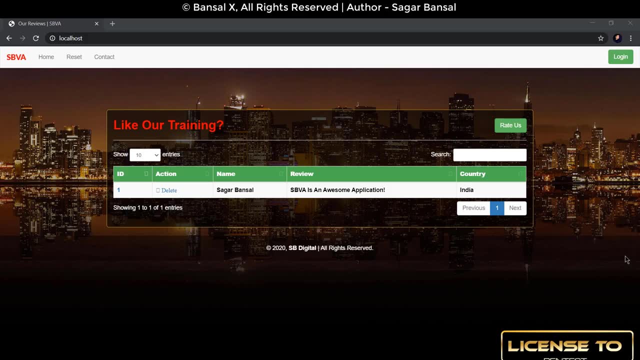 use Google as your friend. the classic injection bypass. well, a classic injection bypass can occur at any place. for this example, I will be using an application that I developed. it's called SPV, a Sagar Bansal's one rebel application. so you can go to this login. 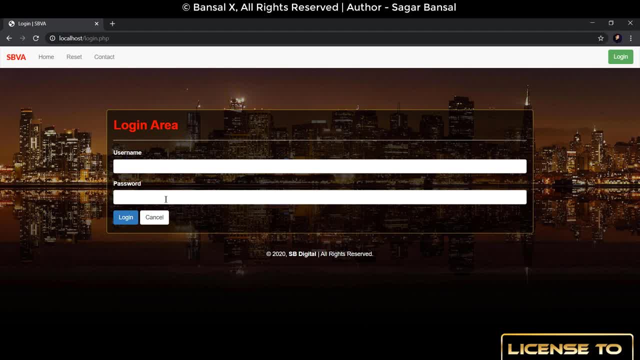 page and this is the place where I'll show you how to do a classic injection bypass, because this is the easiest to understand. now, it's a simple login page. if I do anything like admin, admin, which is a wrong username and password, it will not throw any error and not even say that the username is wrong or the. 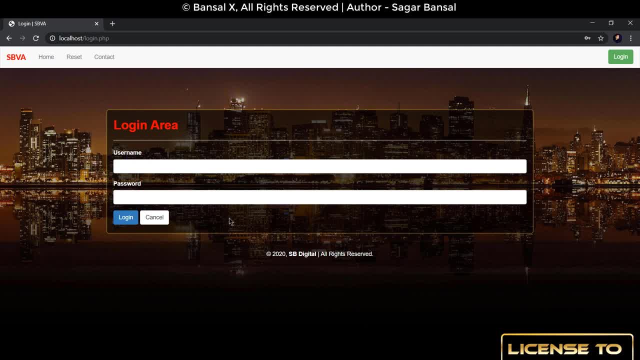 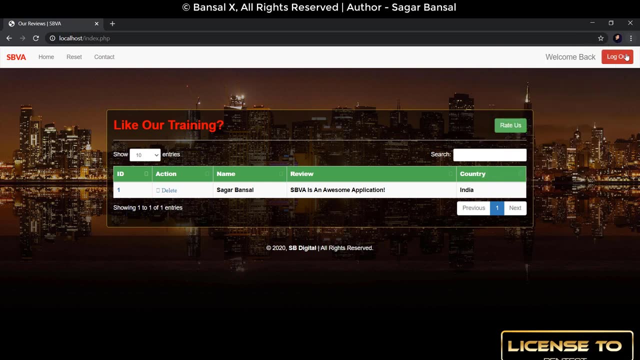 password is wrong. it's completely disabled with the errors. however, if I use a correct username, which is Sagar, and if I use a correct password, which is Bansal, it will go ahead and log me in and you can see, now I can log out, and this is the place where I'll try to do a classic. 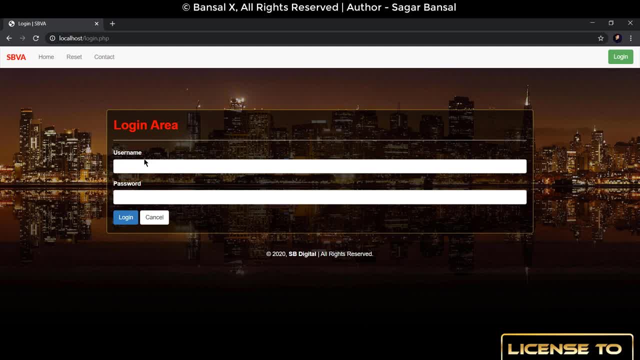 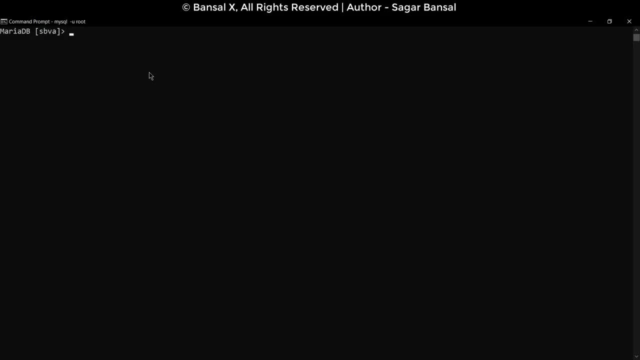 injection bypass. first of all, we need to understand how the code of this application is working. to make it easy for you, let me show you the command line and I'm going to show you the tables here. there are two tables. we will use login table. I can see in the login table there are just three. 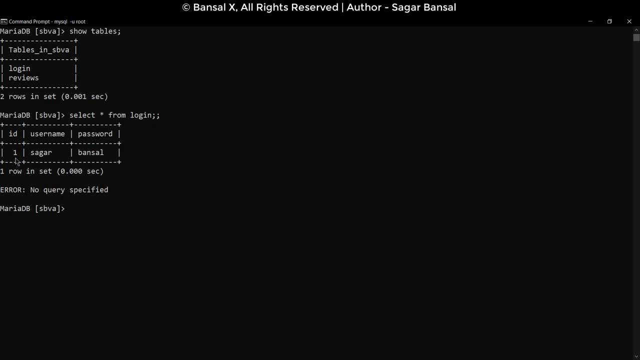 entries: ID, username, password. ID is one. username is Sagar, password is Bansal. now, what do you think the backend of that website is using as PHP? the query might be select. start from login. your username equals Sagar and password equals Bansal. let me show you how. 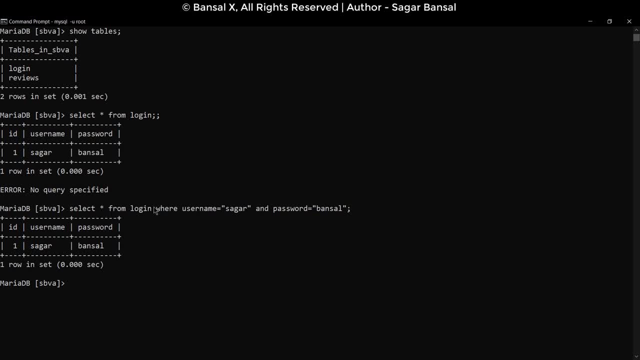 so this might be the query that the website is using: select start from login. their username equals Sagar. now you will see that the website is using the password Sagar. now you can see that the website is using the password. and you can see that the website is using the password. 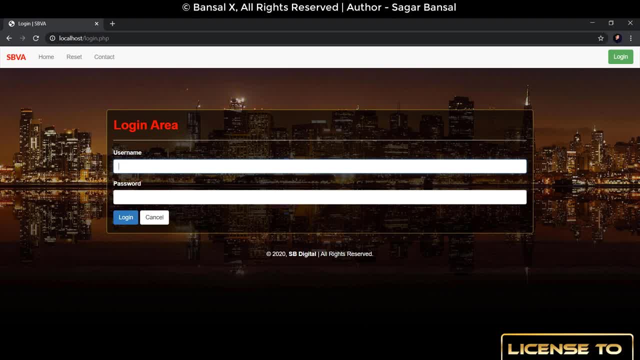 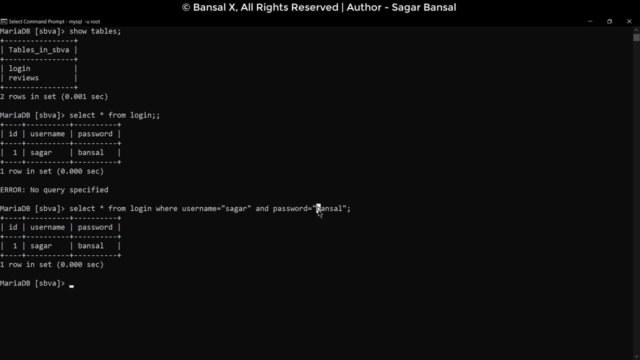 the question is: how can you control this Sagar? by putting it in the website over here in user name field, and you also control this Bansal by putting it again in this field, which is password field. the ability to be able to control these fields, which are being directly used as an input in an SQL query, is very dangerous, and that is where you can do a classic injection bypass. 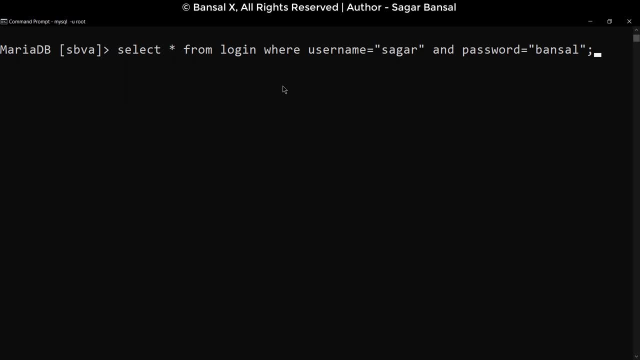 Let's look at it carefully. Since I am the one who controls what I will put in the sagar, can I not go ahead and put sag in a double-chords space Now? do you see what just happened? I just created sag as the variable and I have got the ability to write some code here, and 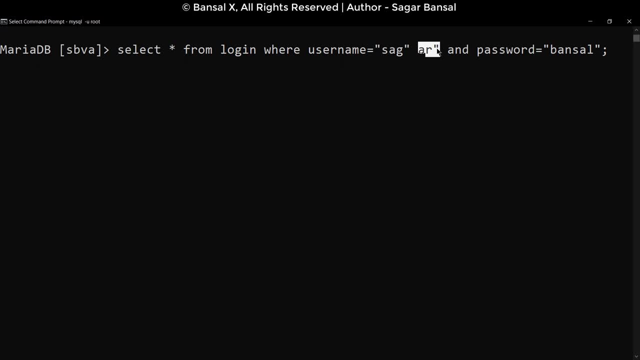 this all is an additional thing. It was not supposed to exist. This was never supposed to exist. It was supposed to be, and here, Well, I just break this double-chords by putting a double-chords, and that's where the classing injection bypass works. 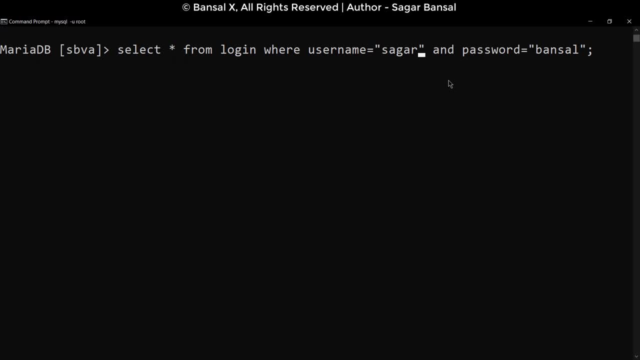 So, instead of this thing, I may put sagar and a double-chords to break and then or one equals one, which is basically that check if username is sagar, or one equals one. That is a classic injection bypass. However, there is a small problem in this. 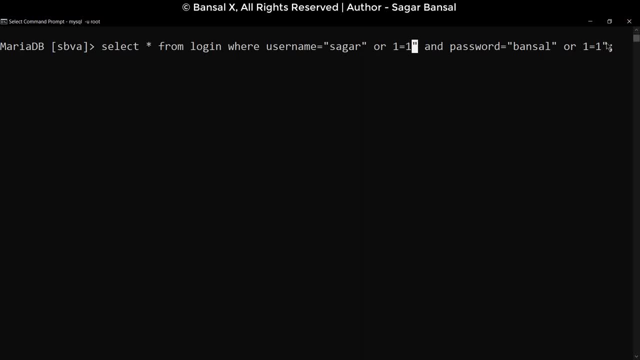 This code is never supposed to be here and this code is never supposed to be here. In such a case, we may go ahead and utilize this code by putting one code here, one here and one here, and similarly, we may use it by putting it one here, one here and one here. 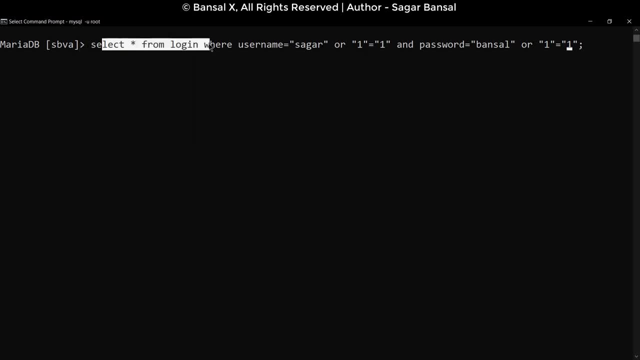 Now This is a perfect SQL statement: Select star from login where username equals sagar or one equals one and password equals bunsell or one equals one. So basically, I can go ahead and press enter and this will work. However, even if I give it a wrong username and password, like admin, this time this will 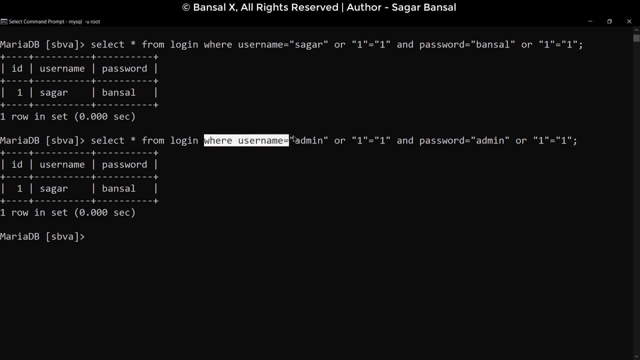 still work Because the statement of where clone This will still work Because it is being nullified by the statement of or clause. in both of the cases, This password and this username doesn't matter until one is equal to one, and this will always. 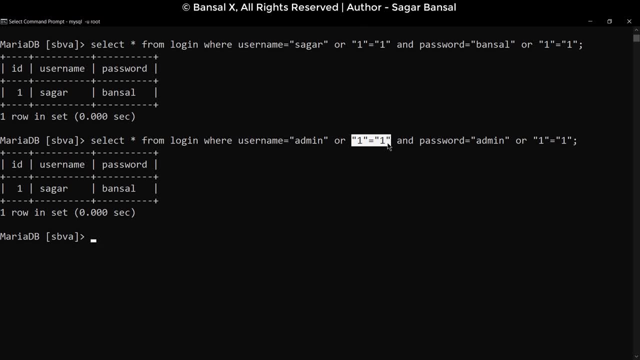 be equal to one, because this is a tautology. So that is how you do an SQL injection bypass. There are many other ways to do that. Maybe you cannot put these double-chords in certain situations, Then how do you do that? 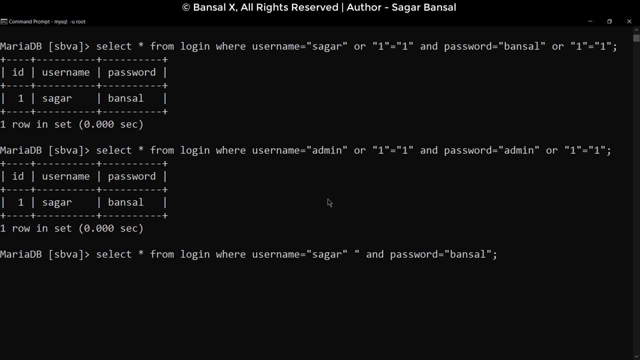 So, for an example, If you are breaking it from here And you are typing or one equals one, Then you may want to go ahead and remove the whole part from here by commenting it out. Comments in SQL depends on the product. In MySQL you can use a hash sign. 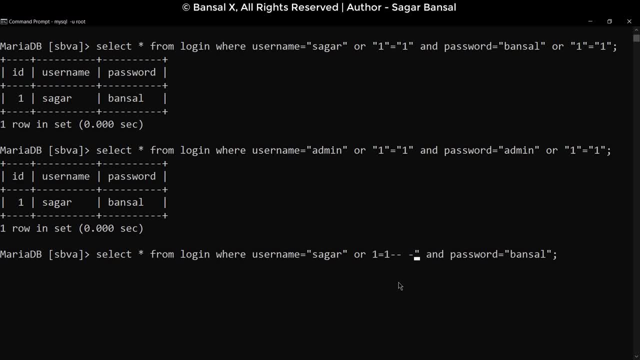 Or a minus minus sign, Or minus minus space minus sign Or a slash asterisk sign. There are many ways to comments And some will work, Some will not work, So you have to try all of them. Let's try with hash. 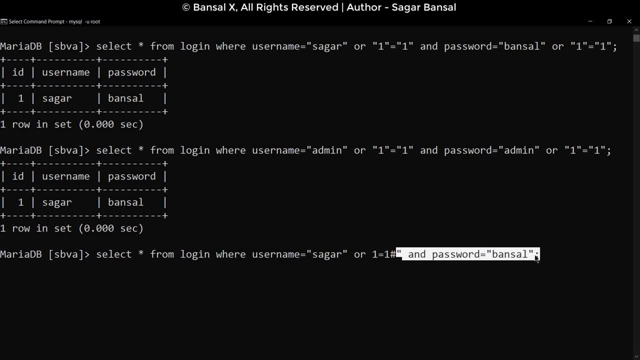 As soon as I press hash, all of the preceding code will be marked as a comment. So my query is: select star from login where username equals sagar or one equals one. That's it. Everything else is being ignored. Now let me try to press enter and let's see if this works. 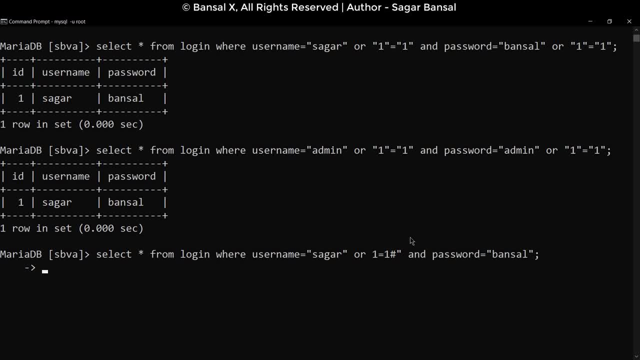 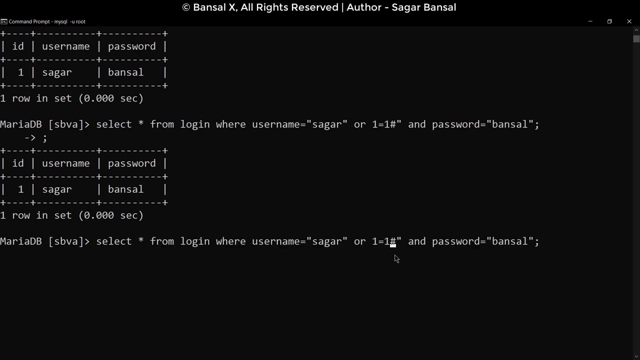 And here you go. It's asking you for a semicolon Because This semicolon is getting ignored. So there should be a semicolon before this comment sign. I'm going to press this. It will work. However, a good query will be putting a semicolon over here before this SQL sign. 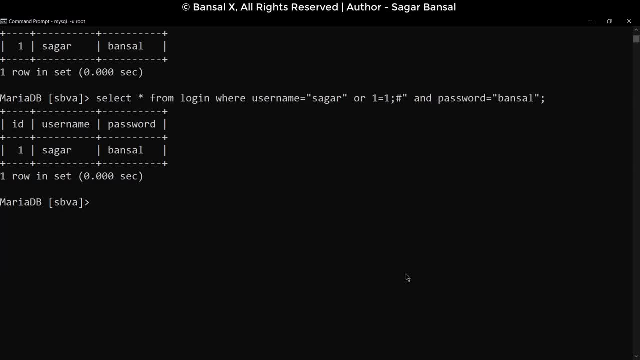 And now you see it works perfectly. So I can go ahead and try another type of comment like minus minus. That works as well. I may try minus minus, Minus space minus. In certain cases minus minus doesn't work, So minus, minus, space minus may work. 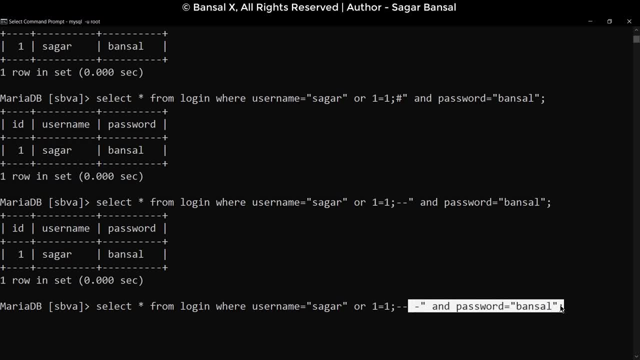 However, here you may say that you know what this is just getting commented out, So it doesn't matter. Whatever I press here- and you know I can even write this thing- It will all get commented out. However, as I said, in certain cases minus, minus doesn't work. 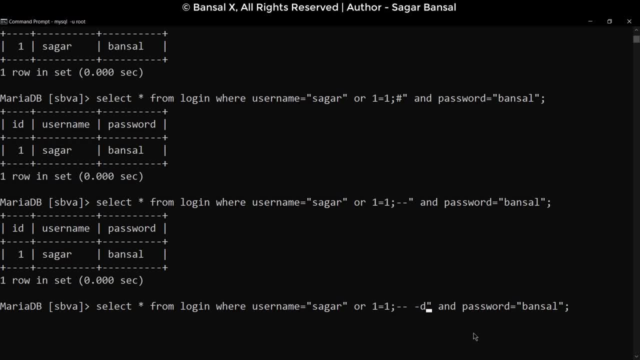 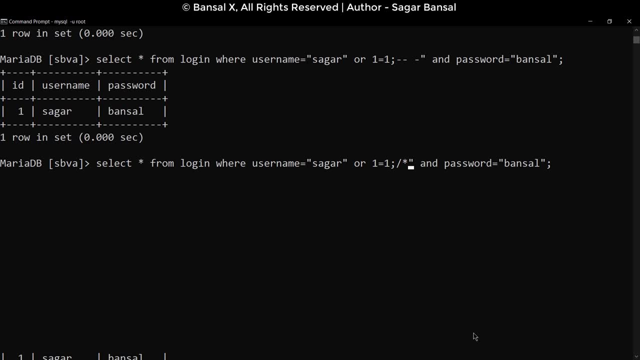 Minus, minus space, minus works, So you may want to keep that in mind. It works. I may want to try with a, with a slash asterisk. This also works. And here you can see: suddenly something has changed in my database and it doesn't look. 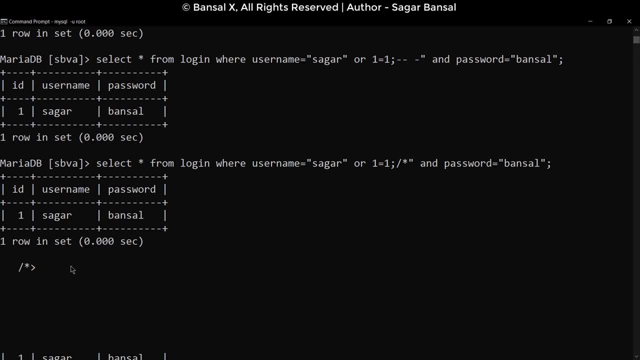 correct. So it is asking me for a star slash, you know, to close the comment. It's a multi-line comment. You can comment multiple lines by writing slash, asterisk And then asterisk, slash, To close the comment And it'll keep asking me for it until I close it. 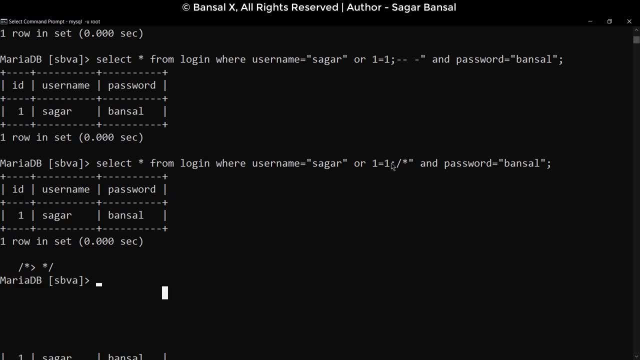 Now I am back in my database console, So we will not close it, because if we close it, then this statement will not get commented out. Hence, in certain cases we just keep it open and system automatically ignores this part. sometimes This one is risky, but works. 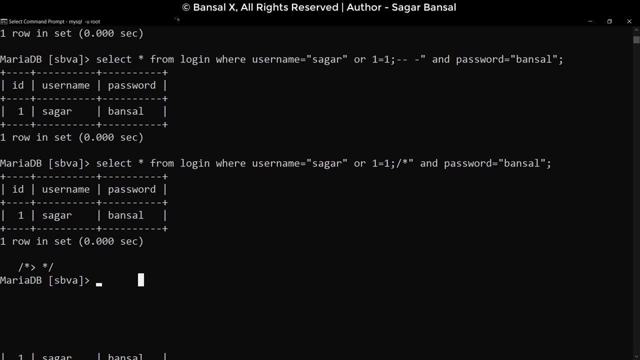 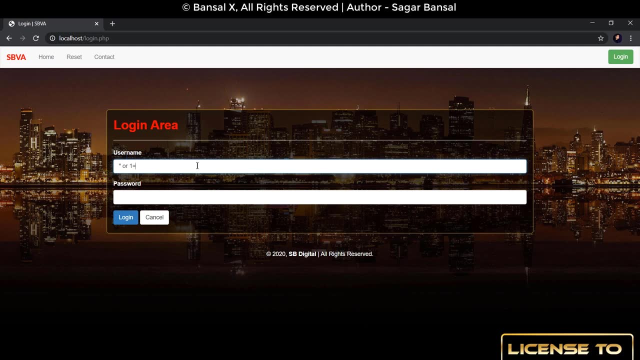 Now that you know how it's working, let's go ahead and try to bypass the website itself. So I will put in a username, A double quotes or one equals one, and then a hash sign. I will copy the same thing and put it in password, though it doesn't matter. 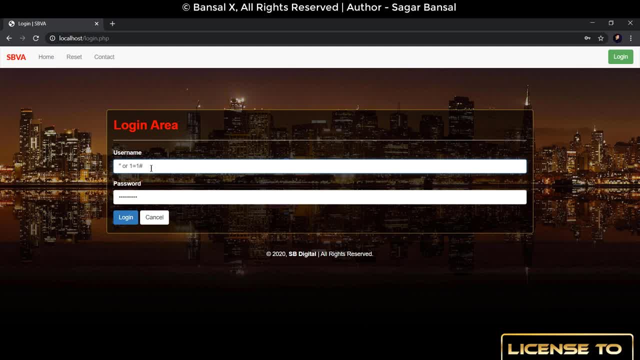 So we're just commenting out the rest of the thing. Oh, we just forgot a semicolon here. Now let's try to log in. Well, that didn't work. What just happened? Let me tell you one thing: In certain cases, 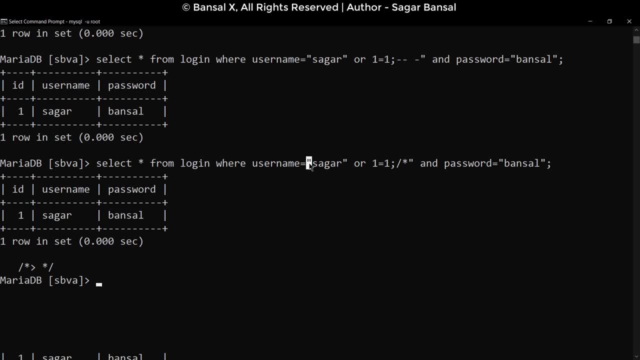 This. double quotes can be Completely replaced by single quotes. It completely depends on what the developer has decided to use. So in this case, The website is not using a double quote. The website is using a single quote, which is a common practice. 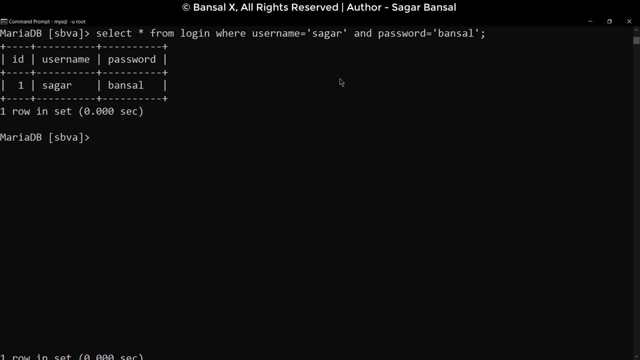 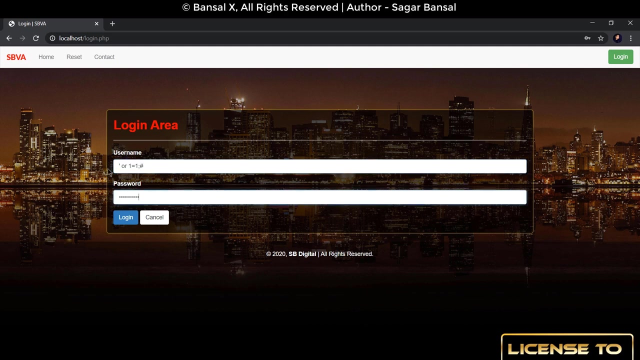 So the website is using the single quotes instead of double Hence, to break out from it, I need to put a single quote here, not a double quote, and then I can press or one equals one. So in the website I will put a single quote here, not a double. 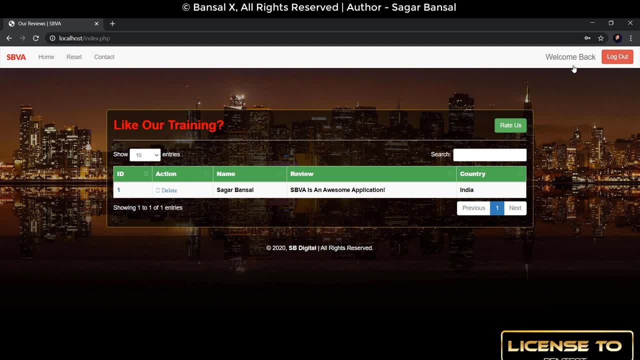 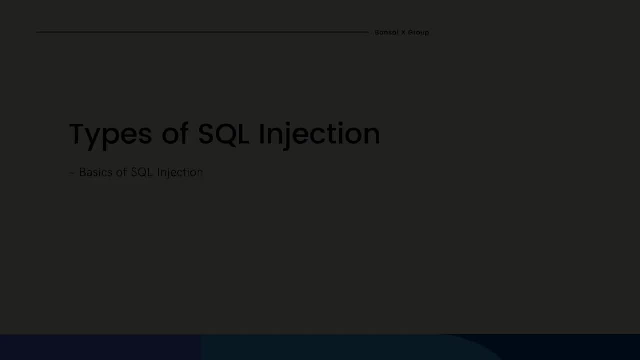 And now I can press log in and you can see I was able to log in without putting any password. That is how a classic injection by passwords, types of SQL injection. There are multiple types of SQL injections which you should be aware of because, depending 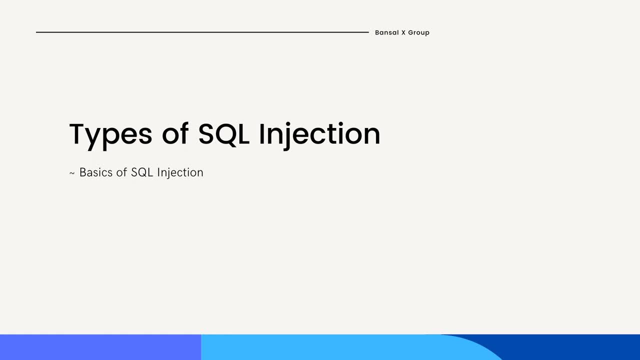 upon the target and the situation, you may have to switch between one type and another. There are two major categories of SQL injection. There are two major categories of SQL injection. There are two major categories of SQL injections. There are two major categories of SQL injection. 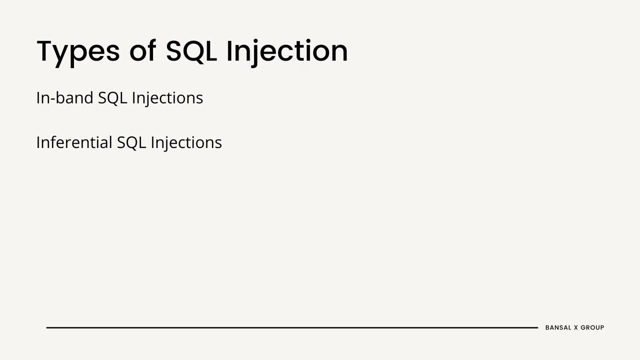 There are two major categories of SQL injection. First one is inbound SQL injection and second is inferential SQL injection. Inbound SQL injection occurs when you are able to get the response from the website. It can be some data or it can be some error. 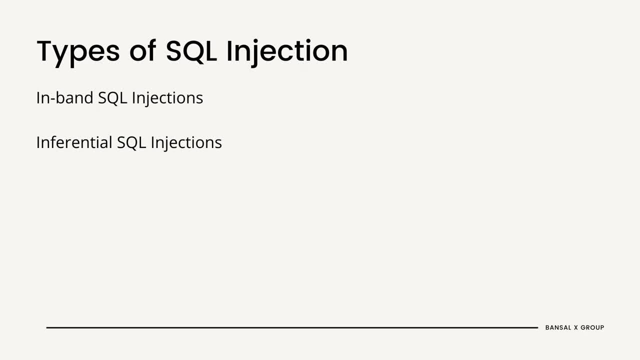 So think about a database, A database containing a lot of paintings. You are able to get those paintings depending upon your searches. So you are searching for a painting which has an id of 1., Which has an id of 2., which has an ID of 3, or you're searching that on the basis of price- any painting. 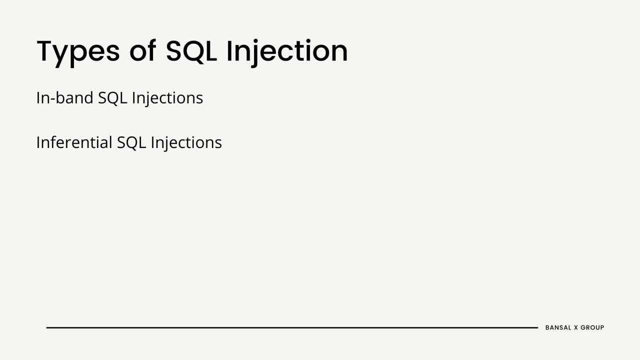 which is costing less than five thousand dollars, any painting which is worth more than twenty thousand dollars. depending upon all this, you'll be getting some data from the database. those are data based SQL injections. there you can use a technique called Union based SQL injection technique, where you will use 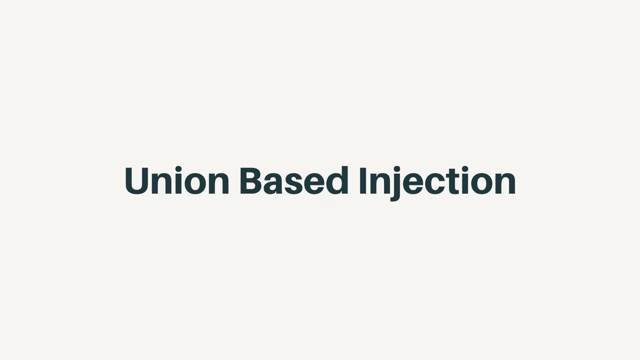 the Union command of SQL. I know it's being a little confusing, don't worry. I'll be explaining what is Union and how to do that in a whole separate lecture. but just understand: when you are able to get data from the application, you will most probably go with the Union based technique. the second one is error based. 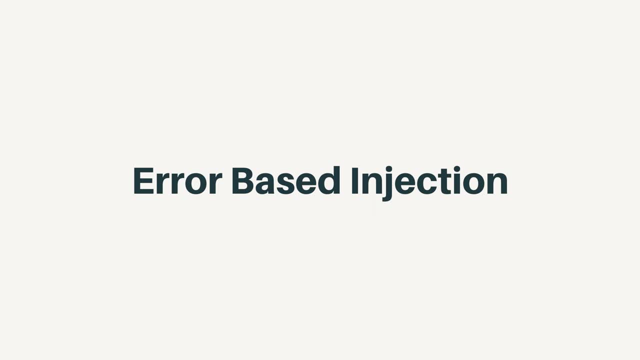 injection. in certain websites you might have seen that when you do a search or you click on a button, it sometimes throws an error. that error is coming because there is some problem in the database, and when we are able to take advantage of the errors to inject our SQL, that is where we use the error. 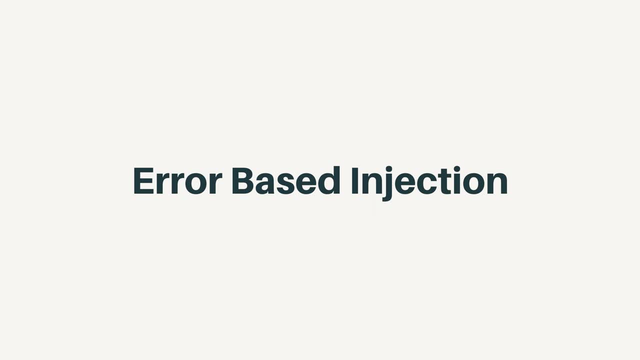 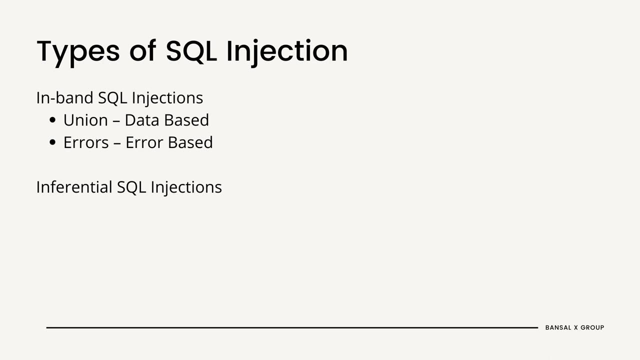 injection technique. that is where we use the error injection technique. that is where we use the error based injection techniques again. I'll have a separate lecture on this. so till now you understood that there are two categories: in band SQL injections and inferential SQL injections. in in band you have the database technique called. 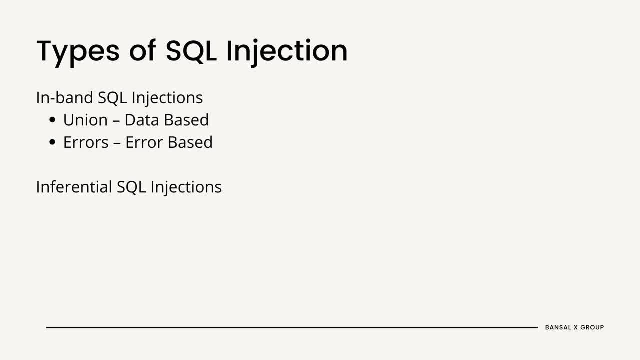 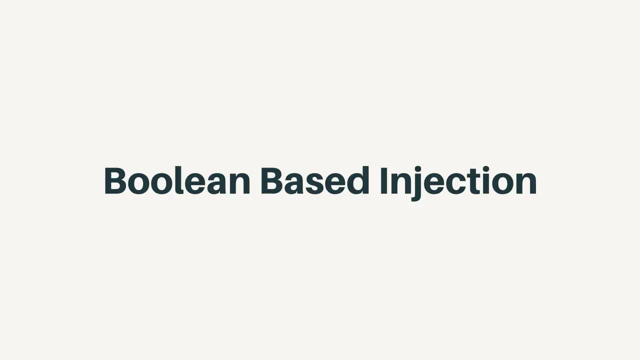 Union based injection and the error based technique called error based injection, now coming on the inferential injection. in certain cases you will not get the error, neither the data. there you have to analyze the behavior of the application. either you are logging in or you're not logging in. it's not throwing any error. 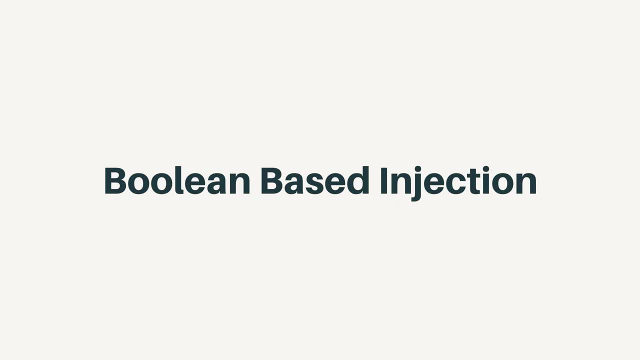 that password is wrong, username is wrong. it's not giving an error, it's just letting you log in or you're not able to log in. that's where you analyze the behavior. am I able to log in? that is a true statement. is it not allowing me to? 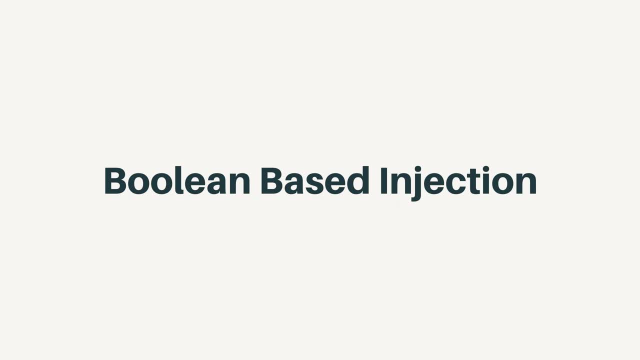 log in. that is a false statement. this true and false is called as Boolean injection technique. similarly, you can observe the time taken by this server when you request a page. it may take five seconds to open that whole page. in certain cases, it may take 20 seconds to open the same page. that is. 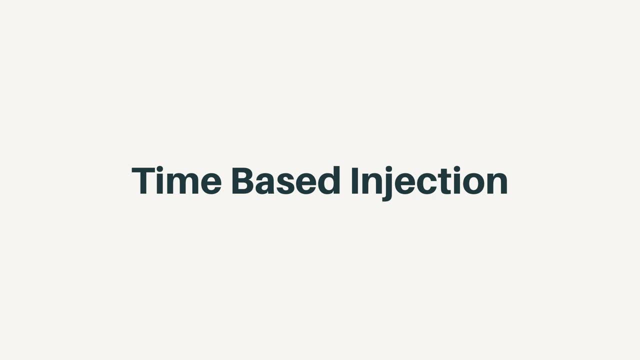 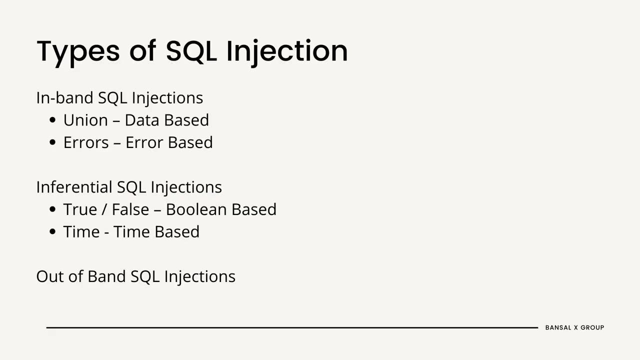 where you can analyze the time taken by the server to process some requests, and that is known as the time based injection techniques. so, as a recap, in inferential we do not rely on data or errors, rather than the behavior of the application. either we will get true or false behavior, which will lead to the 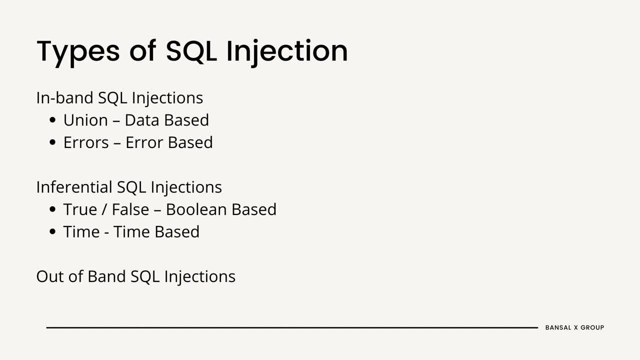 Boolean injection technique, or false behavior which will lead to the Boolean injection technique, or we'll get some time differentiations which will lead to time based injection techniques. well, there even exists a third type of technique, which is called as out-of-band injections. the reason I'm not discussing 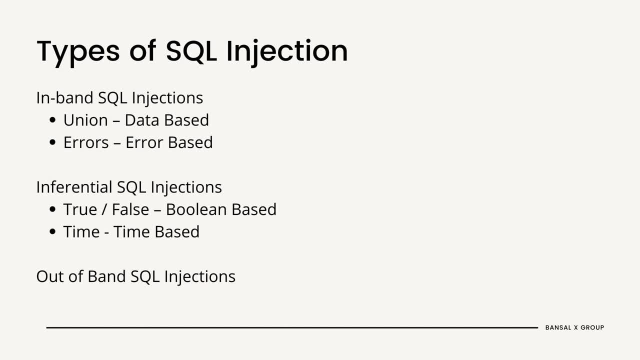 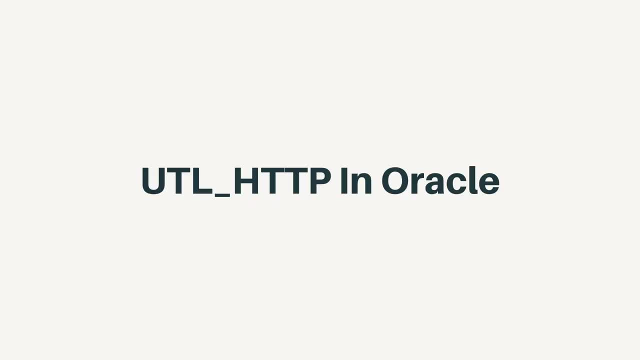 this- and we will not even be covering this in the course- is that out-of-band is a very rare situation. it is not even applicable in every SQL product. for an example, this normally is found on databases which are from a brand called Oracle. there is a special package that is called Oracle and it is called the. 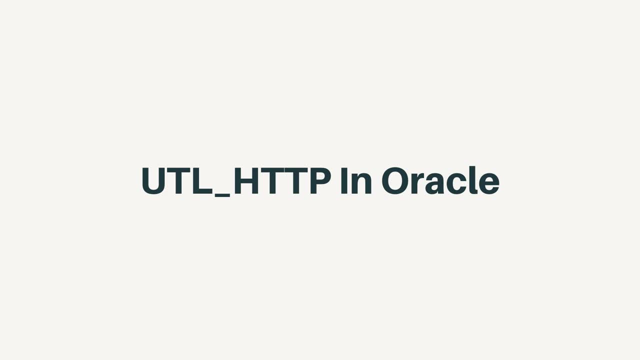 package in that called UTL underscore HTTP, with which we can get the response in our netcat listener. so you can set up a netcat listener and you can get response of your queries in your listener. it's highly rare situation and will not fit the scope of this course. that's the reason we will ignore out of. 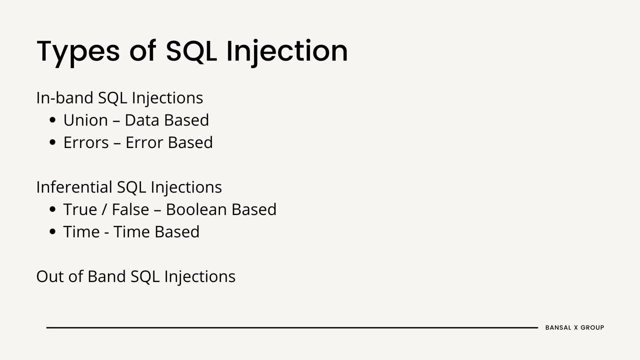 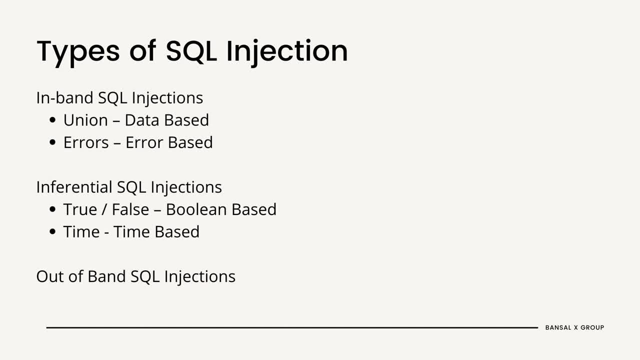 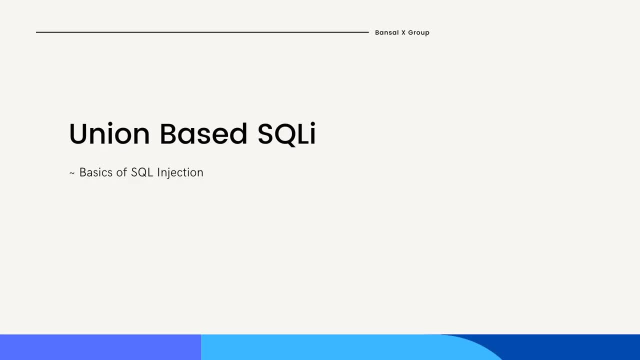 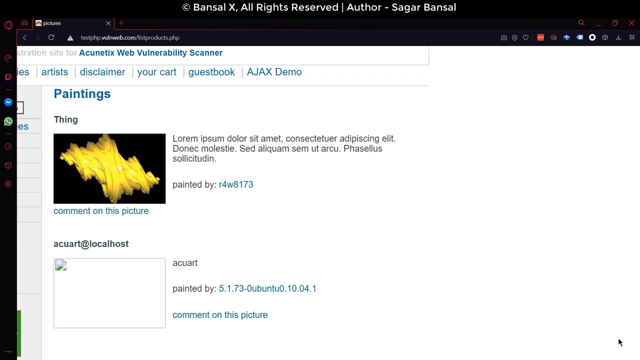 netcat listener being hosted by you. so these are the three categories of SQL injections and we will be covering the first two in the following lectures in detail. union-based SQL injection. well, the union-based SQL injection occurs when we are able to use the union operator to combine the output of two. 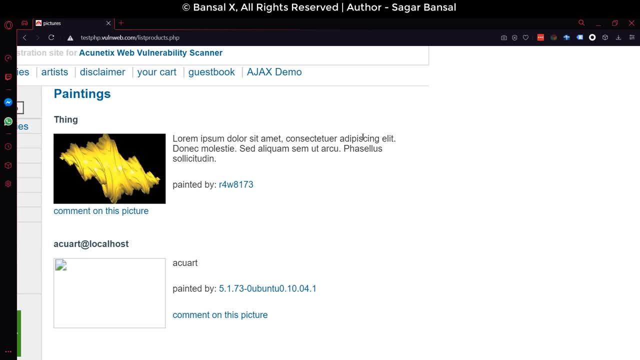 select statements, as you can see in the following screen, this first image, which has some lorem ipsum text and has a author name with a link and actually an image, is the result of the website's default code. however, I was able to create a virtual image which you can see right here, which doesn't exists, which 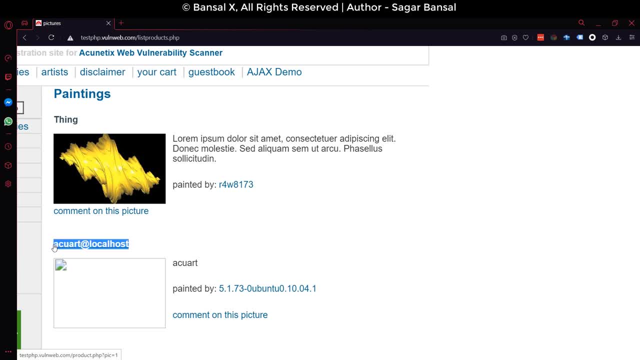 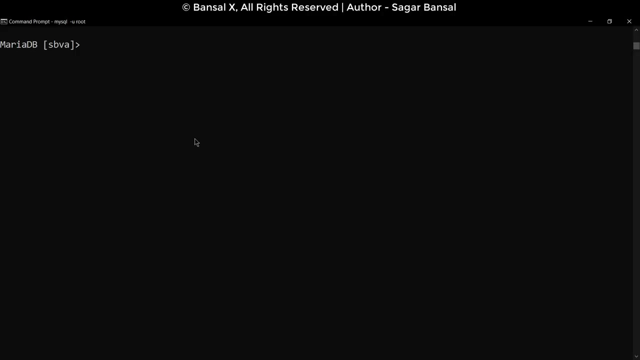 has a name as the database user. instead of the description it has the database itself and instead of the painter name it has the version information of the database. so I was able to create a virtual row and extract data through. that seems complicated, right? let me make it easy for you. I have two tables in. 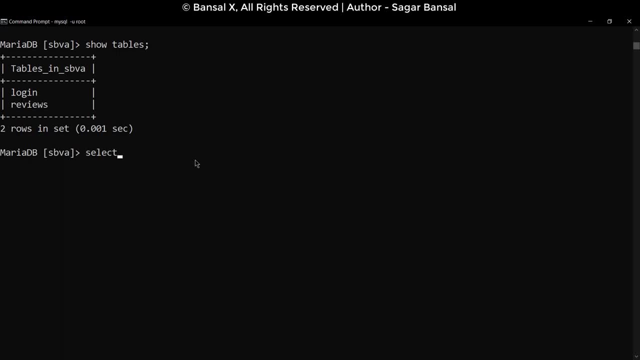 this database. first one is login. if we see the login table, there are three columns: ID, username, password, IDs. one username is Sagar, password is Spencer. just one record. now, if I use union operator and I tried to combine one, two, three, I will be able to combine another row which has the value one. 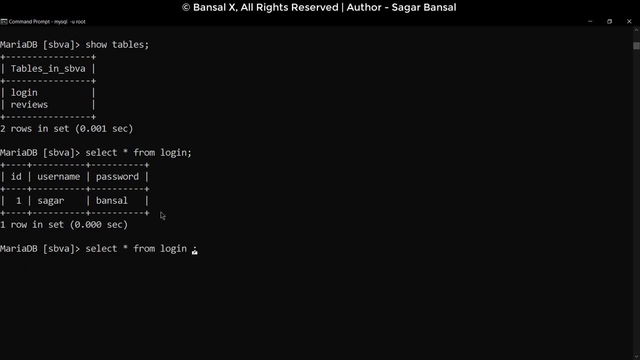 two, three. let me show you how that works. as you can see, I just tied select star from login union, select one, two, three, and there is certainly another row which has the value one, two, three. this will only work when you are giving the exact number of columns. if I try to give only one and 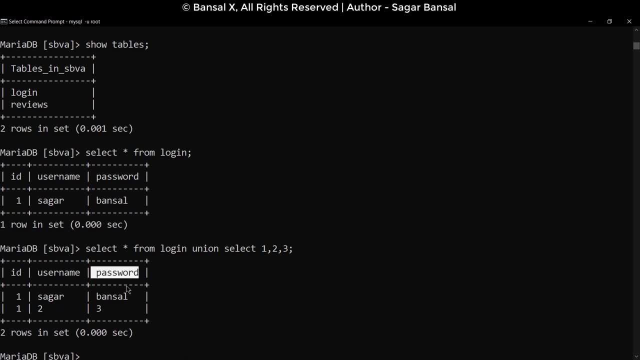 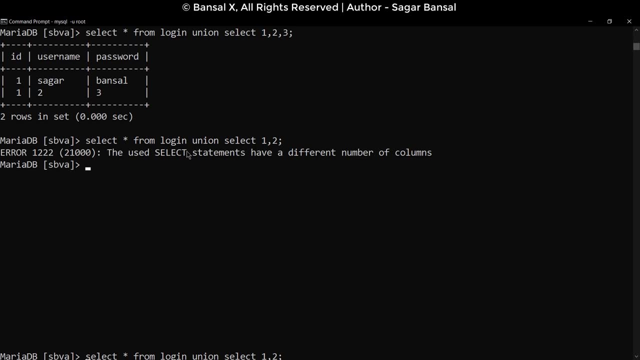 two, I'll throw an error because the third column will not have a value to put in. as you can see, when I try to give only select 1 & 2, it says the select statement have a different number of columns. So it should always be the same number of columns which are putting here. 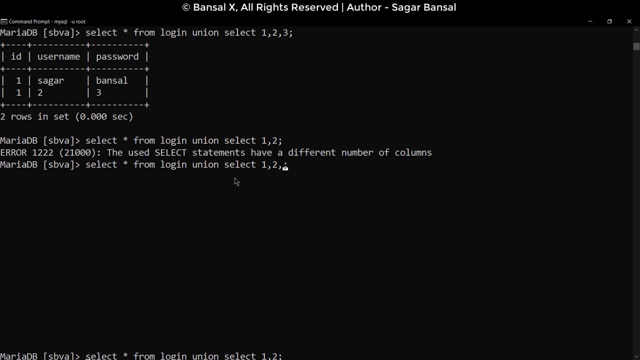 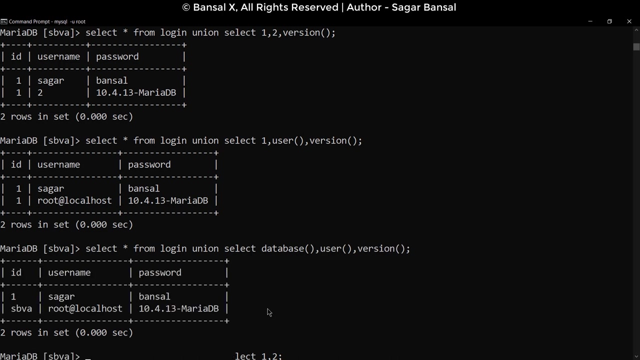 Now I can go ahead and extract data instead of three. I can put version and I'll throw up the version number Instead of one. I can put a username and throw the user instead of one. I can put the database: I'll throw the database name. Seems easy, right, So I can just copy this thing. 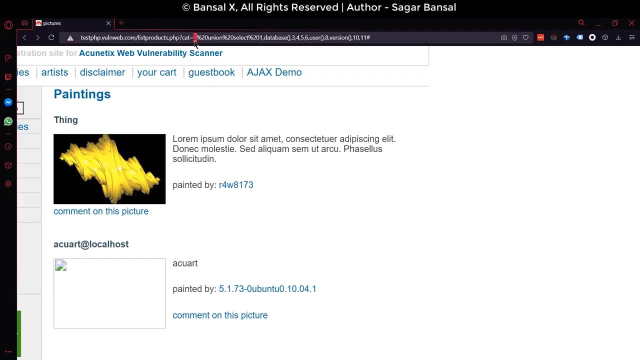 and take it to this website and run it, and it will work, Will it? Well, no, it won't. It'll throw an error. Let me show you what You can see. it says: the SELECT statement has different number of columns. 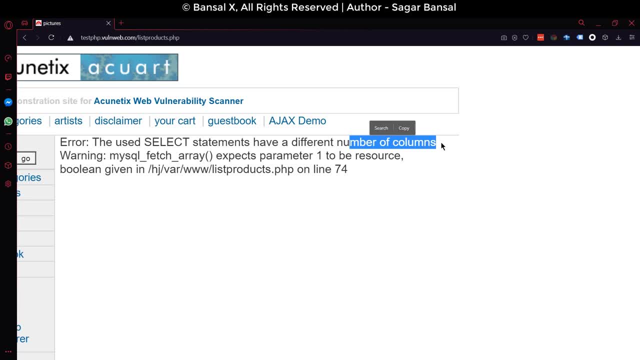 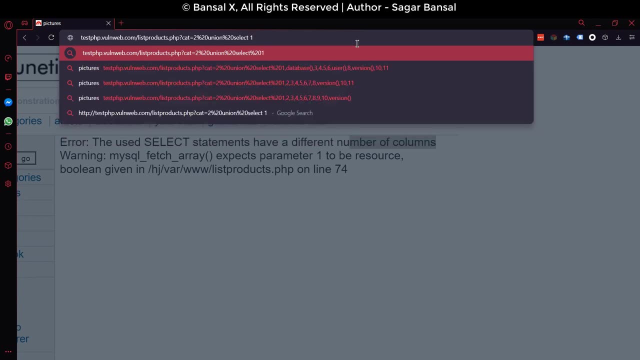 You cannot expect them using three number of columns, right, So they might be using four columns or five columns or six columns. There are two ways to find columns. First is brute forcing, where you can try SELECT one. That doesn't work. Then you can try SELECT one and two. 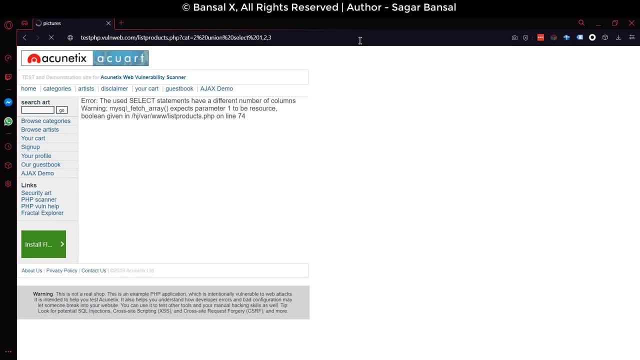 That also doesn't work, And you can then try SELECT one, two, three. And you can then try SELECT one, two, three. That will also not work, But this method may take a lot of time. Hence we can use an efficient method which is ORDER BY clause. 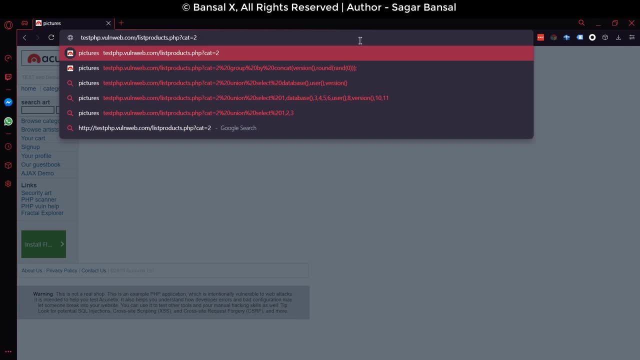 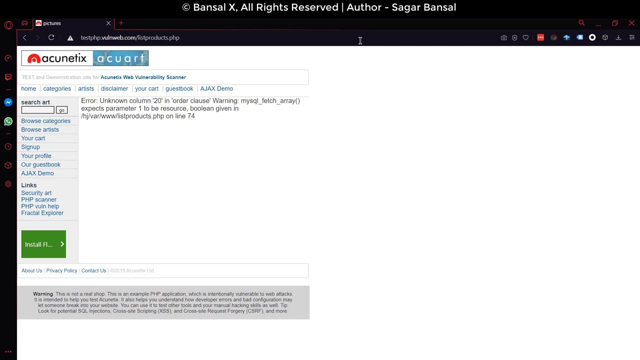 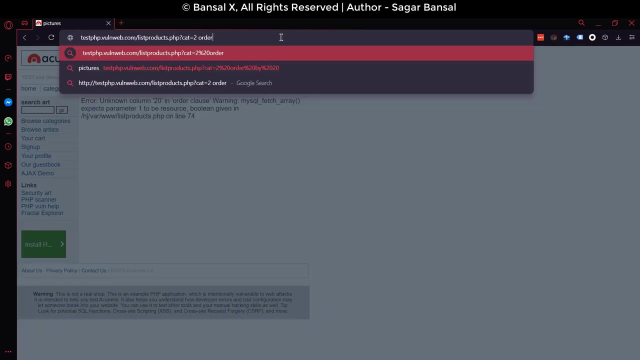 Instead of putting SELECT statement, I can put ORDER BY And I can say ORDER BY 20.. And it says unknown column. 20 in order clause means that the number of column is less than 20.. If I try 10 now it works, which means the number. 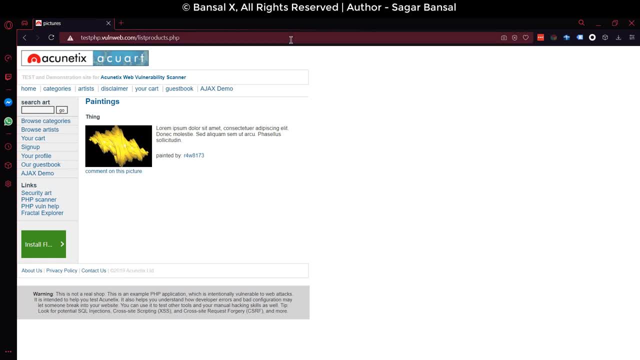 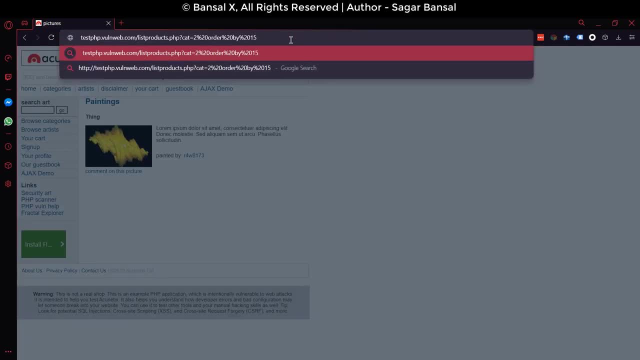 of columns is either 10 or more than 10.. So now I know they are in the range of 10 to 20, I can use a middle range which is 15. And that throws an error. So unknown column 15,. 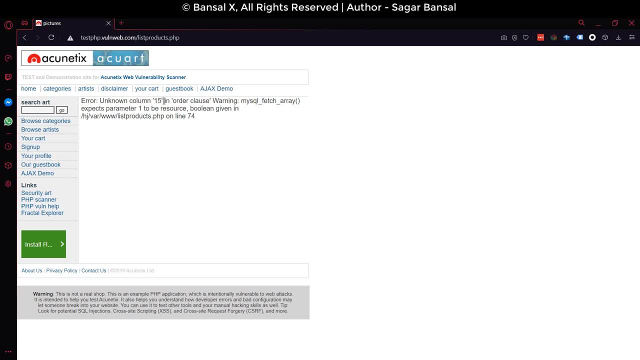 it means our columns are in between the range of 10 and 15.. Now I can put 13.. It still throws an error, which means our number of columns is either 1011 or 12.. I can put 11. That works, So either. 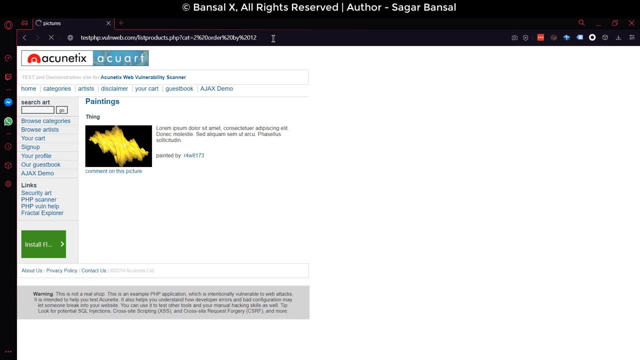 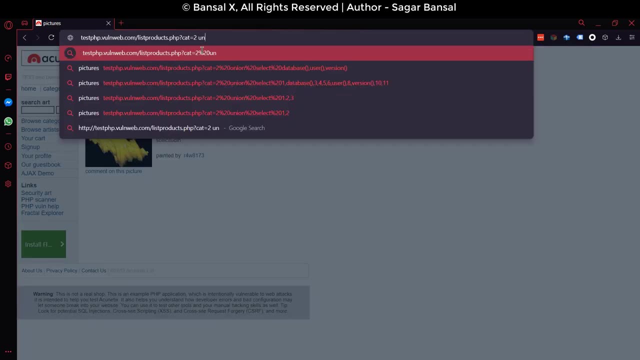 11 or 12.. Well, 12 throws an error, which means the number of columns in this application are 11.. Which gives us the output. So I can say now select 123456789, 1011.. Now you can see it creates. 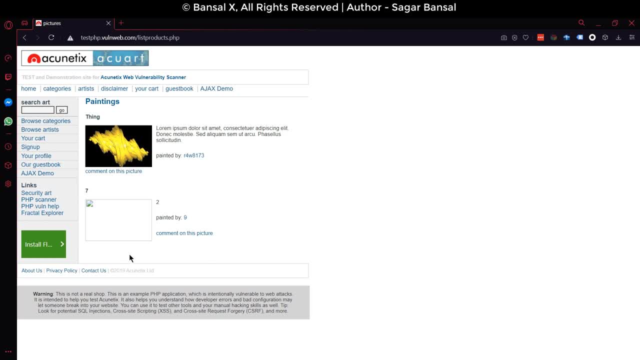 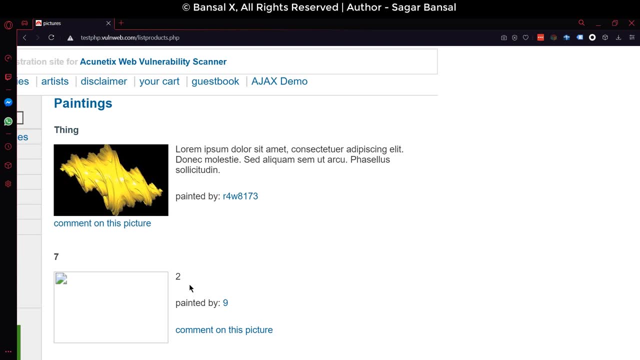 a virtual table. But point to understand here is not every column is accessible. I can see seven here, I can see two here, I can see nine here. So I can extract information through column number seven, through column number two and through column number nine. These are three. 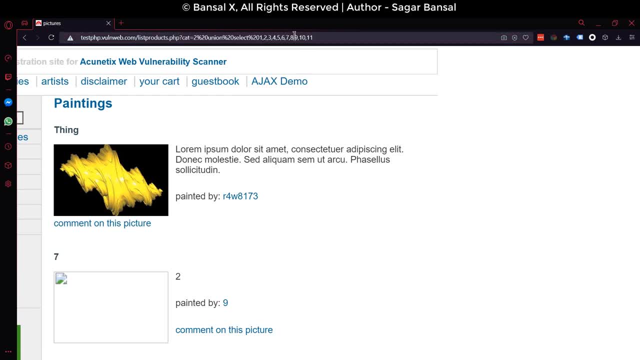 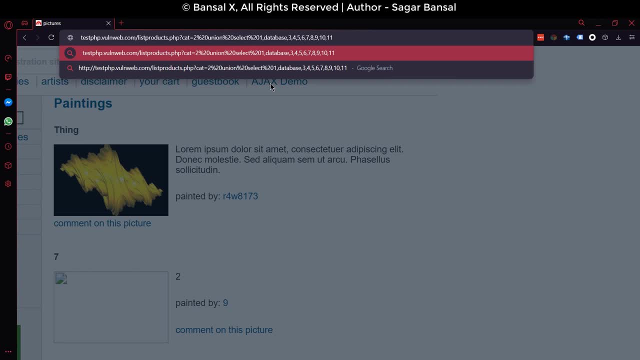 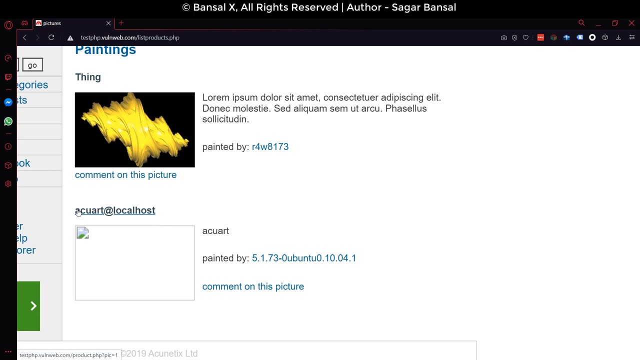 columns where I'm getting the information. Hence I can put my database, let's say in column number two, In column number seven I can put the user And in column number nine I can put the version And you can see. we were successfully able to find. 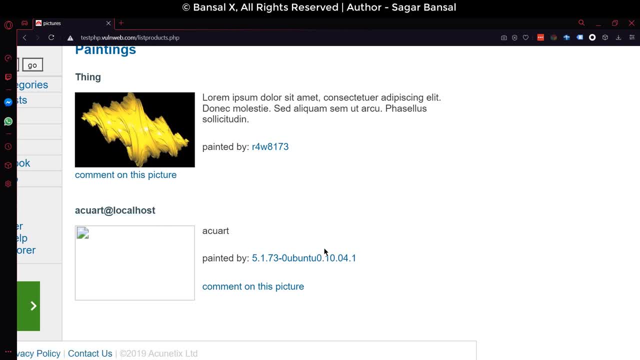 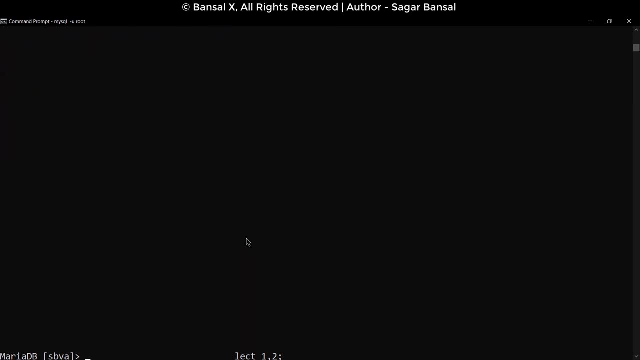 the username, the database name and the version. Can we take it forward? Of course you can find any information that you like. Can you find other database? Yes, It depends on how deep you understand SQL language. So in order to find all the databases, there is a special table called information schema. 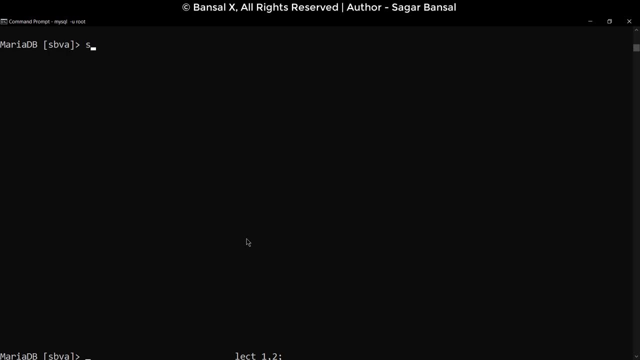 schemata. You can find that using this, There's a column called schema name In a table called schemata, in a database called information schema. As you can see here, the first database is always information schema, which contains this table schemata. 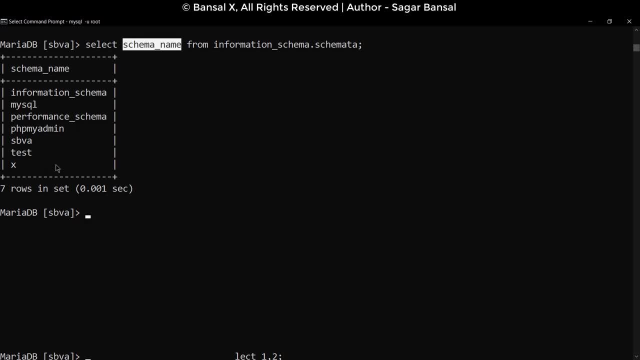 which has a table column called schema name which has all of these entries. So if you query schema name from information schema dot schemata, it'll show you all the databases. Can I take this thing from here And can I put it on the website? 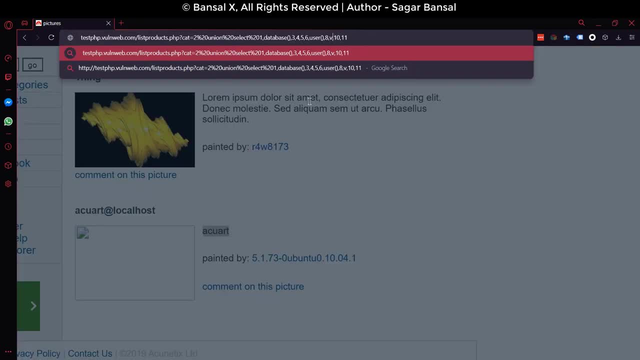 So it's all there And we can use it to find all the databases, just some of them, And in column number nine we can see we have found one which contains that information schema. This is a table that states information schema And when we click on it 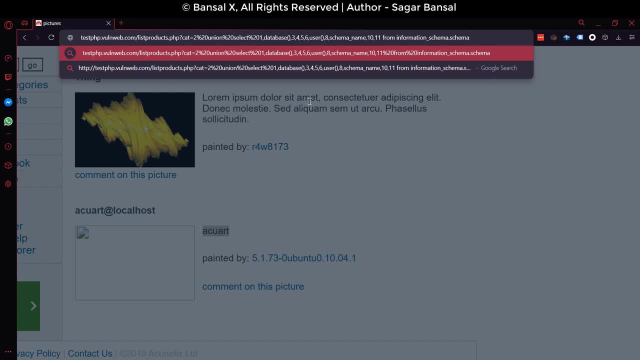 it's showing this table that contains these three different databases And it's showing us the database name, which is the database name, content, brand and the website name. But there are a few other ways to find this table. So we've got this table here. 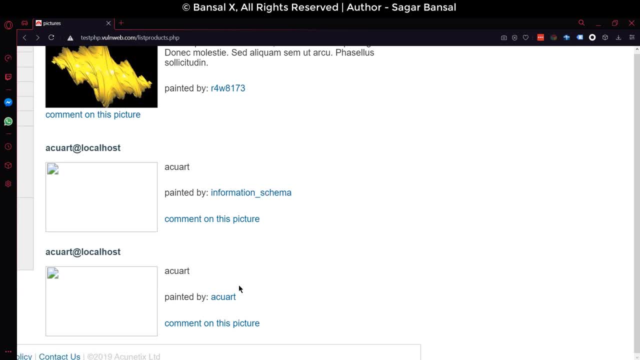 And we'll go ahead and create it. We're gonna use our source code to find the database, We're gonna use this table to find this database And let's go ahead and create a database. And now we can see: we got: first database, information schema, second database. 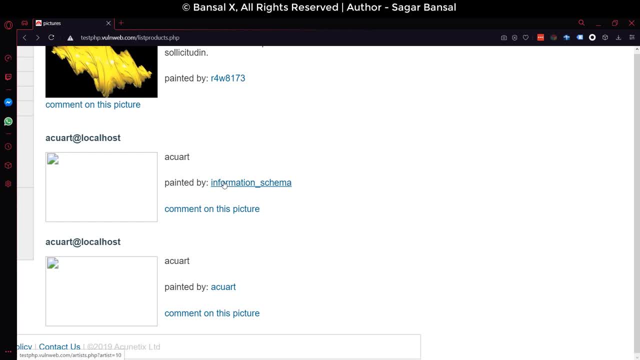 and there are no other entries, which means this specific website only has two databases. Specific website only has two databases: information, schema and acquired. I Can go in and on with multiple examples, just to give you one more examples on how to find the table names. So the query for that will be: 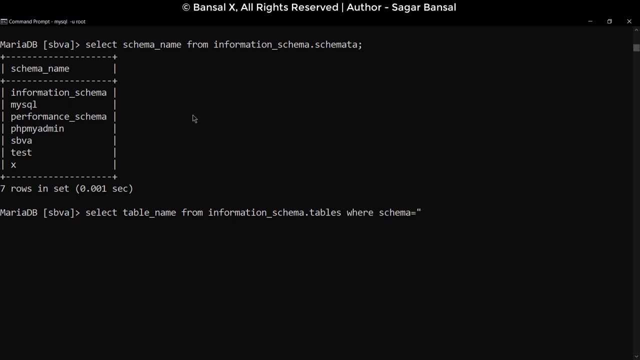 You Select table name from information schema dot tables where table schema equals X, where X is the database Which you want to find. in this case, I found the X where there is just one table called users. Can I take the same thing and put it on the website? Of course? 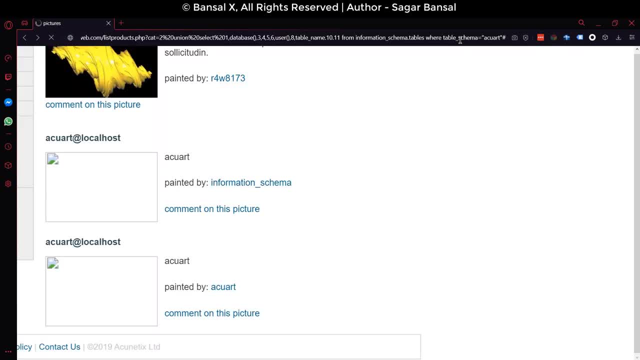 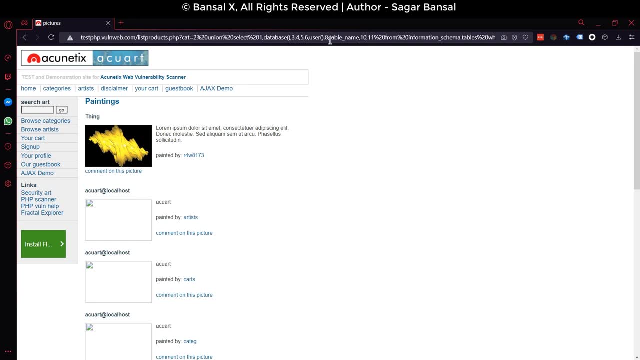 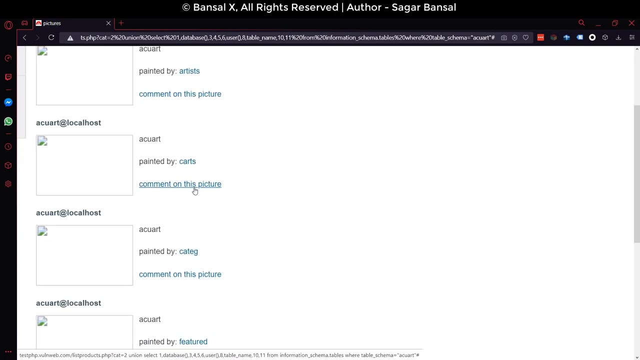 As you can see, I just found the table names. The query I used was table name from information schema dot tables where Table schema equals acquired, because I wanted to find the tables in the database called acquired and the table names are artists, cars, chaotic featured and. 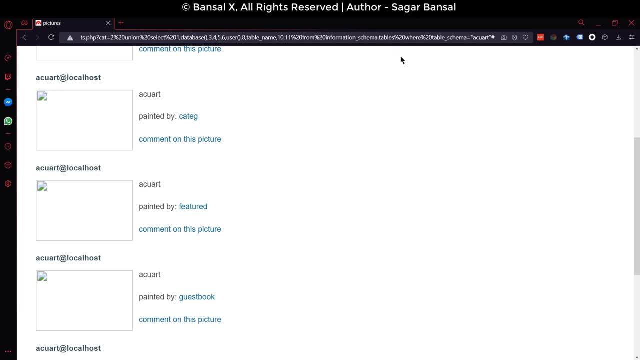 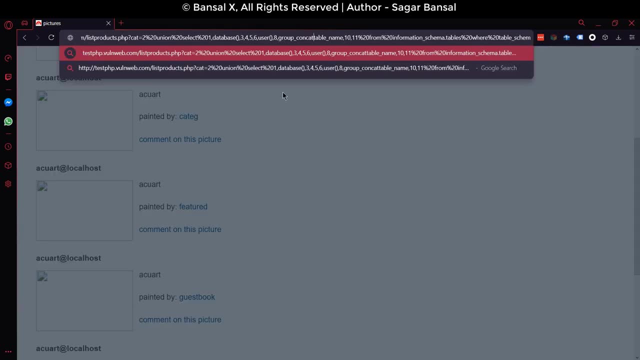 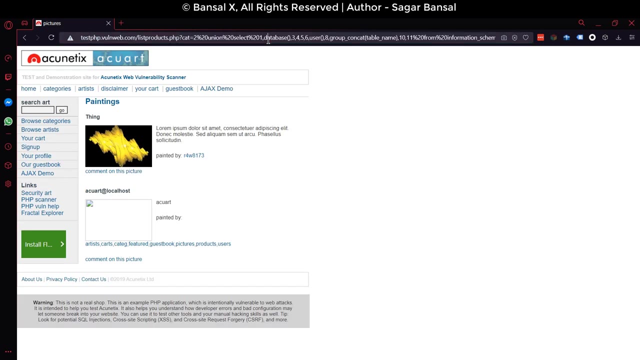 figured, gets book and so on. There is an interesting function that you can use here, which is group can cap. Now, when you use this function called group can cat- and in that I am asking for table name- You can see it doesn't gives me a lot of results. It just groups all of them together over here, painted by 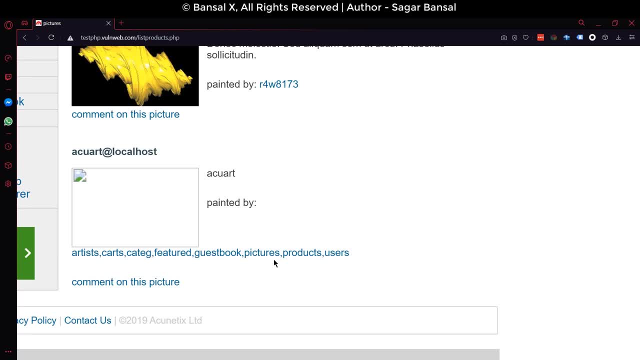 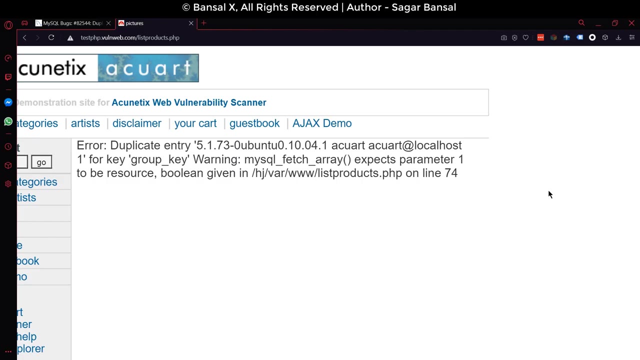 artists, cats, cat-hack feature, gizbo pictures, products, users. So everything in one line, super clean stuff. And that's how you do union base SQL injections- Error-based SQL injection. Well, an error-based SQL injection occurs when you are able to trigger certain bug in the product. 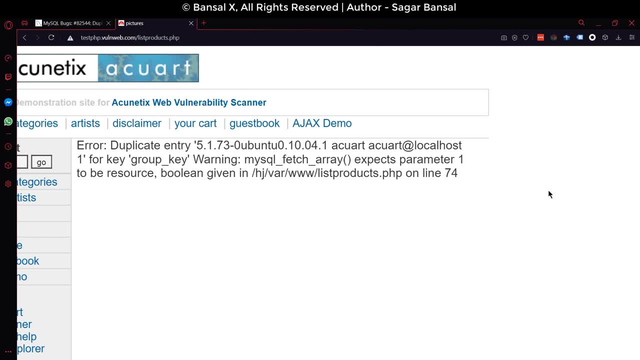 Which leads to some errors, and you have the ability to control those errors, to extract data. in the following screen you can see that I was able to create an error which is about a duplicate entry in the group key, but in this error you can see I was also able to extract the version number. 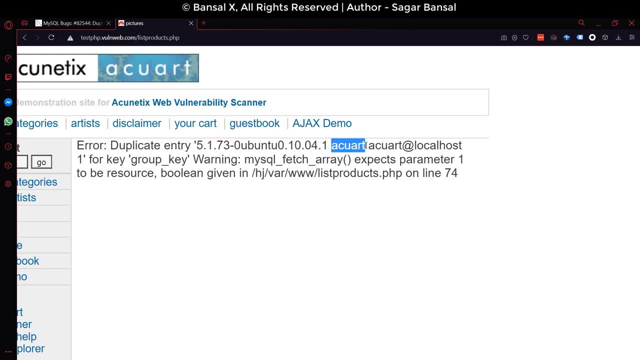 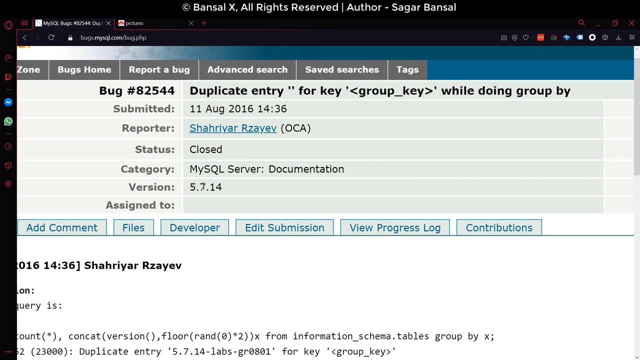 of the database, the database name and the user of the database. this is what an error-based skill injection is all about. now, as I just said, this depends on the product and a bug in that product. you can see that this version is five point one point seven. let me show you a page here. you can see five point seven point. 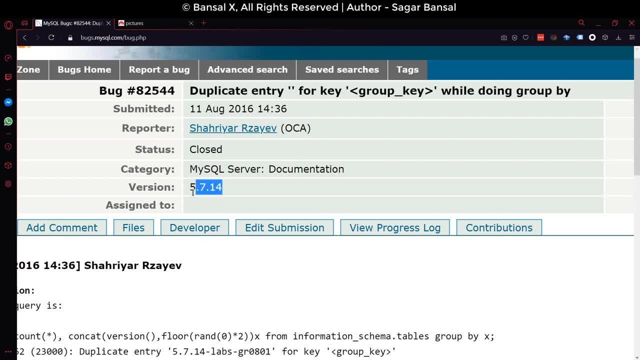 one, four, so I'm using a much older version on that website. however, this bug ID eight, two, five, four, four. this bug is valid in all the latest versions, in 2020 as well. it was published in 2016, but even after four years, this has not been. 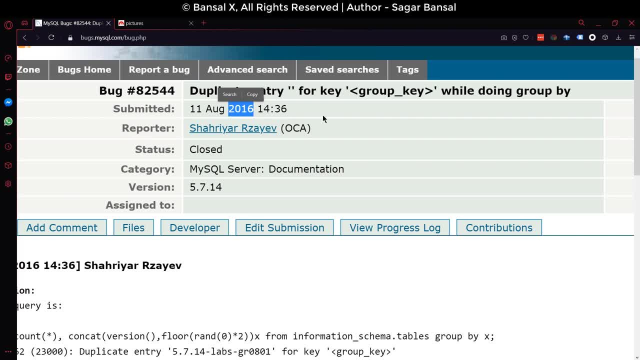 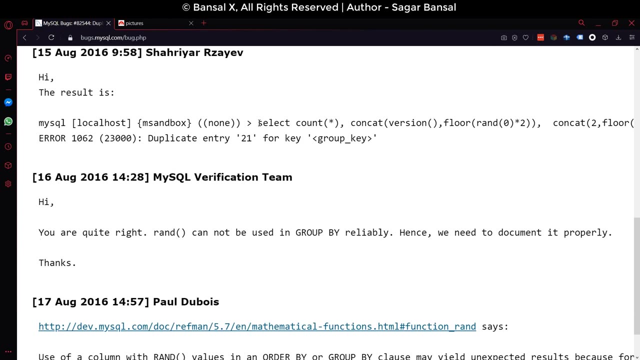 passed and looking at the history, I don't think so. it's going to be passed soon. so the bug is about a duplicate entry in the group key while doing a group by clause. if you go ahead and scroll down, you will see that you can create this error by selecting something, counting it, concatenating the stuff with. 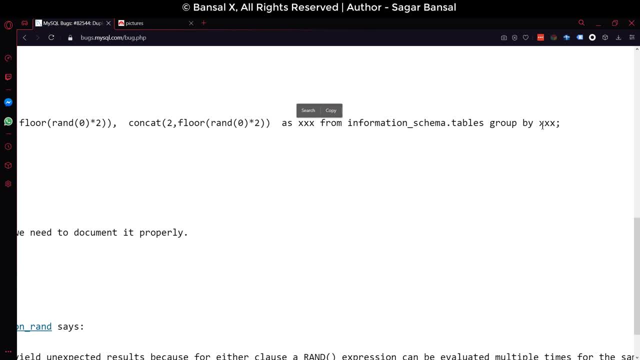 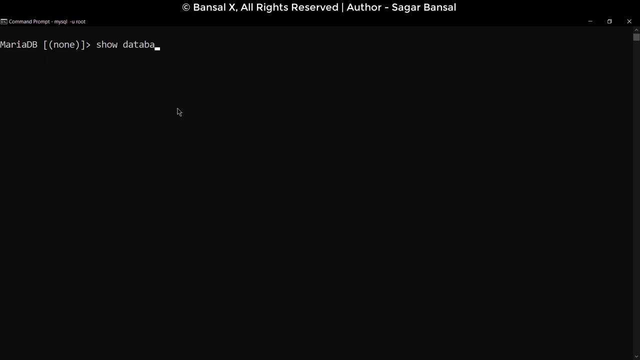 the round function concatenating with floor function from certain table and grouping it by some value sounds complicated, right? don't worry, I'll break all of this for you. so I'm going to show you all of this in my test environment. I do have the following databases. I will use X for this specific test. there is just one table in this. 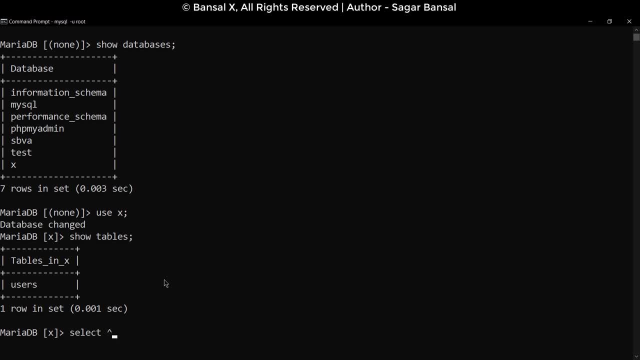 database called users. in this specific table, there is one column called name and there are three rows saga, Alice, Bob. now, this error occurs when we are able to associate a random pattern. for that, the first step is to associate a random value for each of the results. to do that, we use the round function. 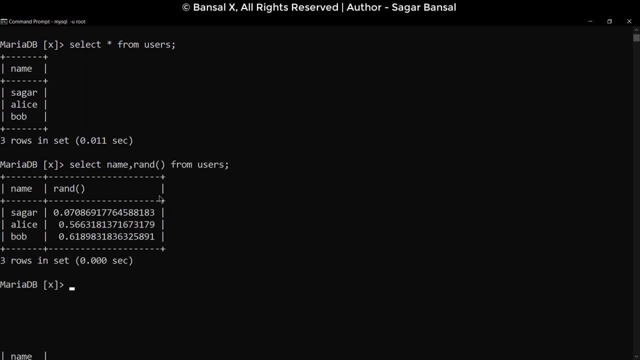 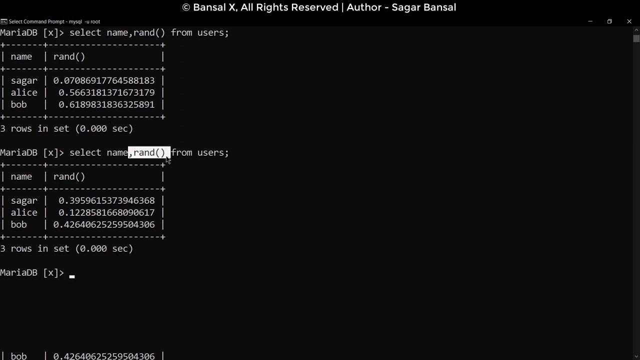 as you can see, when I select this column, which is name, it returns three rows. but I also selected a random function which is creating three random values in front of these. since it is a random function, anytime I create this again and again, it'll create all new values. you can see, when I type this again, all the values. 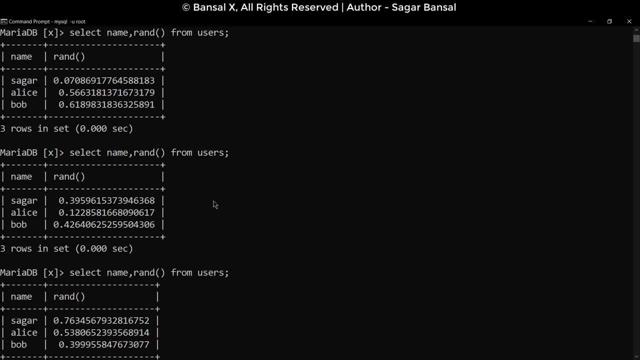 have changed. if I try it once more, all the values have changed, have changed again. These values are completely generated random and they will range from 0 to 1.. The next step to trigger this bug is to control the output of the random function. But I just 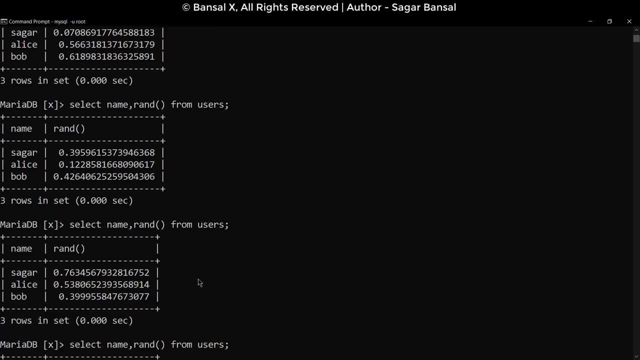 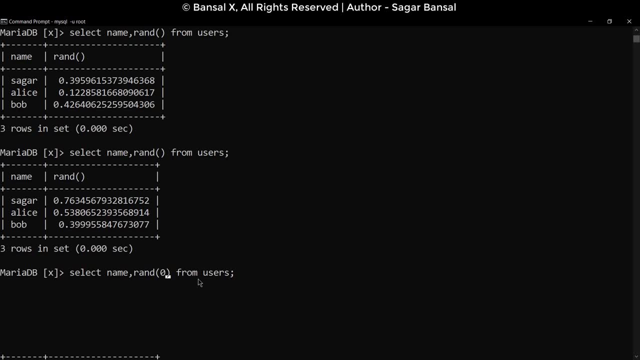 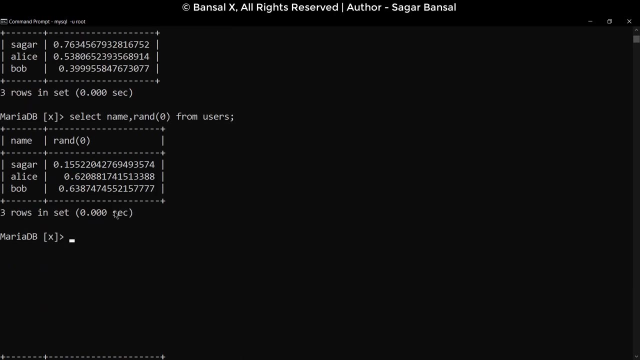 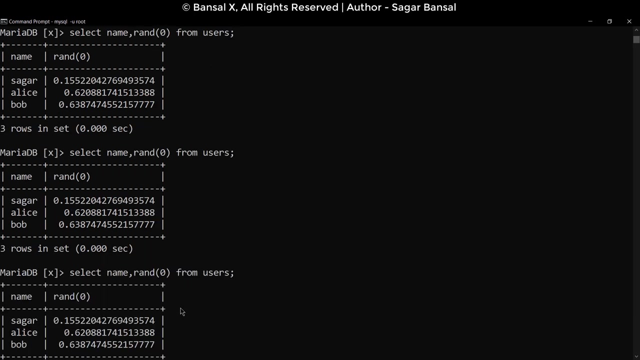 told you it's completely random. You can use a seed value. Here I will put a seed value like 0.. Now, once I put a seed value, the result will always be same. This is what comes when I run it once. This is what comes when I run it twice. This is what comes when I run it thrice. You can. 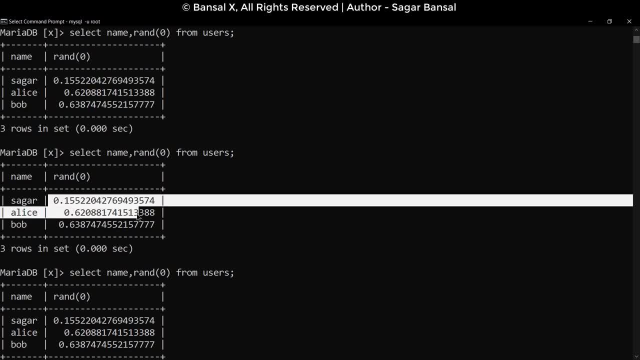 see all the times it's generating the same three values. Now the next step is to create a duplicate entry, But my question is: do you think this number is going to be the same as the previous one? Does it have any probability to come on this place or on this place? These are billions of. 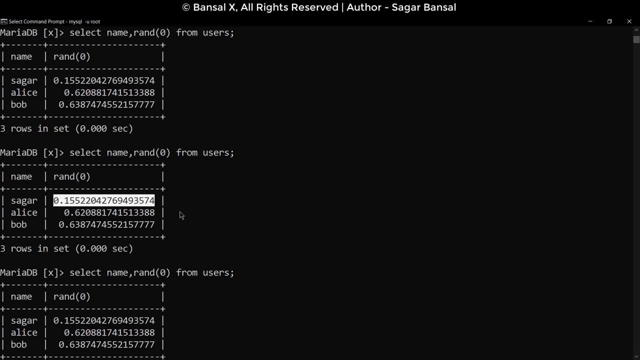 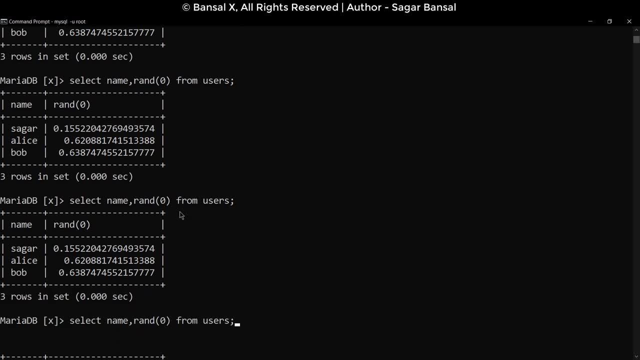 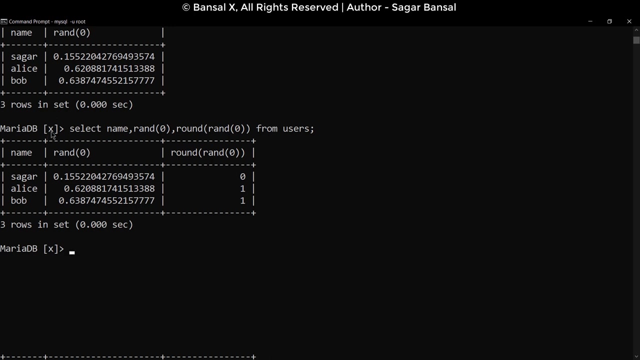 combinations. So the probability of this is almost impossible. For that we will use a rounding function. Let me tell you how that works. So in the following example, I just added a round function on top of our round function. Hence it is rounding the values to the closest 0 or 1.. And now there is a 100% probability that our 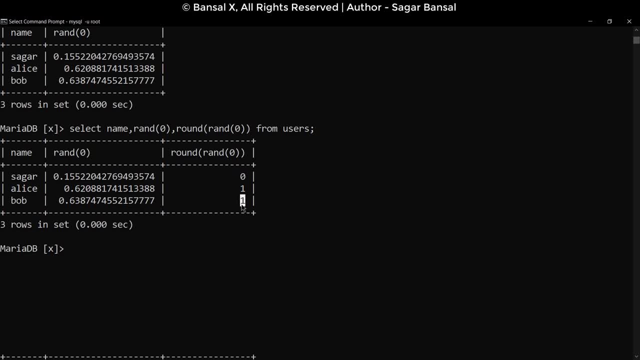 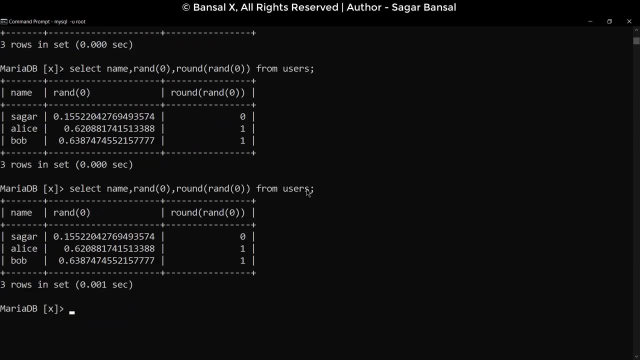 value will repeat and there will be a duplicate entry, since it will always be 011.. It doesn't matter how many times I try this, it will always be 011.. You can see it never changes Now that we are able to generate random values which are still. 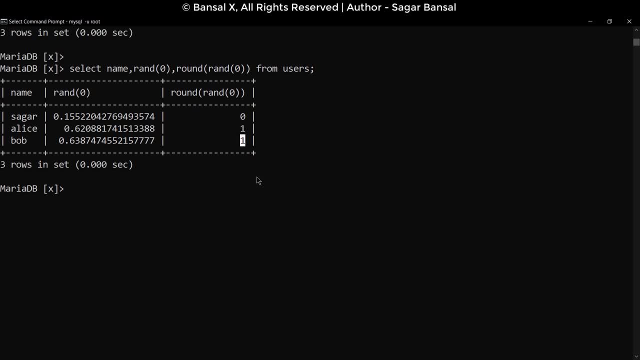 controlled by us and we know that it's going to create 011, and this one is a duplicate entry of the above one. we can use the group by clause And I can see when I use group by and a round rand, the results are not three but rather two. 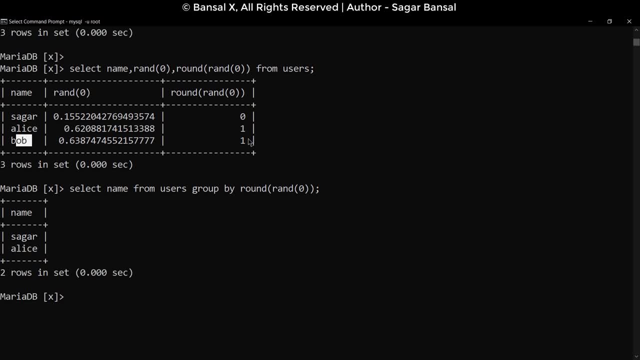 because this Bob is also having the value of one and Alice is also having the value of one, Hence they have been grouped together. Finally, to trigger the bug, we just need to put having min 0. And you can see duplicate entry, one for the key group key. That's debug, Another approach. 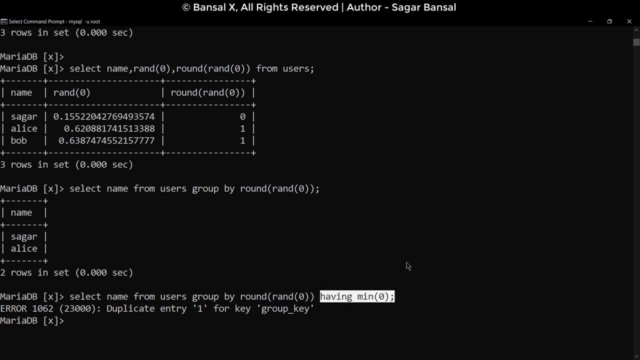 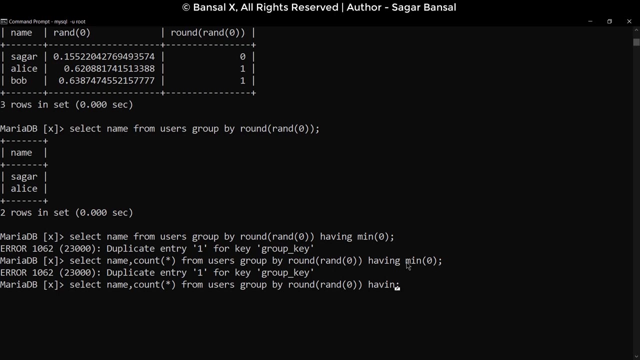 which the official guide says, instead of putting having men, you can put count. So the count will come here And if I remove the having thing, it will still trigger the bug, because bug is coming from count. Now this may sounds interesting that this count is able to create the bug, but it's almost useless. 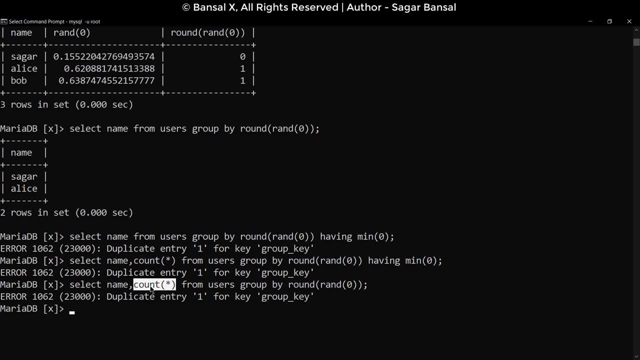 when using error based injections. The reason is that most of the times, this select something from something statement is locked and we can only modify this part. Just to give you an example, it may be select name from users where name equals saga, and then we can modify the group by round. 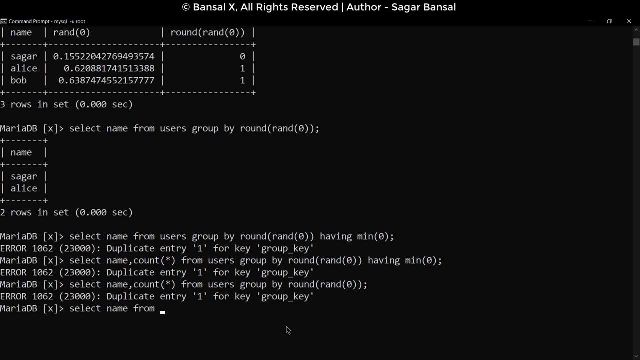 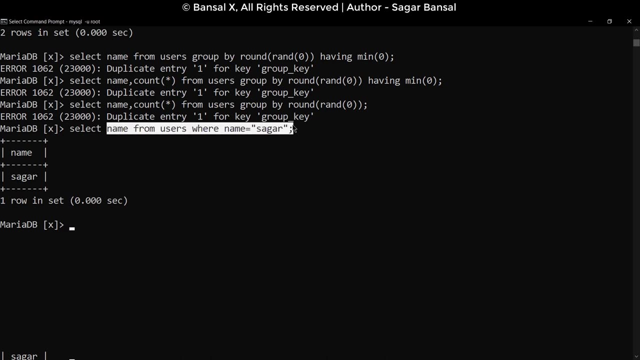 function. You can see this is a standard database query: select name from users where name equals, and we put this name in some search box. The problem of this is it is always going to give you one result. however, we need at least three results for this bug to trigger. Hence we can. 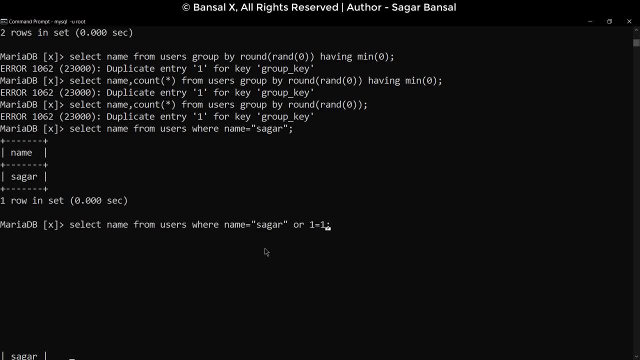 put, or one equal one to nullify this. where statement. So think about it: select name from users where name equals saga, or one equal one, which is always true. hence, it will select all the names, giving the whole table. As you can see, it dumps the whole table, So now we can put our 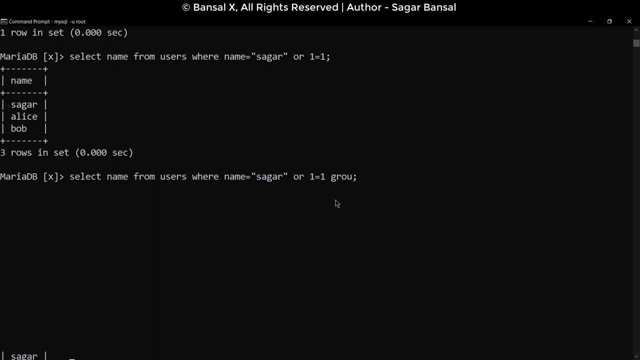 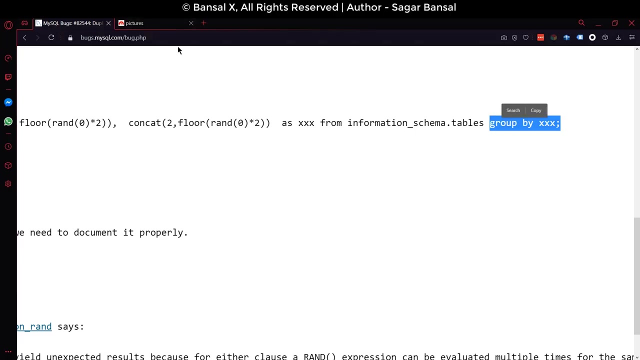 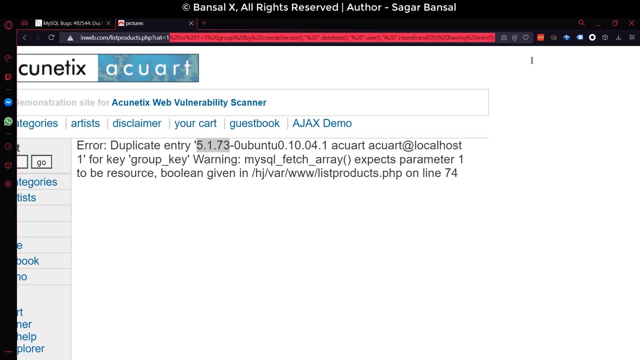 group by round having min equals zero, And this triggers the bug. And this is the final output which we want as our payload, So I can copy this. I get go on this website and you can see it normally takes a parameter called cat When 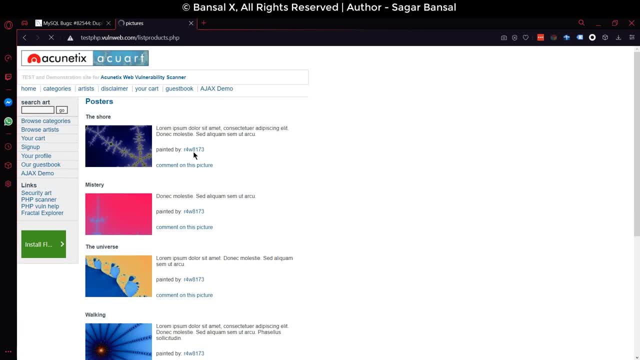 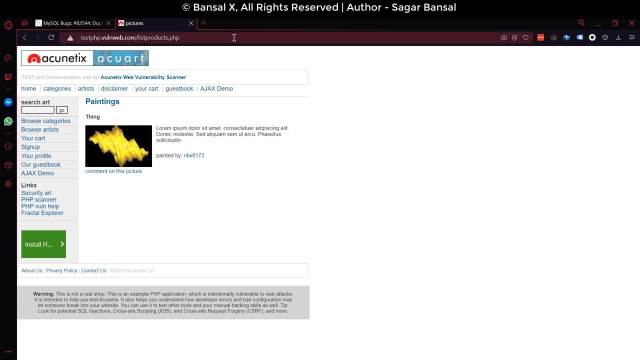 it gives a parameter called cat, we get 4.5.. So we can get if the parent is in the parent field of our cat. it comes up with all these images. If I give a parameter cat equals 2, you can see it comes up with only one result. So let me try to bypass this one: cat equals 2.. Since 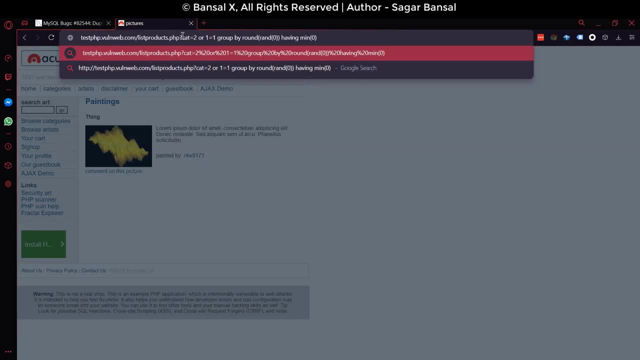 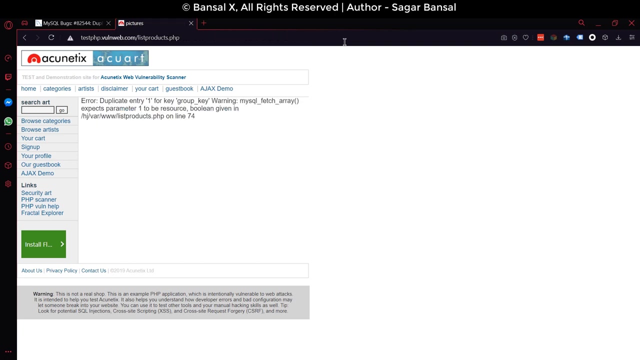 we already have, or 1 equals 1, this will bypass the situation of cat and it'll give us all the rows in the table and it'll group them by a ran function having min equals 0.. I'll put a comment here to ignore the other stuff and you can see we get the error Duplicate. 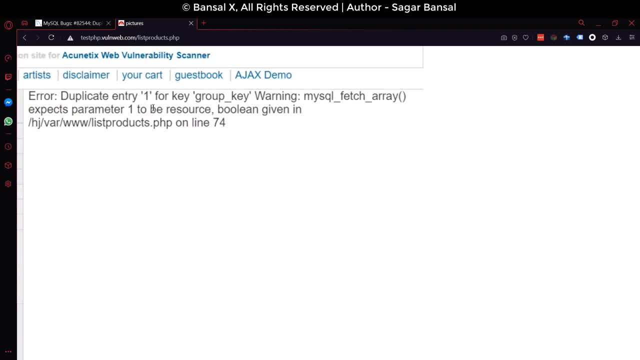 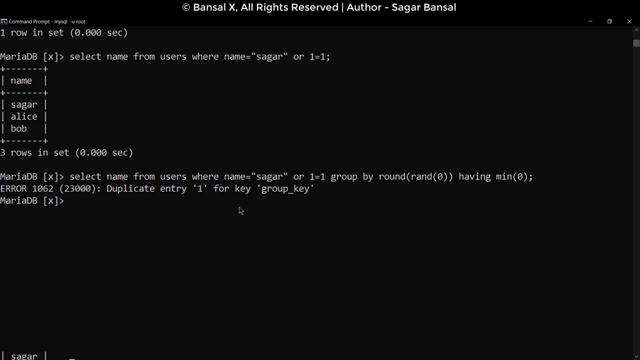 entry 1: key group key. This 1 is the result of our duplicate entry and it's the result of our ran function, which is over here. So can we use it to extract data? Of course, Let me show you that, how we can do it. 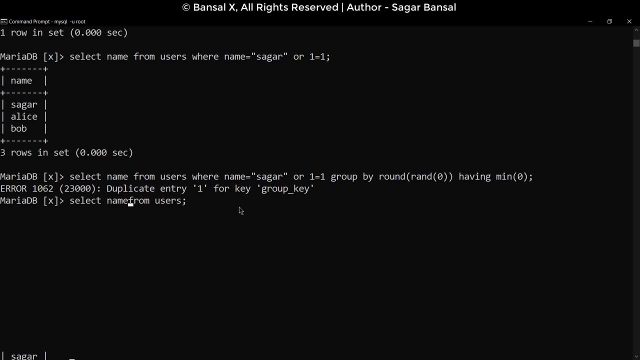 I can see. what I just did is I did a select name, round rand, and then I did a concat version, round ran. so the output of round rand is 0 1 1, which you can see over here: 0 1 1, and I concatenated: 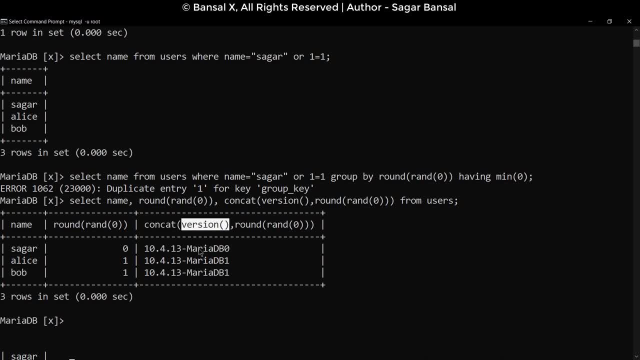 this with the version of the application. hence, you can see, since the version is constant and round rand is changing, we still have a perfect duplicate copy of 2 & 3. these are perfect duplicates because the version is constant and this part is changing. hence, in the same way we 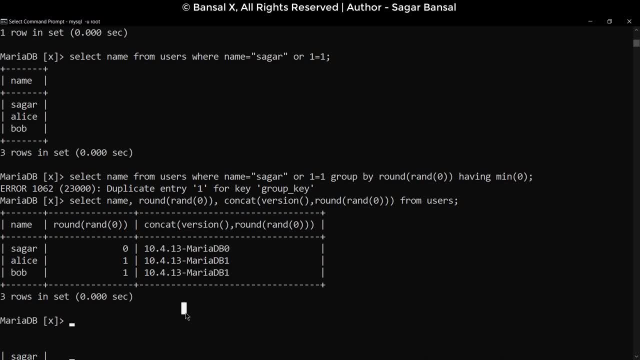 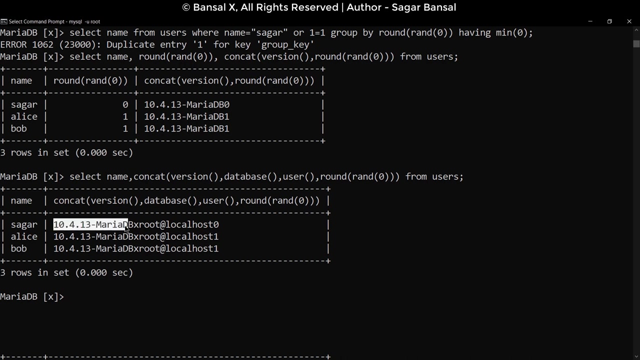 can concatenate whatever we want and we can extract data. a good example here will be: you can see, we got the database version, then we got X, which is the database name, as you can see over here. then we got a root at the date, localhost, which is the user. we can even put spaces in between. 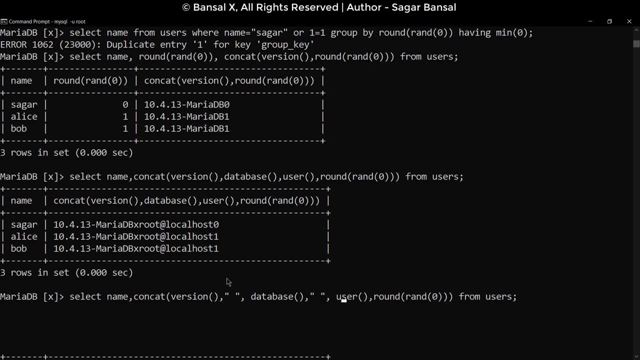 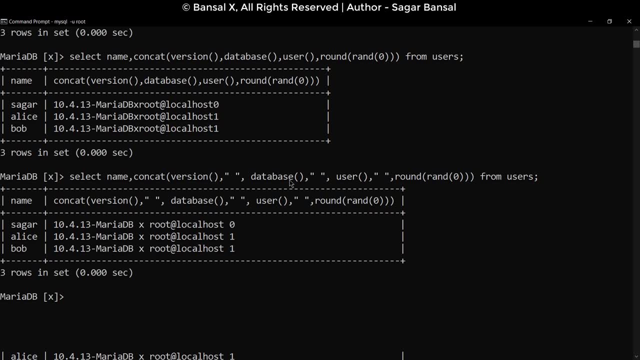 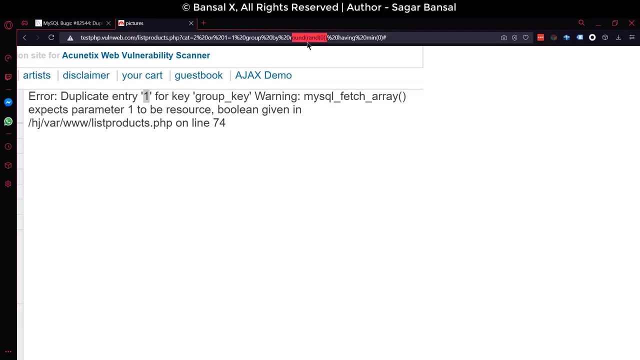 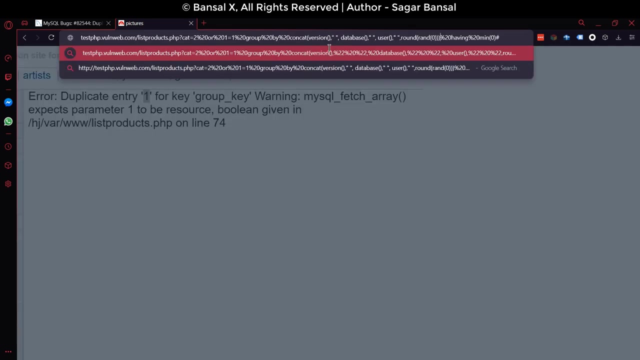 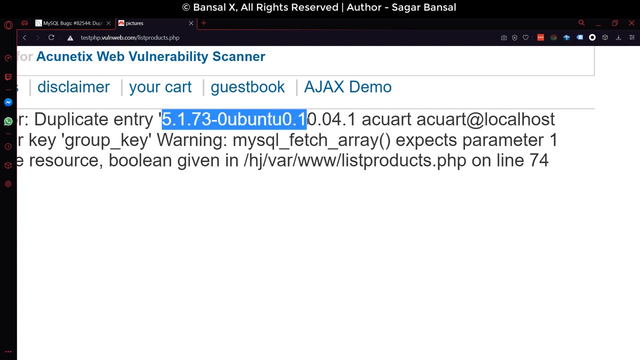 and this will just make it easier for us to identify that this is one thing, this is second, and this is third and this is finally the rand. so I can just take this whole concatenation string here and put it instead of this round rand function and we got the version number, the database name and the user at the rate localhost. that is how. 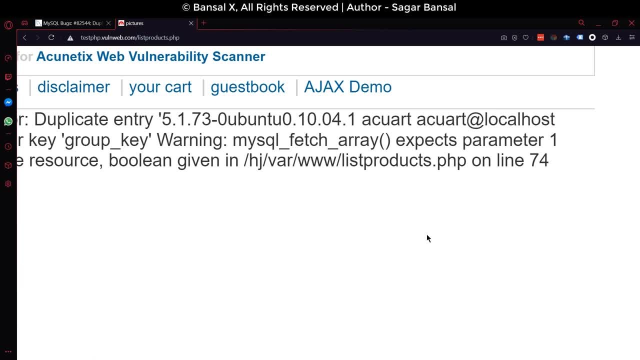 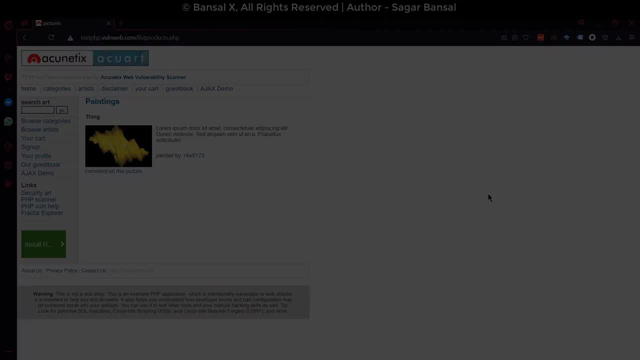 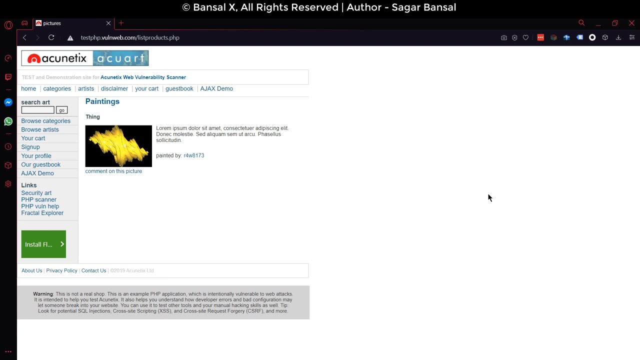 error based SQL injection works, and this is how we accelerate data through error based SQL injections. boolean based SQL injection: well, a boolean is a situation that has already been done. it will be called boolean structure. where a boolean is a situation- well, a boolean is a situation of 0 or 1, which is false or true. There will be many cases where you will find these kind. 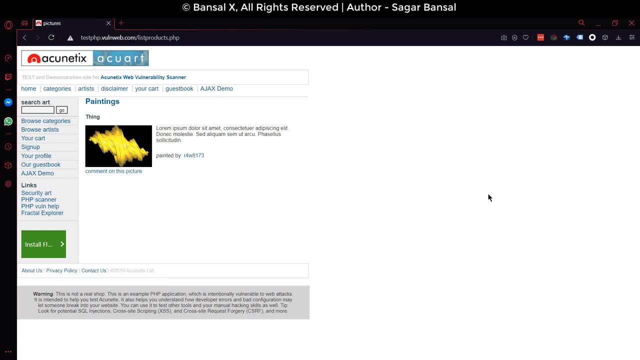 of situations. It can be a simple login page. If your password is correct, you will log in, If it is wrong, you will not. So it's 1 or 0, or 0 or 1.. In this specific example you can see if I try. 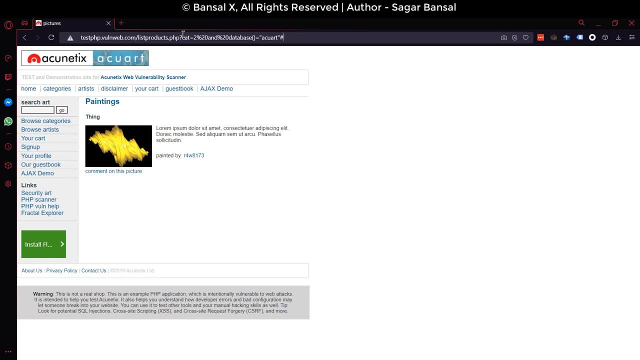 this specific command, which is cat equals 2 and database equals acquired. So I am putting a condition here: This application may be taking select star from something where cat equals 2, which should give me this image. But I'm saying and database is equal to acquired. So I'm giving. 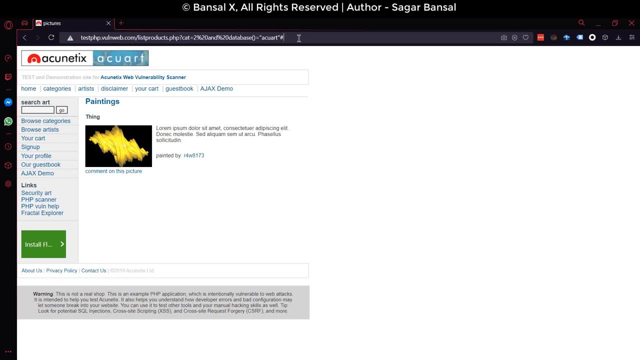 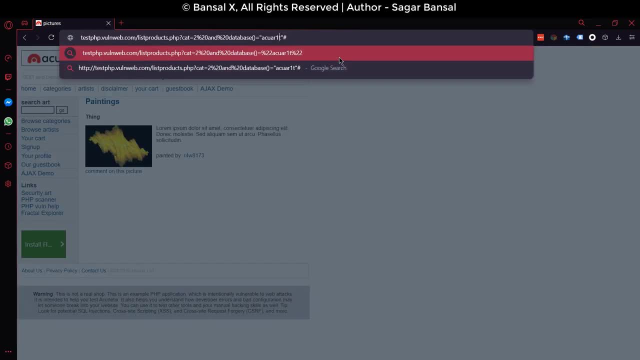 it a database name. If my database name is correct, this application will only show me the result, as you can see over here. However, if I change this acquired to acquired1,, which is not the database name, it will not show me the result, as you can see. 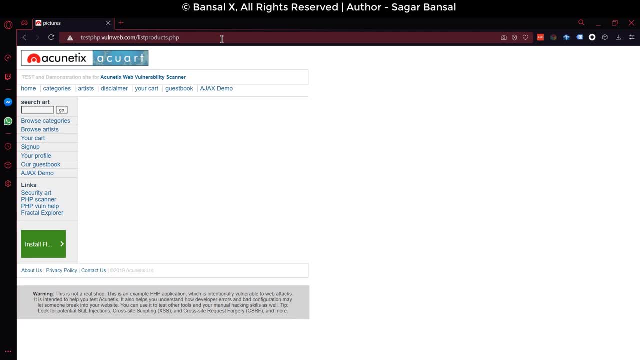 This is where the Boolean injection can be used to get data. How do you get data out of it? You can put a lot of conditions here and you can use patterns like like pattern length, pattern, substring-pattern, For example. I can name a string, a string that kind of indicates the state of the initial and what you're saying. by using aколькуny I can put out some changes. You can need some variations in here, like these strains and invariant names. change the commands Now a single repetition via this, the instruction also picturing back what I wrote in these conditions. 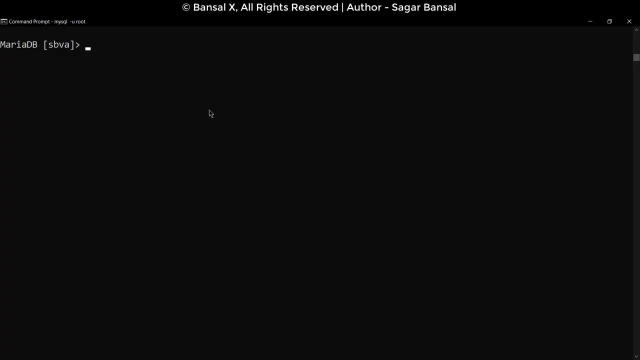 Let me show you with examples. here I have this table called login. This table has an entry which is id1, username sagar and password bunsell. Now a standard query will be: select. start from login where id equals 1, and this will: 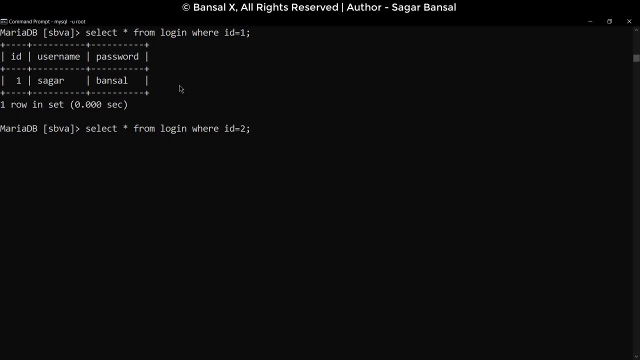 throw the table. If we say id equals 2, which doesn't exist in the database, it will say empty set, which means it will not show me anything. So instead of putting id2, I can say id1, and I know that the statement is true and I can. 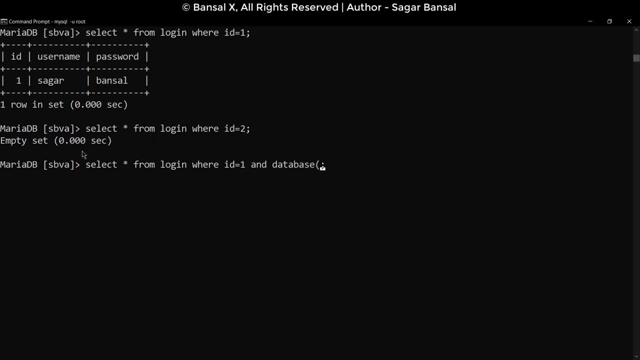 say: and database equal sbva, which is the name of this specific database. and since the statement is true, You can see we get the result. I can get the result even if the statement of first parameter is wrong. If it is where id equals 2, I can use the command or, instead of putting and: 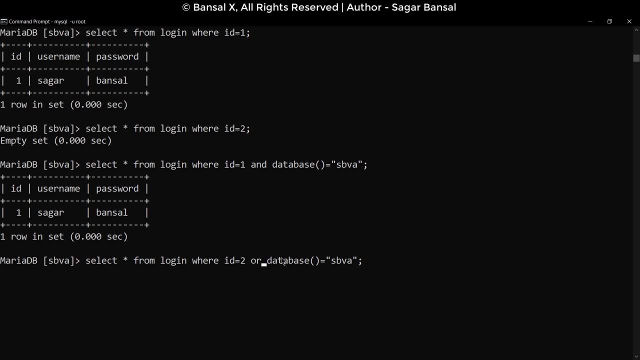 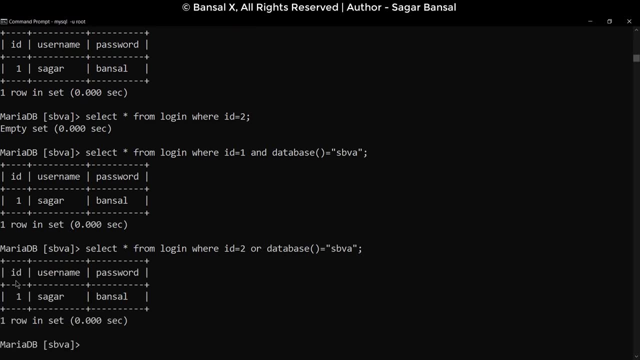 So select. start from login. where id equals 2 or database equals sbva, Now, database is equal to sbva for every single of them. hence it shows us the same table. If the first is false, you can use or to get the data. If the statement is true, you can use and to get the data. 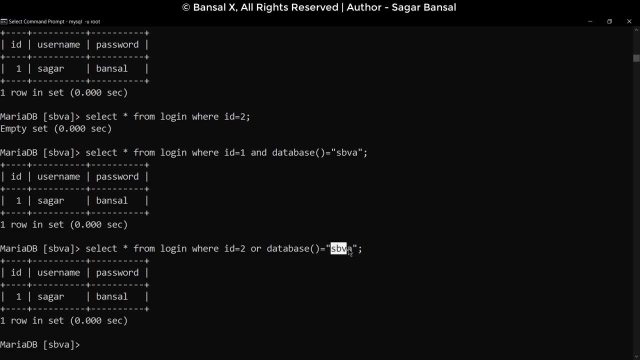 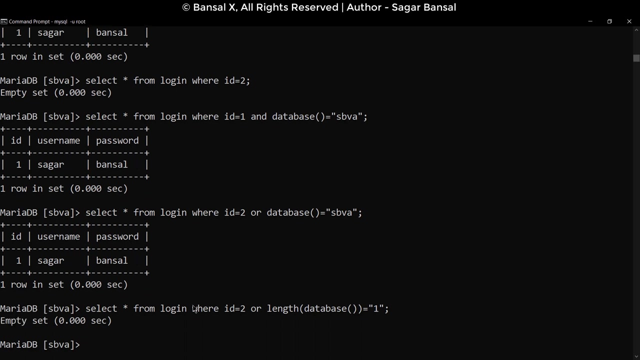 But the question is: how do you get the data? How do you know that the database name is sbva? It's pretty simple. You can use the length function to find the length. first of all, I have a fresh comment So I can say: select stuff from login where id equals 2 or length of the database is equal. 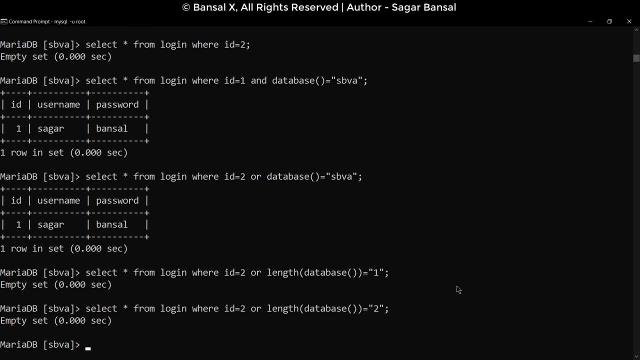 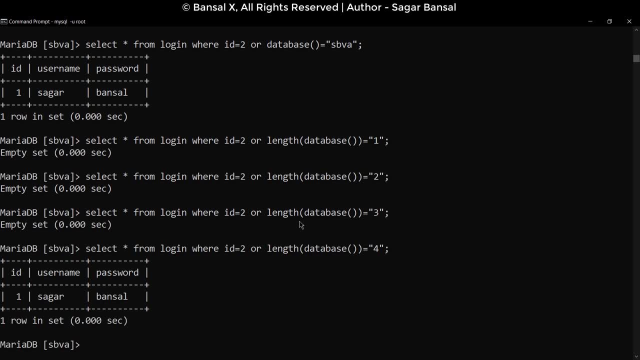 to 1 and it says empty set. I can try 2: it again says empty set. I can try 3: it again says empty set. but when I try 4, it gives me the result. This tells me that the length of the database is 4.. 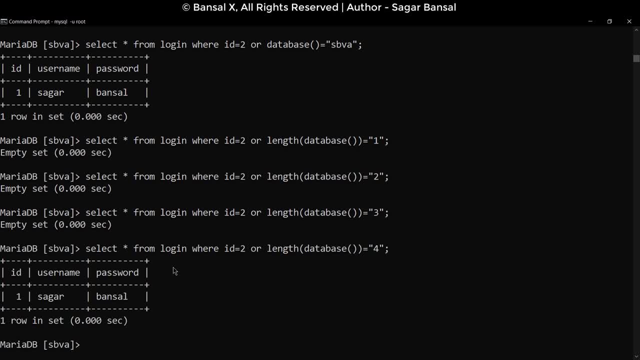 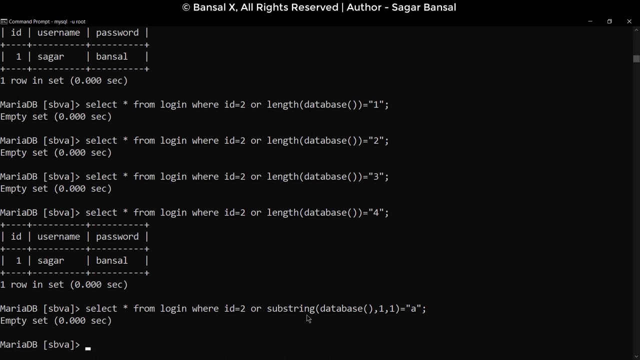 Now we have to see what is the first character in this length. For that we can use substring. We can say select stuff from login where id equals 2 or substring of the database function. check the first character and only check one character and see if it is a. 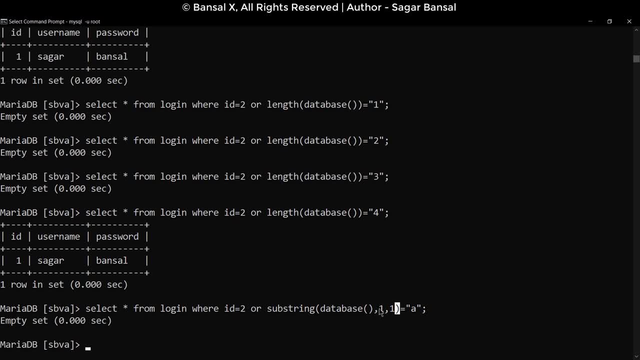 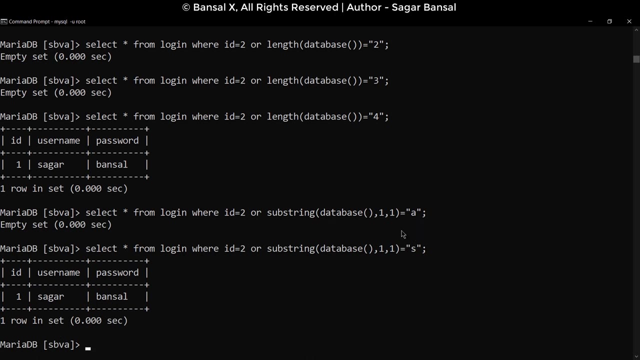 However, If we are checking one character and if we are checking the first character, it is not a, it is s because the database name is sbva. If I check s here, you can see we get the result. So you can brute force from a to z by putting this kind of pattern. 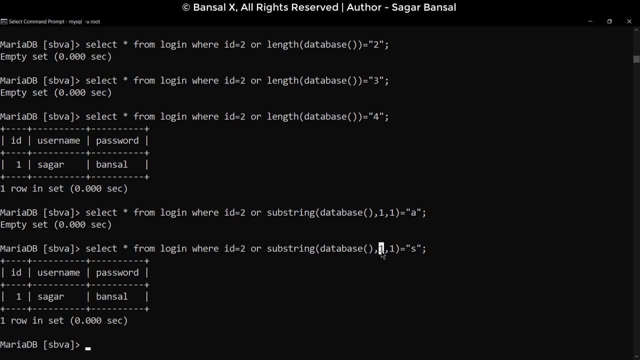 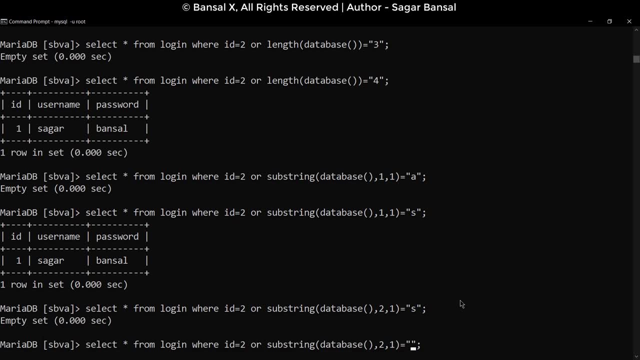 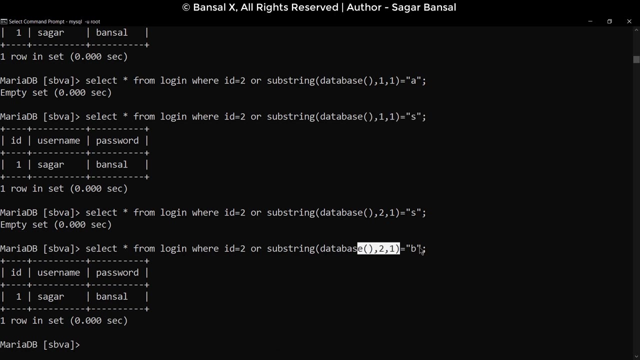 Also, you can check for the second character by replacing the first one. This will not give me any result, But if I change this s to b, this time it gives me the result. So the first character is s and the second character is b. 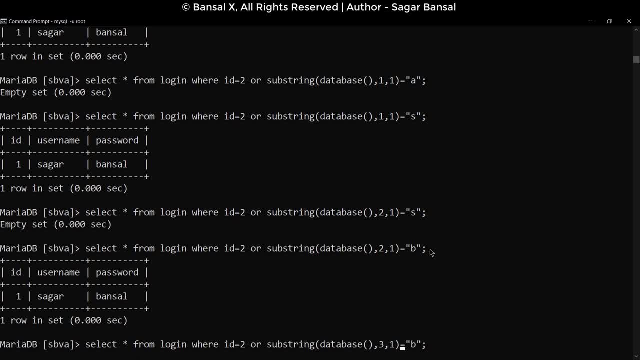 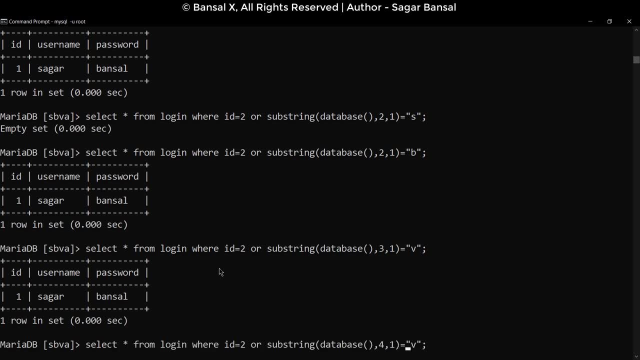 Similarly, I can try for the third character, which is v, and I can try for the fourth character, which will give me a result on a. I can even try combinations. so instead of just one character, I can try two characters at the same time. I am going to try two characters, starting from first, which is s, and b. 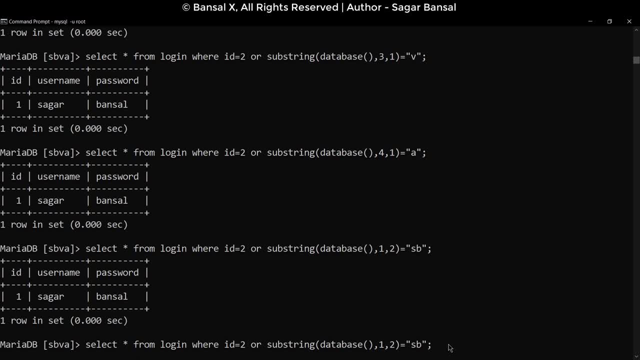 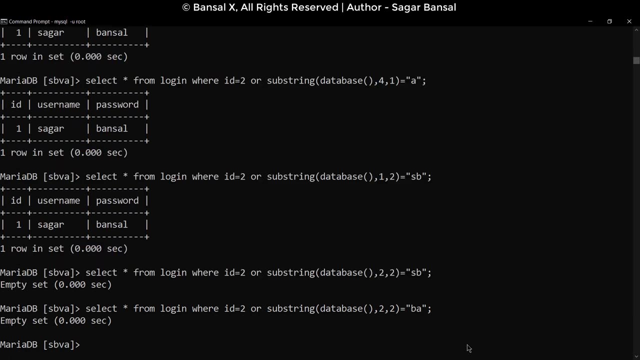 You can see it gives me the result. I can try from second character two characters which should be b and a in sbva. So b and a. If I try sb it won't give me the result, but if I try b and a it will give me the result. 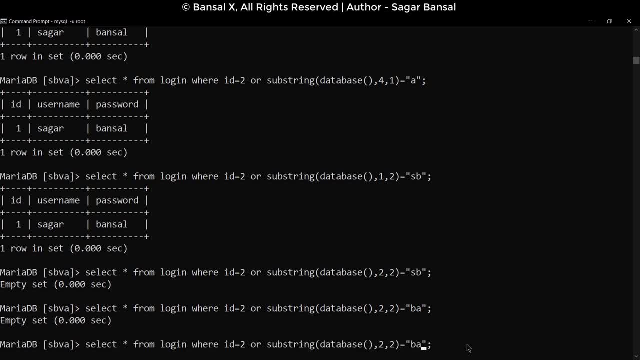 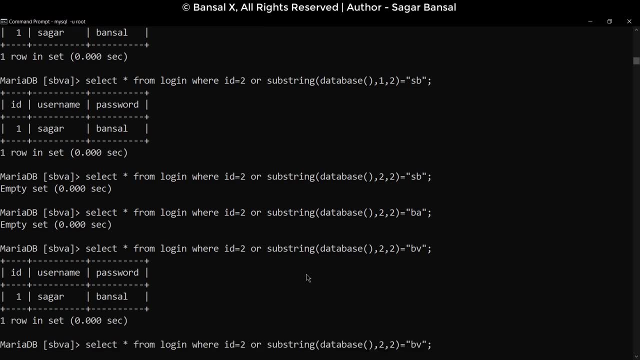 Well, that doesn't matter Because it is sbva, Because it is not ba, it is bv And you can see sbva. I can try the whole database itself by putting one and four, which means start from first character and select four characters in the string which is sbva. 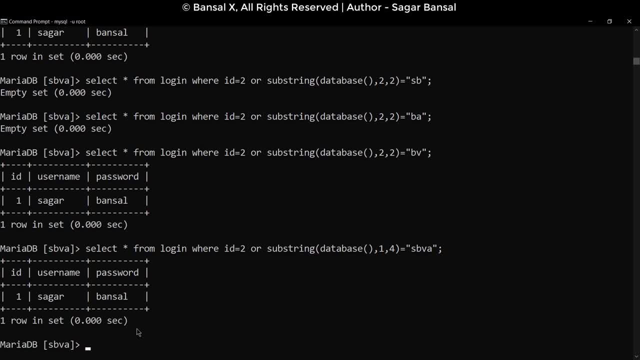 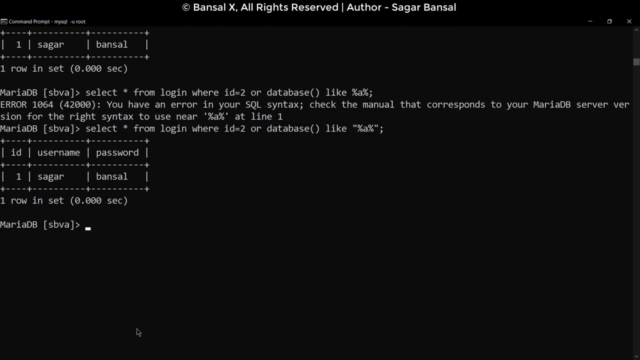 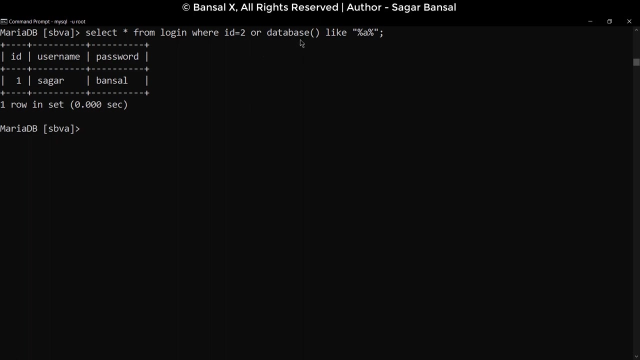 And that gives me the output. I can even use the like function here to speed up the process. You can see, in this command I'm using select stuff from login where id equal to, or I get a status So to, or database like percent, a percent. now what this percent means. it's a wild card, it means 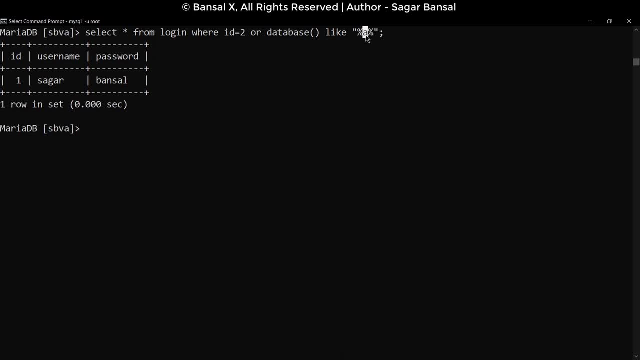 check. if there is a in the database name, it can be at any place. so any places before it, any places after it. you're just checking that. i can say check a, b, that's our reason works. but if i check v a, that gives me the output, because s, b, v a are the last terms. 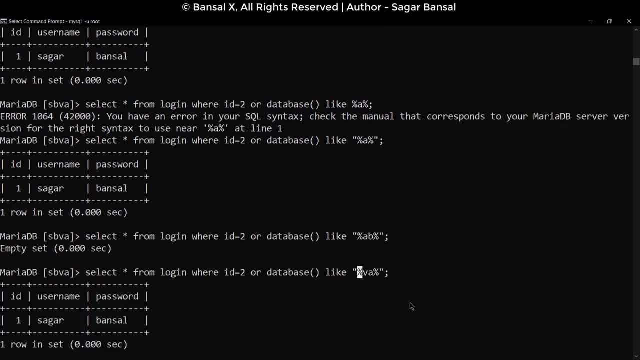 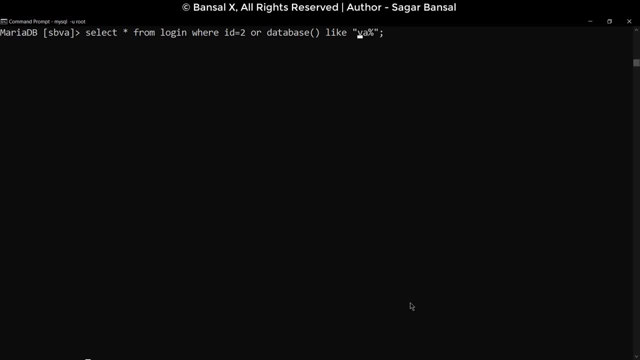 i can remove the first percentage if i need to. we will make it v a, but we will not get any result because we are saying, see, if the database is like v a and then something which is wrong, because the database is like s b, v a, not v a, something it's not v a, n v. 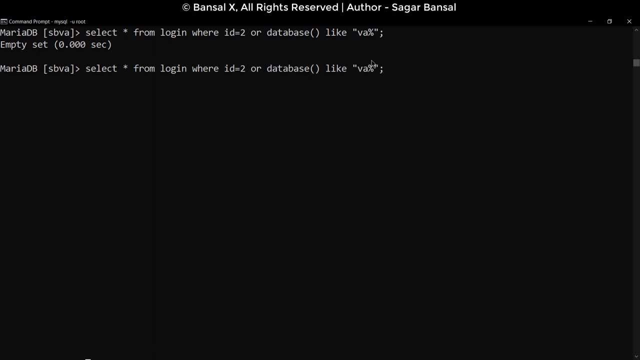 a b, it's s b a instead. i can do is i can replace the last percentage and i can say check if database is like something which ends with v a, and this gives me the result, and that is how you can use the like function to find stuff i can. 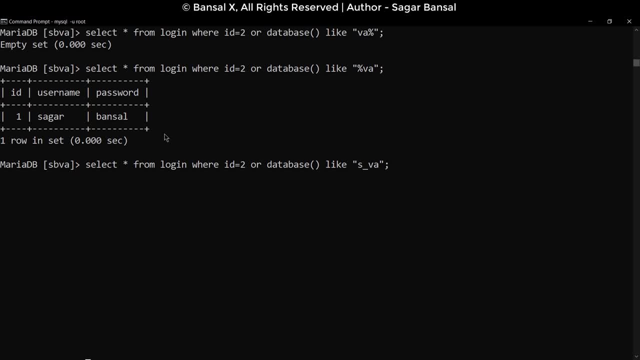 say s underscore va, which means I don't know what will be there in between this, but there is just one character which should give me the result. Or I can just put a percentage when I don't know the number of characters which should again give me the result. 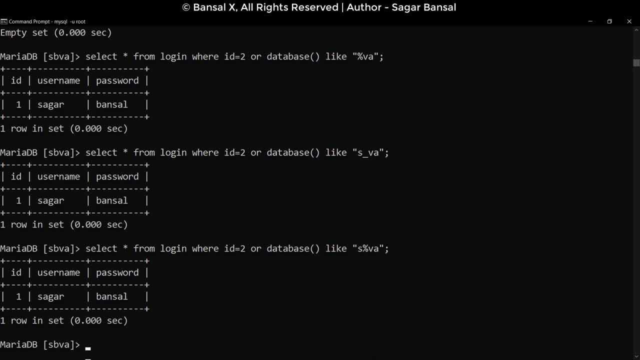 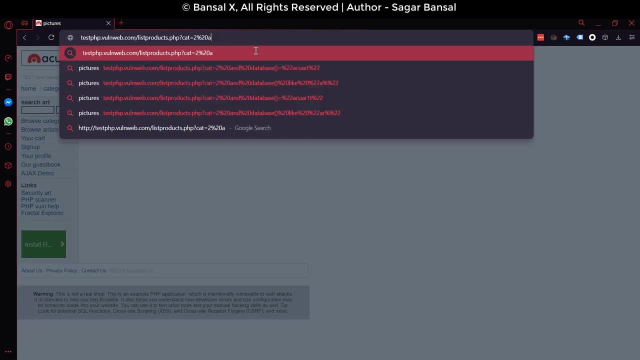 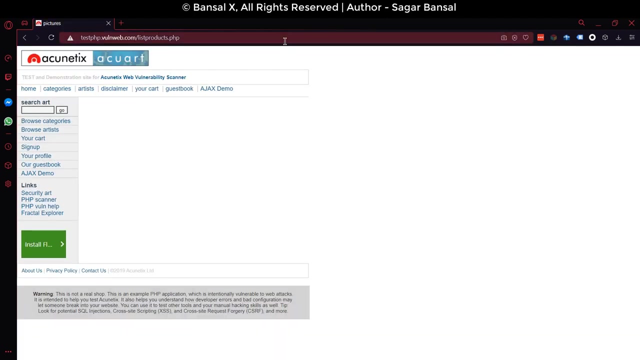 It's all about pattern matching. Let's try to do the same thing on the website. So cat equals two and because we know that cat statement is true, The length of the database is one, which is not true, and we don't get any. 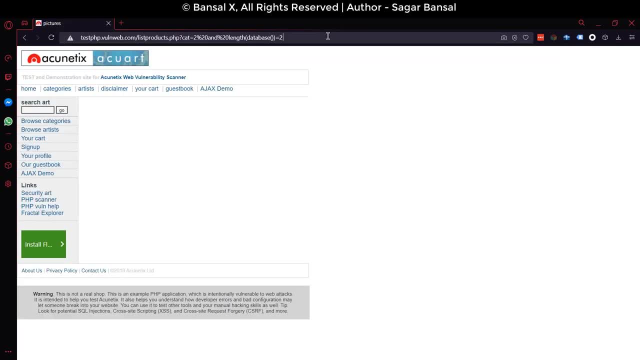 output. Length of database is two doesn't work. Length is four doesn't work. Length is six certainly works, because the database name is ACUART, which is six characters, and in this way you can go ahead and try a lot of combinations and try to extract data bit by bit using boolean. 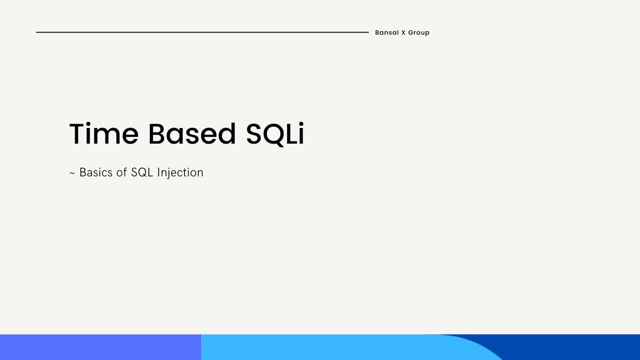 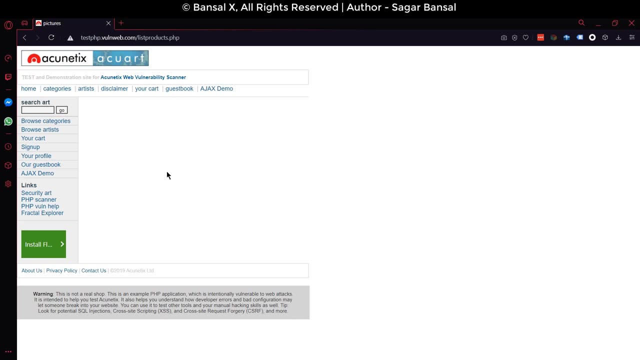 based SQL injections: Time based SQL injections. well, there will be certain cases where you will not be able to see any output on the screen. It will be the screen, which is same in case of a valid statement or an invalid statement. In certain cases. instead of looking at the output, we can look. 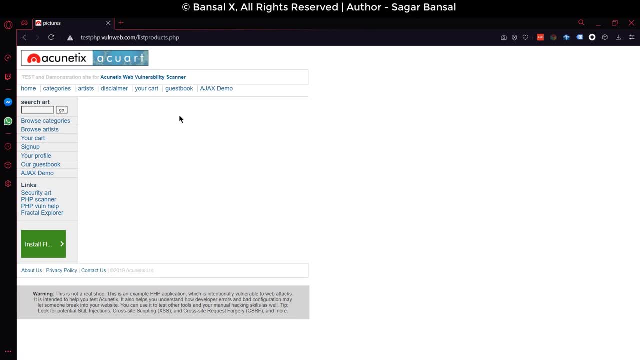 at the time which the server takes to process the request or to send the response. In the following case, I am trying to ask the server that check if the database name is ACUART, If it is then sleep for 10 seconds. So if I press enter I can see that the server is not able to see any output on the 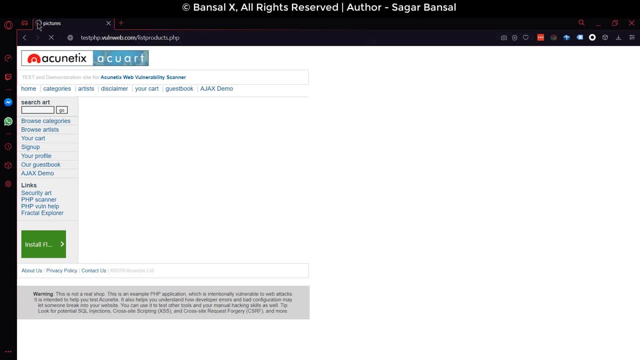 screen. If I press enter I don't get anything on my screen, but you can see the server is taking 10 seconds to give me the response. It's sleeping right now and after 10 seconds it will send some response to me which is again the same page. So on my response nothing changes, but it took complete. 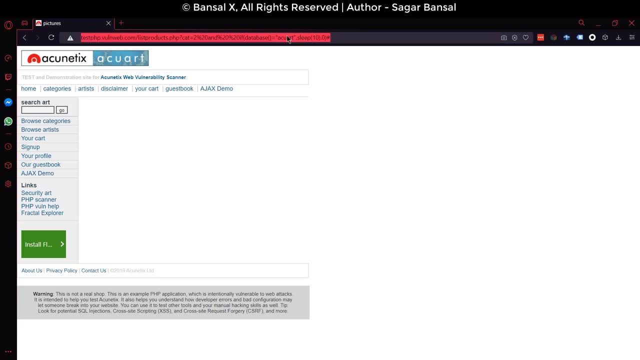 10 seconds to show me the page. Instead, if I just put some random name here, it will not take more than two seconds to give me the response. That's it Now. if I press enter, I can see that the server is taking 10 seconds to send a response. That is where I can justify if the statement is true or 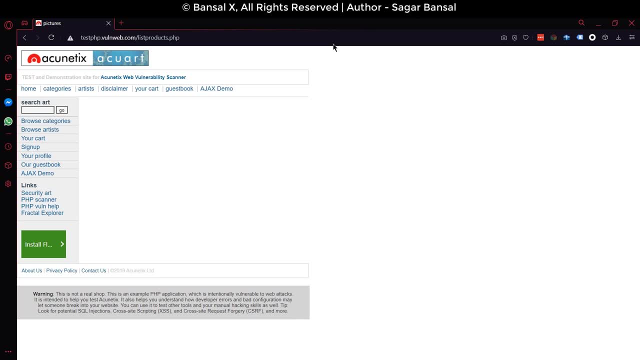 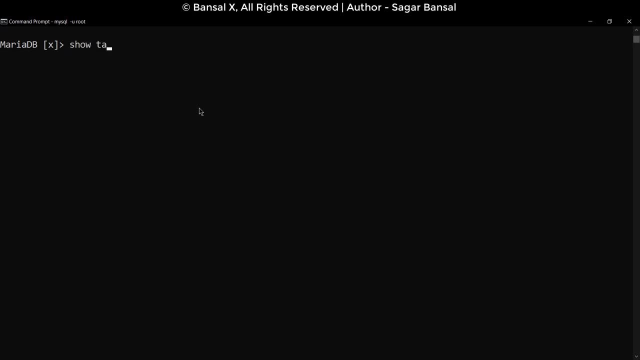 false just by looking at how much time the server is taking to give me the result. Just to make it simpler for you, I am going to show you a few examples. There is a table called users and you can see in this table there are three users: Sagar, Alice and Bob. However, let us assume that we do not have the ability. 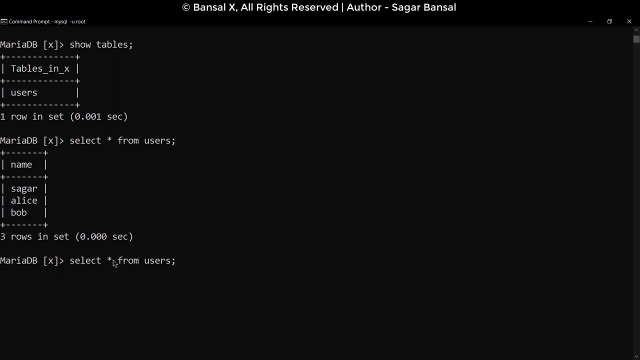 to play with these users. every time, the output is just these three users. What can we do in such case? We can use sleep statement by combining it with AND, Select star from users and IF, And here you will put your sleep statements. However, please note, this depends on product. 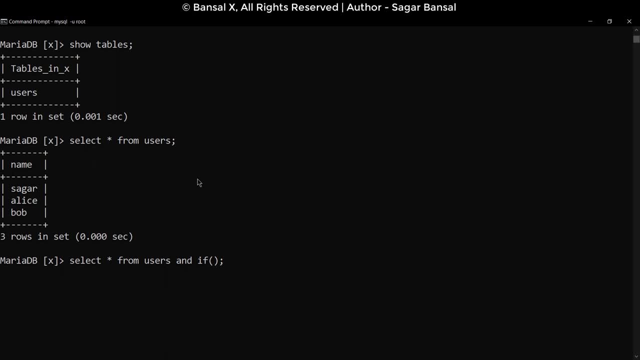 to product. In case of this database, which is a MariaDB implementation of MySQL, the function works in condition true- false, Which means you put your condition. If the condition is true, then this will happen. If condition is false, sleep is true. sleep is true. If condition is true, sleep is true. 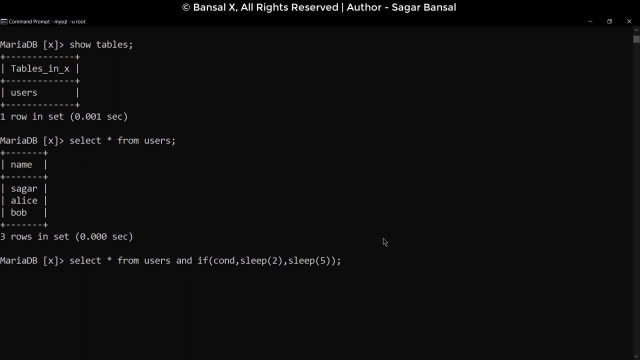 sleep is true And the condition is: database equals a. If I try to run this, it throws an error And the error occurs because there is no logical condition and the user has not. should answer previously in this, you see, to use time-based injections, you need a logical condition. 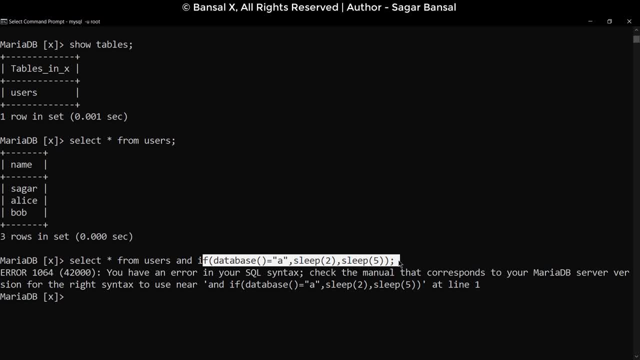 like where, which you cannot control. so if the application, instead of this, is using where name equals saga, now the application is checking for a logic select star from users, very, name equals saga. this is something which the application is checking, it's a logic condition, and then we are putting and: 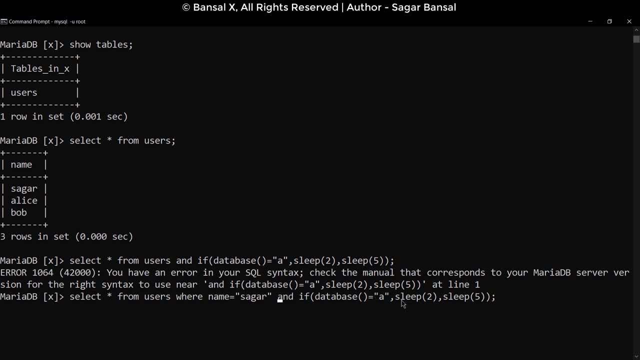 also check if database equals a, then sleep for two seconds or five seconds. this will work and you can see the database is sleeping, but how much- two or five? you can see. it's slept for five seconds, which means database name is not a, because it is X. so can I show you with the X, of course. 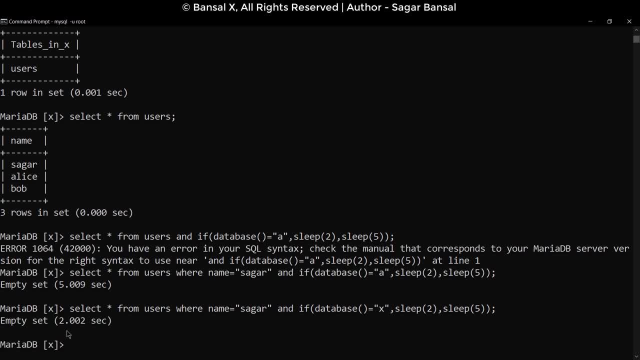 you and I do it with the correct database name. it sleeps only for 2.002 seconds. two seconds because of the sleep function: 0 0, 2 seconds to process the request. again five seconds because of the sleep function: 0.009 seconds to. 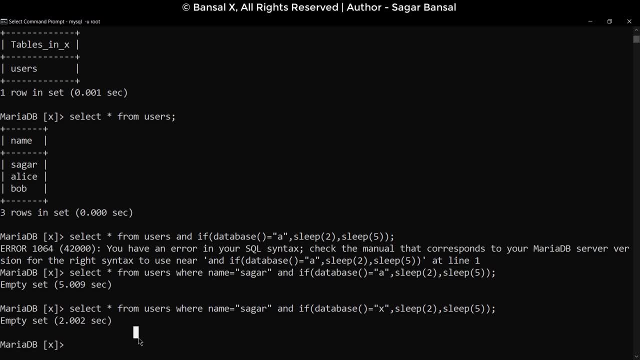 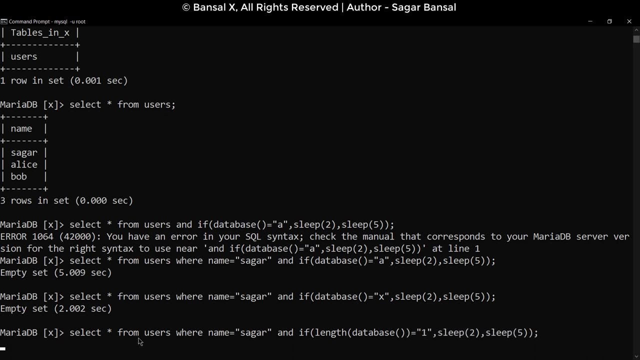 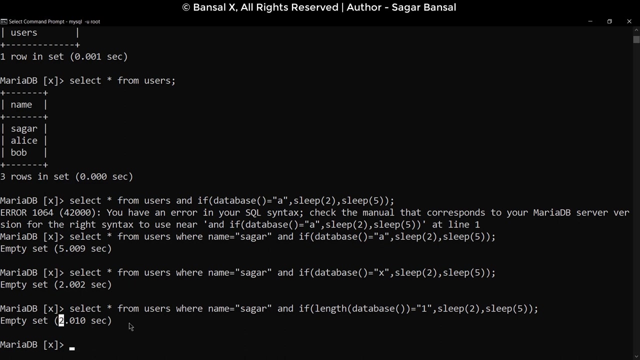 process the request. similarly, we can use different patterns like length, and now we are comparing if the length of the database is one or not, and in this case the length is 1. if we see if the length is 2 or not, it'll say no because 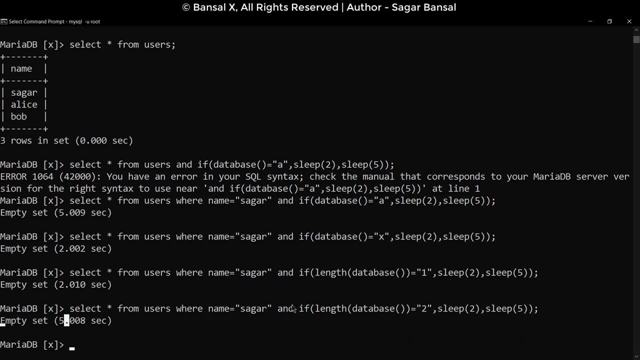 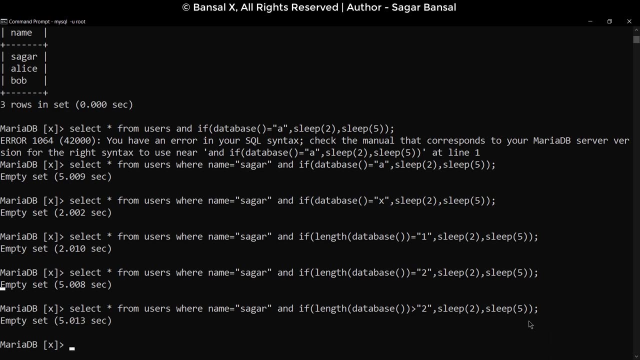 it'll sleep for five seconds, giving me the confirmation that the length is not equal to 2. I can even use a greater than sign here. so if length is greater than 2, then sleep for two seconds. if not, then sleep for five seconds. as you can see, 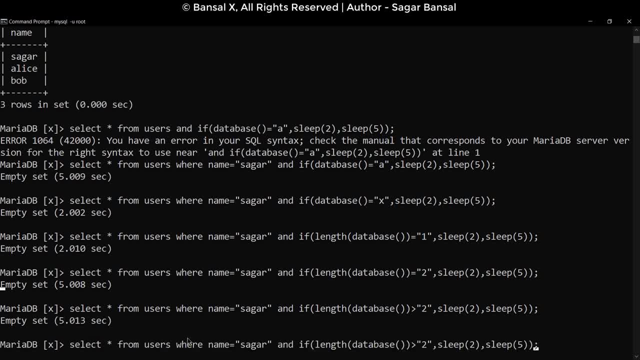 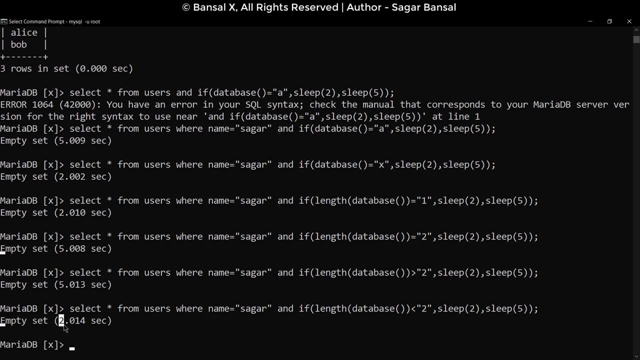 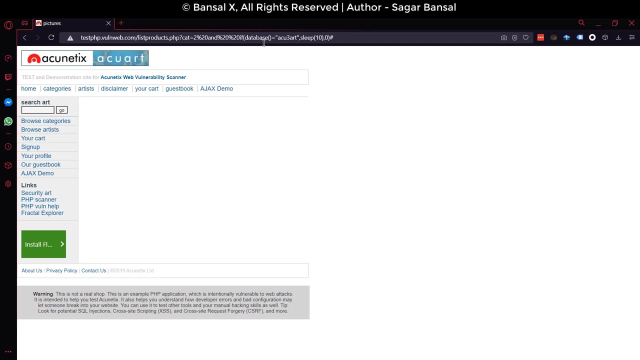 length is not greater than two, it is less than two. so I can say length is less than two and this will sleep only for two seconds, as you can see. so by such techniques you can analyze the time of the database and conclude if a situation is true or false. I can even do length calculation here. 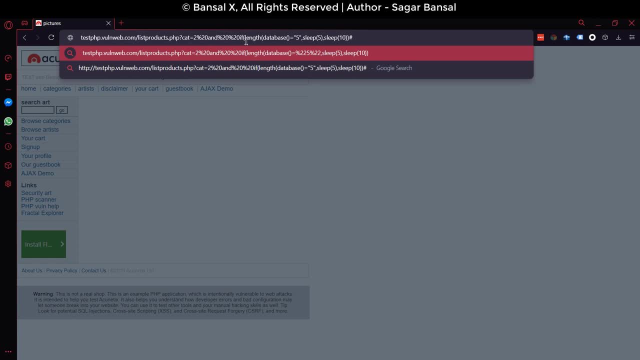 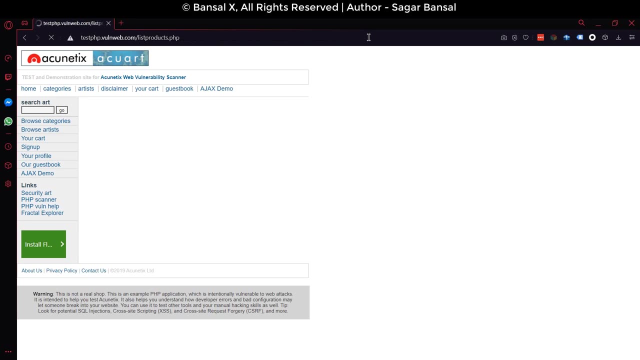 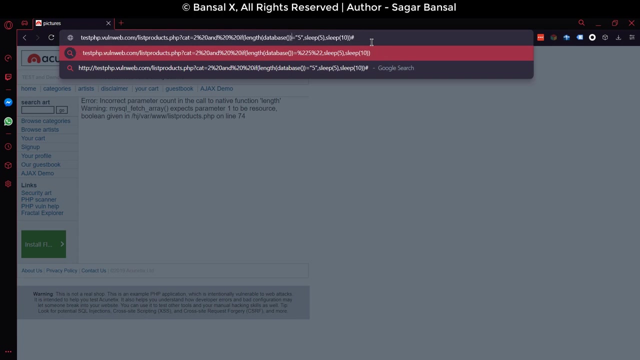 so in this following example, I am checking: if the length of the database equals five, then sleep for five seconds. otherwise sleep for ten seconds, one, two and it throws an error. let's see what the error is: length. okay, did we did some mistake? yes, we forgot to close the length function, so let's close it and let's try. 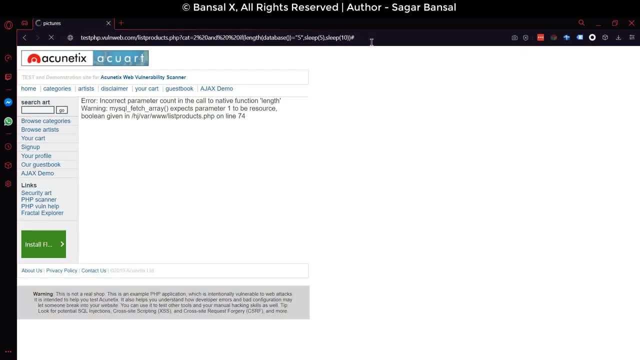 now one, two, three, four, five, six, seven, 8, 9, 10, 11, 12, 13, 14, and maybe i'm counting too fast and it just comes up with the result and you know i can conclude that that was definitely not five seconds. however, if i try it with a number, 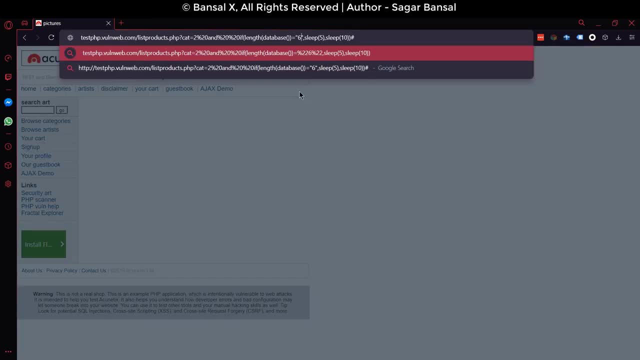 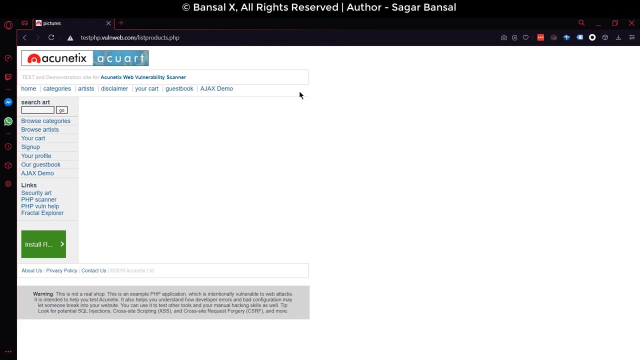 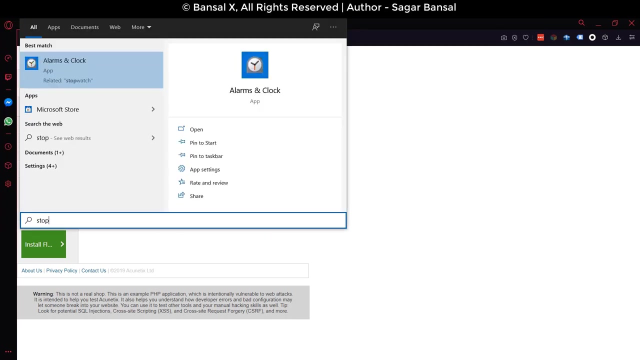 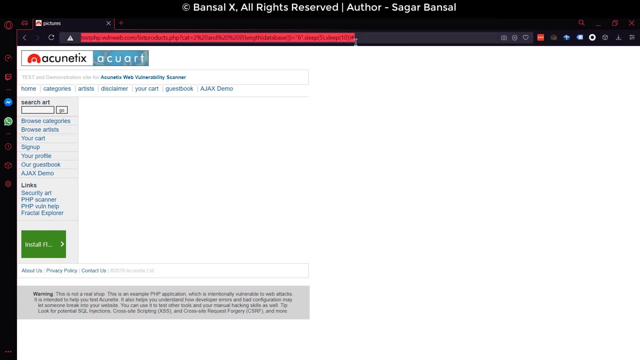 of six, which is actually the length: a, c, u, a, r, t. one, two, three, four, five. so do we get the output? yes, we get the output. right, that is kind of how it works. let me go ahead and start a stop watch instead. this should be easy. so i'm going to say: 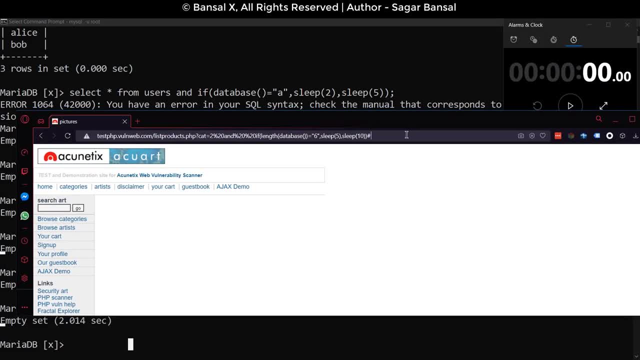 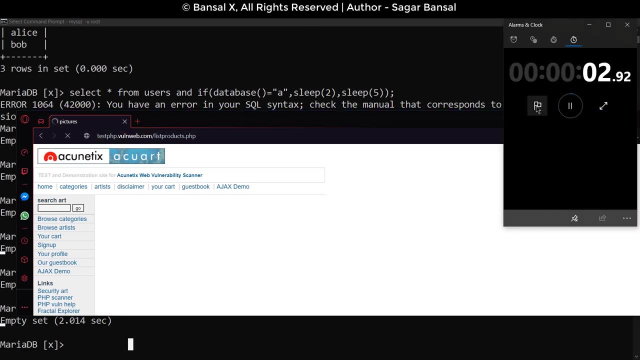 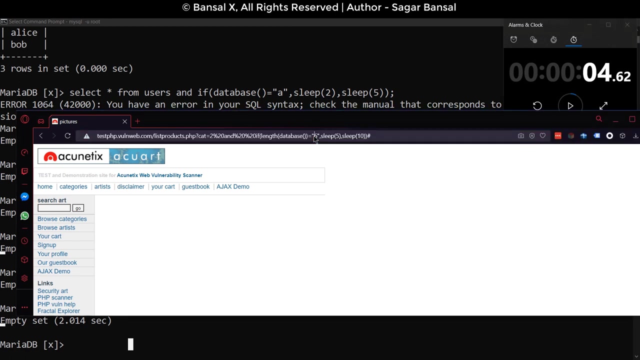 and do we get the result here? here we go. we got the result in almost four seconds, but still, because i started it and it took one second to. you know, come from browser to stopwatch. it took one second over there if i do a wrong statement, like five. 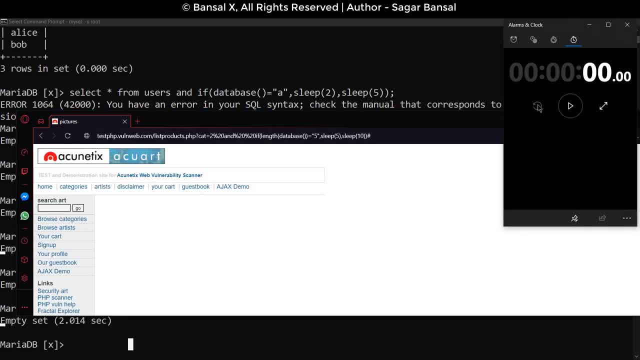 and if i reset that and if i press enter, then let's see. so we got, we got. we got the output in 11.51 seconds and assume it was taking somewhere 12 seconds, because i came from the browser to here this was one more second. so roughly 12 seconds instead of 10. so that is the. 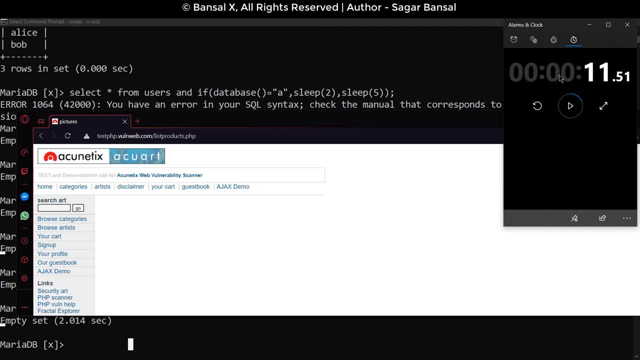 processing time it is taking, but it is definitely clear that if the request is true, it comes somewhere around five. if the request is wrong, it comes somewhere around 10, because i am giving that in my assumptions right. that is how you get to know if it's true or not and if it's not. 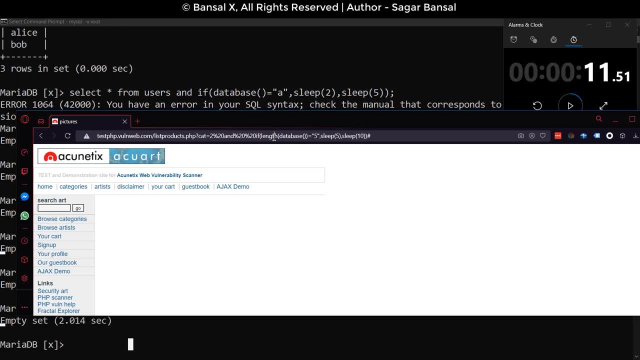 if it is true or if it is false. and just like you use the length function, you can use the substring function to calculate the name of the database or to get any kind of information from this database. it all depends on how well you understand sql, but that is how the time-based sql injections work. 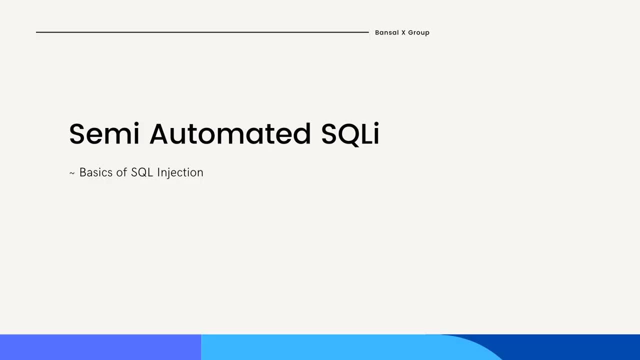 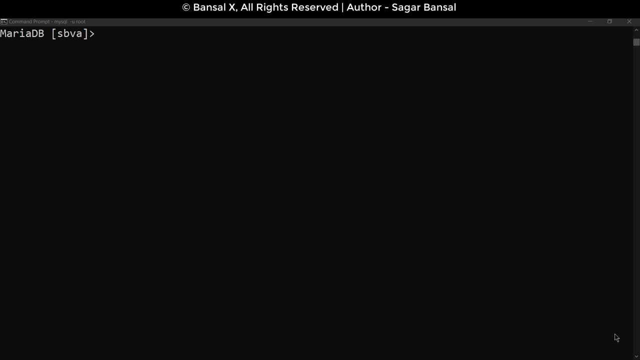 using semi-automated tools for sql injection. well, there will be certain situations which will be humanly impossible for you to test thousands and thousands of payloads with. think about a login page. if you're bypassing a login page and they have used certain filters, it will not be easy for you to try all the possible combinations. 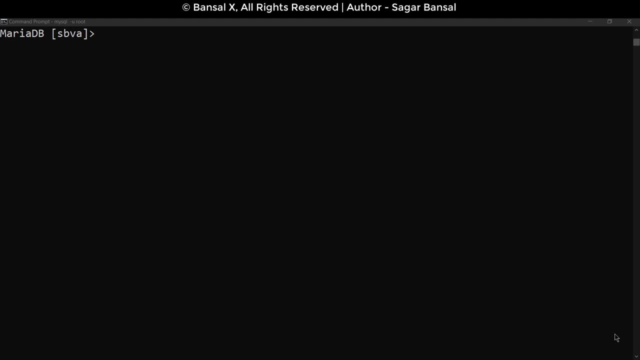 that is where semi-automated tools come into the picture again. remember, these are just semi-automated, they are not fully automated. you still need to understand why sql injection occurs, where do they occur, how do they occur and what is the reasoning behind everything, and accordingly, you can use them to automate the heavy lifting. 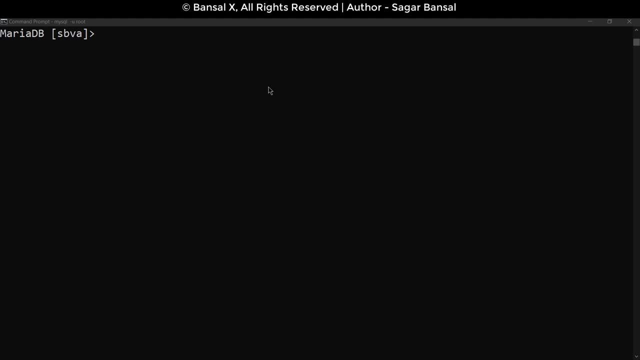 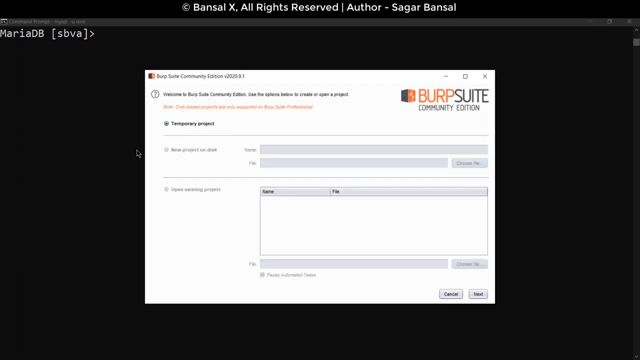 one of the tools which i personally like is called burp suite. there are alternatives like os zap. however, burp suite is a good and reputed tool. you can download it from portswiggernet. just download the community edition and install it. it's available for all the operating systems. 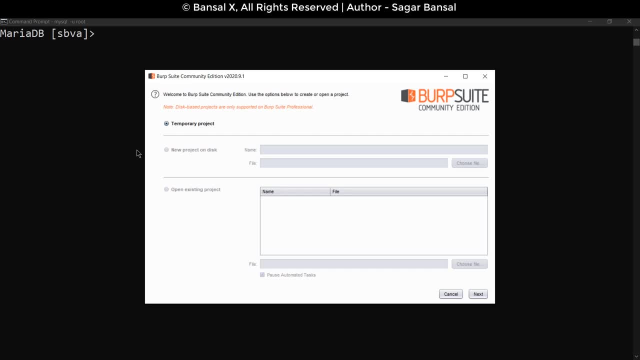 it's a simple next, next, next install, so i will not cover that part. in community edition you cannot save the data, so you always have to start a temporary project. that's fine with us. you can start with the default of verbs. that's also okay, just start it. 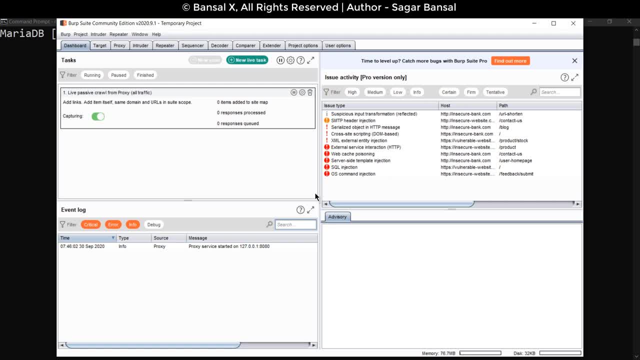 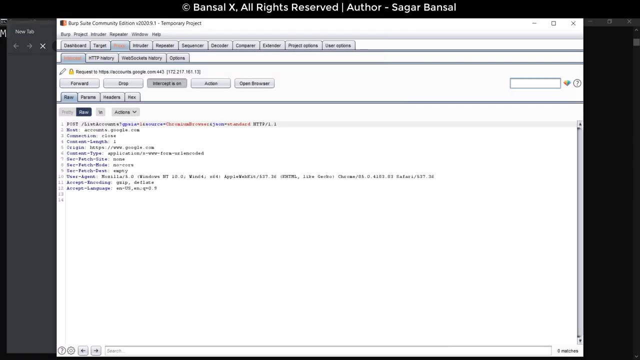 and now burp has started. now there are many ways to use it. everyone has a preference. however, in these new versions they have started to make a built-in browser. if you go to this proxy, you'll see here open browser. this is a chromium browser and it's a specially configured one because it works. 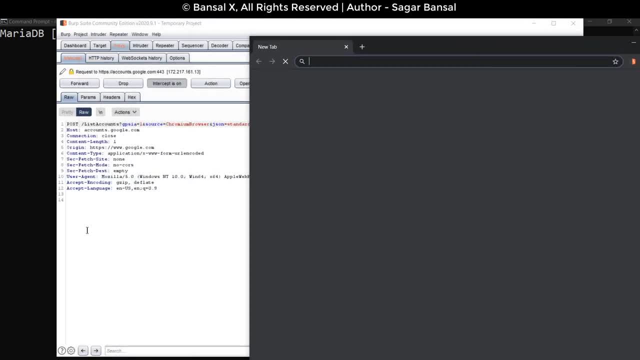 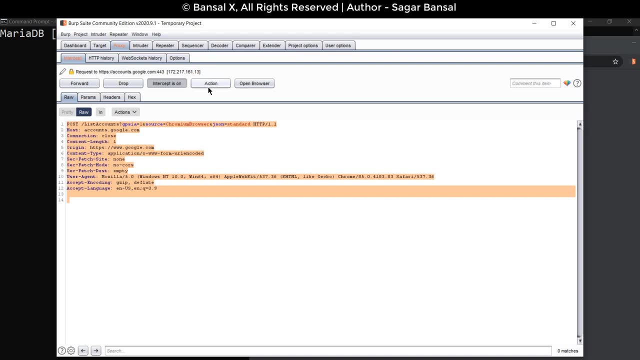 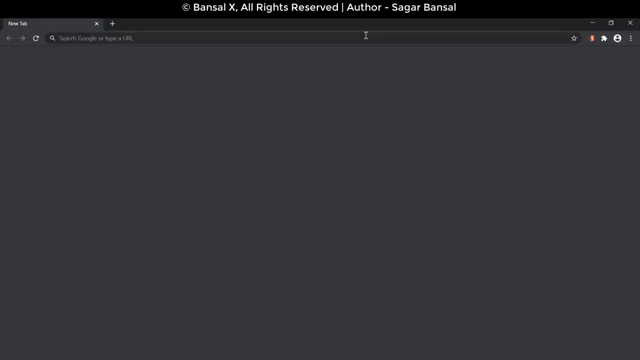 with burp suite out of the box. now here, just make sure you do turn off this intercept because you can see it automatically starts capturing a lot of requests and we don't really need this. just turn this off now. go to your browser and open whatever you want to open. so i'll open my target. 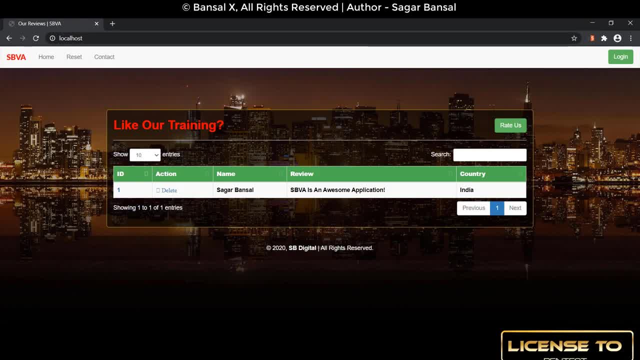 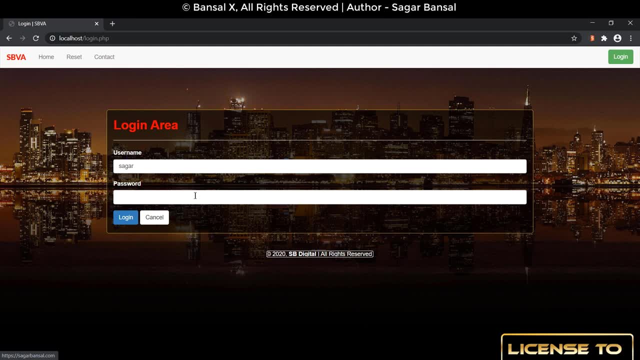 which is localhost, and here I'll go to login and here I'll put certain username and password, like Sagar as username and mypass as password. now you see, it doesn't really work. of course, the password was wrong, so we were not able to login. that is fine. we can go to burp and 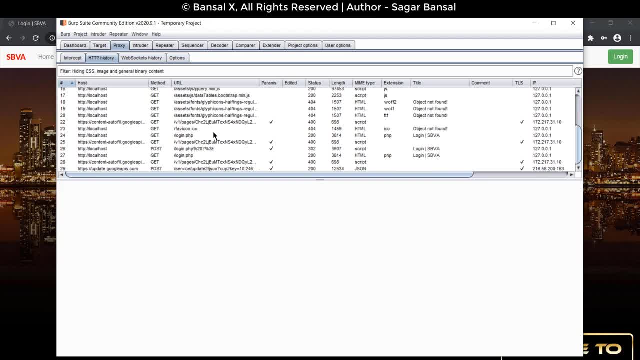 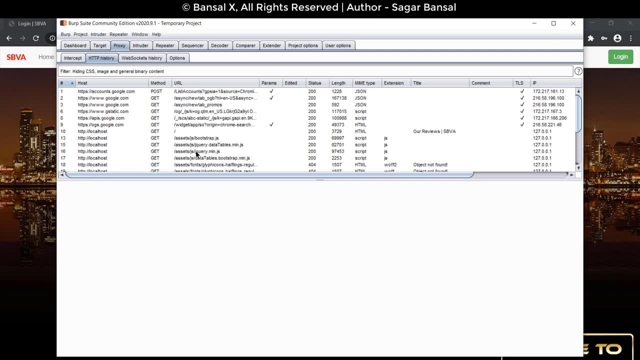 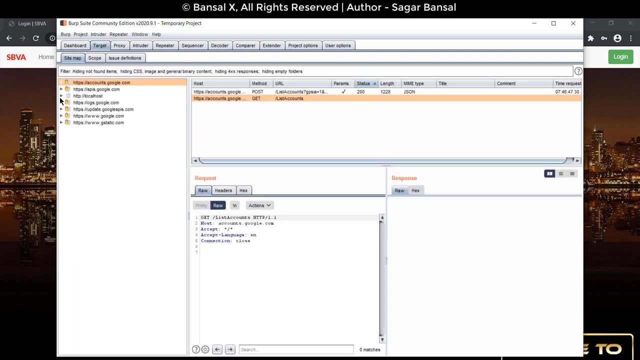 if you go to http history you will see all the requests that have passed through burp. using this specific browser it may be hard to find that request in these much requests, so you can go to the target tab and it's the graphical tree view. we are using a localhost. 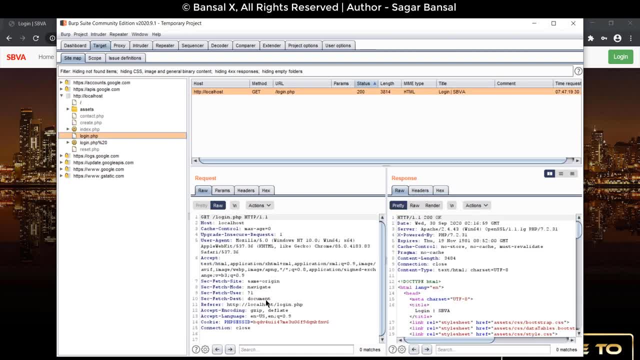 and we are using loginphp. it is interesting that this is not the right request. however, there is one more loginphp which has certain percent- 20 in that, but this is the right request. you can see: username equals Sagarphp, password equals mypass. this is what I typed, so this is our request. again, there are two. 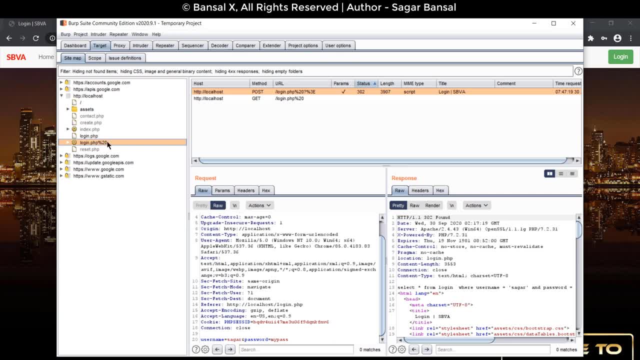 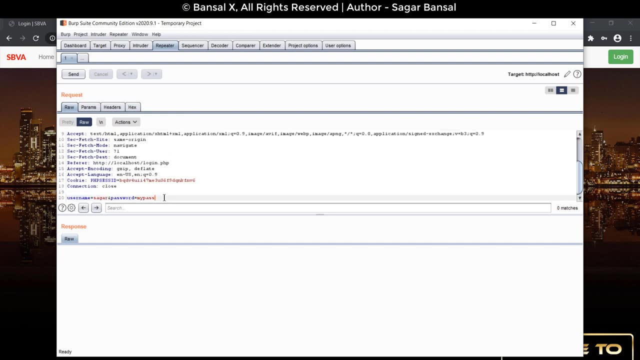 requests: loginphp- loginphp- percent 20- something that is fine with us. we can send this request to repeater. now you can see the repeater highlights and now you can do whatever you want with this request and send it from here and the response will come over in this window. so 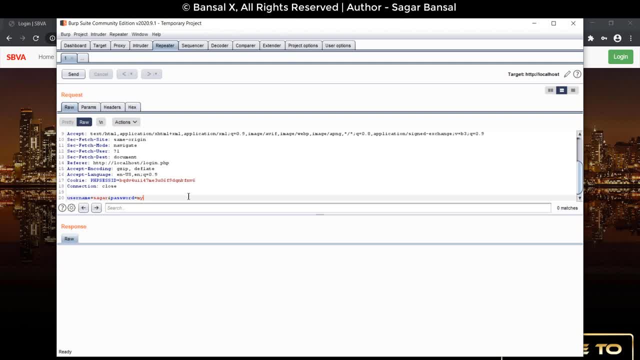 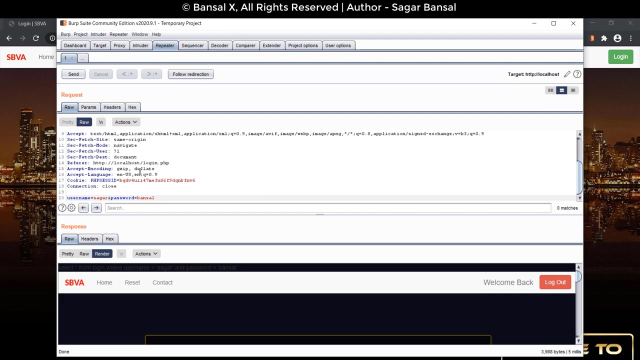 first of all, let me try, instead of mypass, let me try the right password, which is bunso. let's try to send it now. let's click on render to see how it works in the browser and we were able to login. as you can see, login if I use a wrong password. 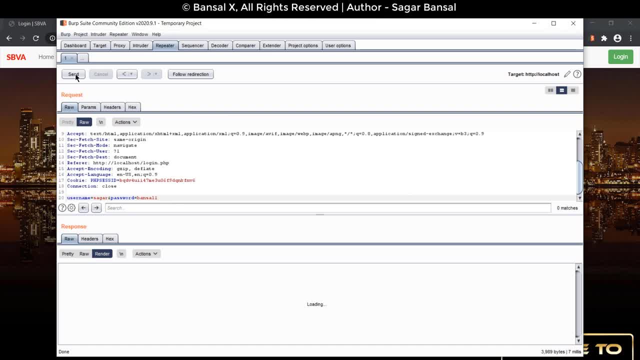 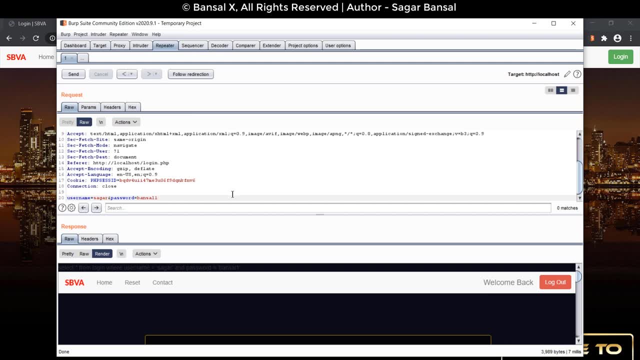 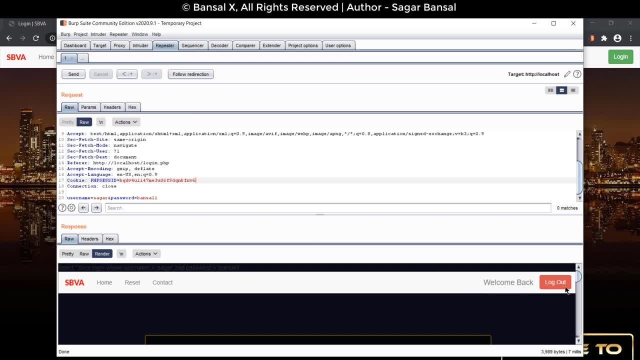 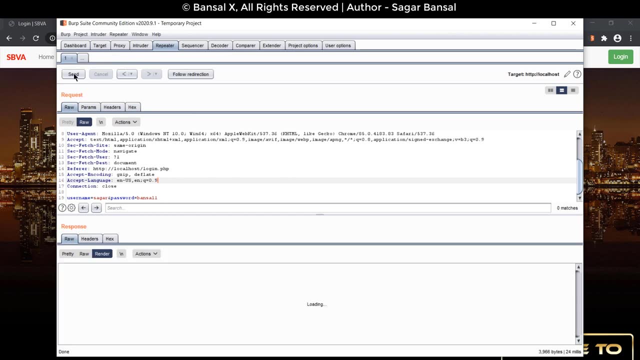 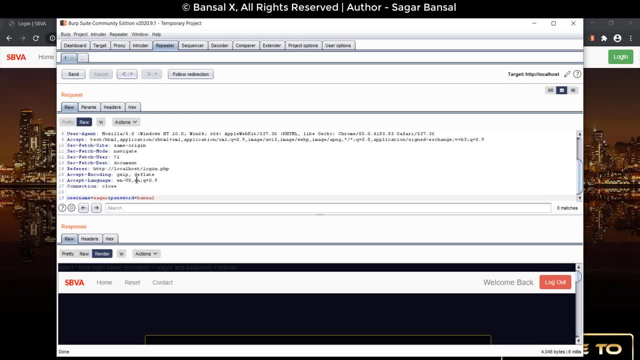 I press send, I am logged in. if I again type the wrong password, I am not logged in. Though the request is working fine, however, I would suggest that you remove these additional characters from it. It doesn't really matter and it won't affect your testing, but the file name is loginphp. 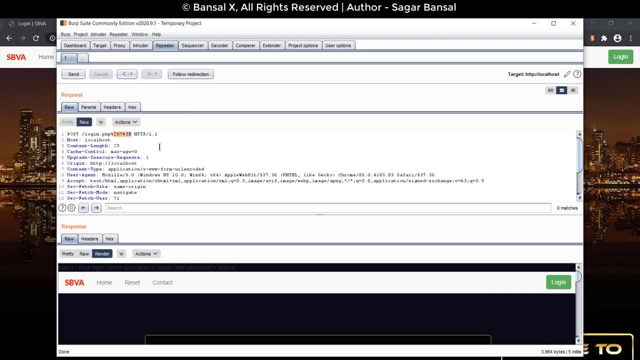 not loginphp and these characters. So due to some processing, it certainly picks up these characters in the request. That is fine. you can safely remove them. and now this is a perfect post request going to loginphp using HTTP 1.1.. 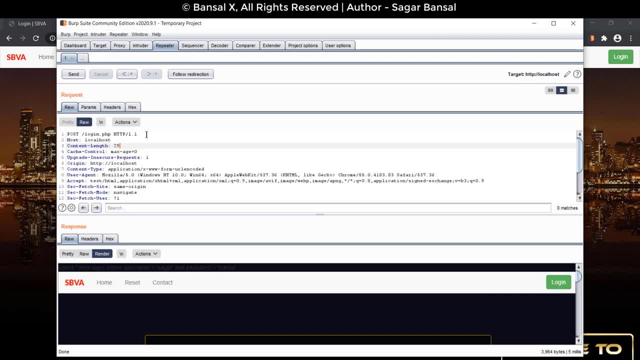 Again, if you didn't do this, if you didn't remove that, still the request is working fine and you can use it. But I like to be a professional. Now we know that this request is working, so, instead of using the right password and 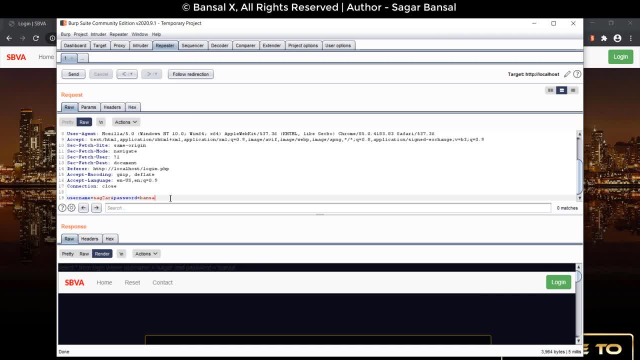 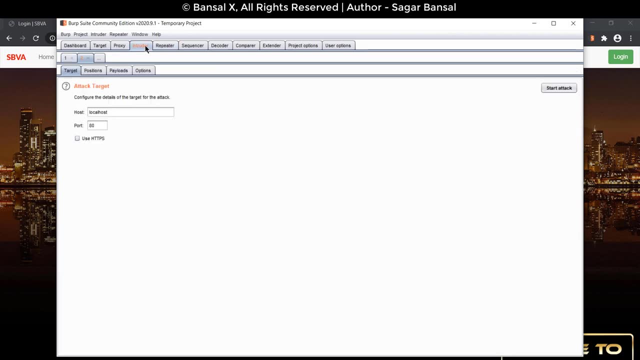 username. I am just going to give an invalid username and an invalid password Again. let's send it once more to confirm it's working. fine, Now we can send this thing to intruder, so send to intruder. You see, the intruder tab highlights. I'll go here and it tells me what are you attacking. 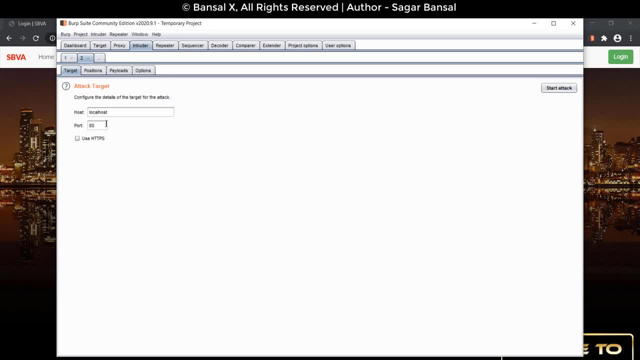 I am attacking localhost. That's correct On port 80.. That's correct Because I'm not using HTTPS. If I'm using HTTPS, then I have to put port 443 here, or some other port, depending on the configurations. But since I'm using HTTP, so I'll make sure this is unticked here. 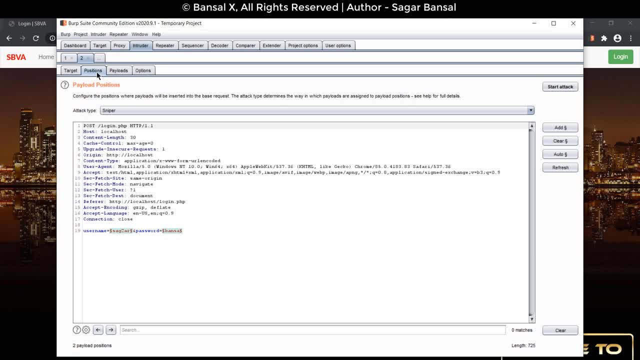 Now let's go to positions. and the great thing about burp is it automatically positions everything. You see, these things are marked in green and they have been positioned automatically. That's the auto mode of burp suite. You see the auto here. 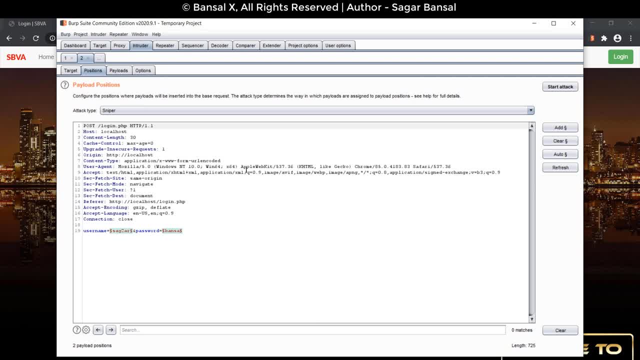 However, in certain cases you may want to add something Like: if I want to add a position myself where I want to do SQL injection, I may want to go ahead and select this and I'll say add here And now. this is also marked as a position. 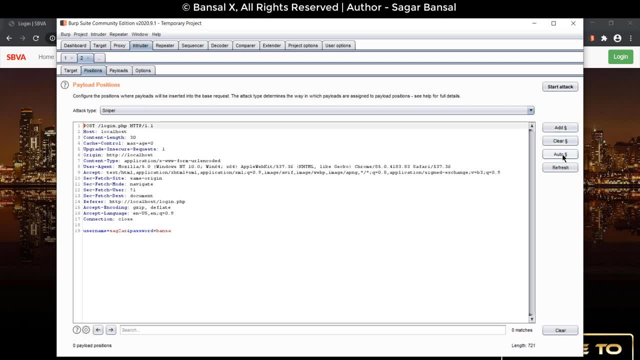 I can clear all of these by pressing the clear button and I can again just say auto to automatically select the right positions, which burp suite does very well. There are four modes: Sniper, battery, ram, pitchfork and cluster bomb. All of them have different purposes. 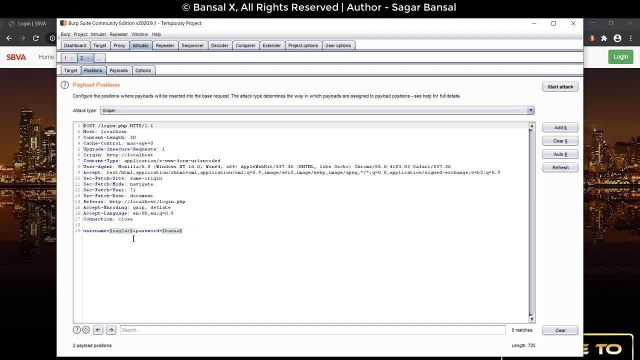 Sniper for instead will try two payloads. right, It's trying payload number one here, which will be my SQL injection code here and then my code over here. But Sniper will do that one by one. So, for example, it will try my SQL injection here and keep the password as B-A-N-S-A- whatever. 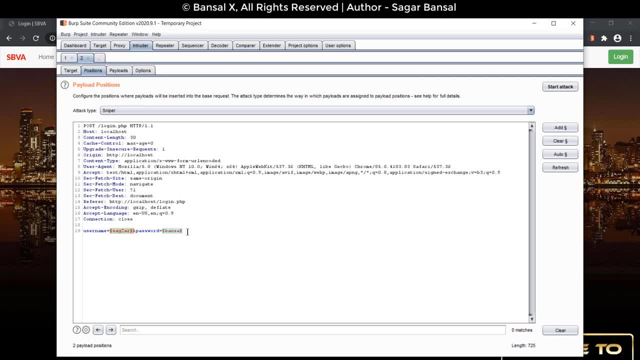 we have given In the input in the request. So it will only change one payload at a time. Then, once that works, it will keep this as it is and it will change the password which is the payload two. So it will change payload one, keep the second as it is. then it will keep the first as it. 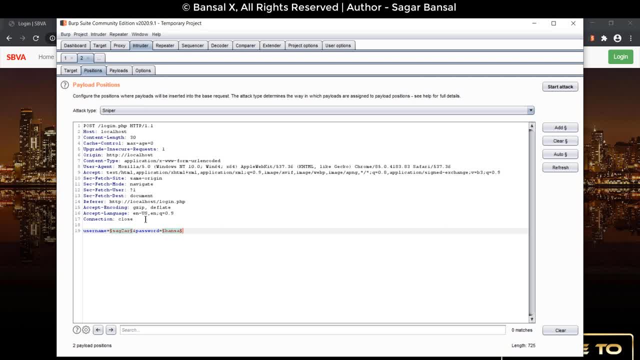 is, and change the payload two. So it's one by one. That is what Sniper is. Again, all of these four have different purposes. Battery ram uses both of them together. So if I use battery ram, It will change both of the payloads at the same time. 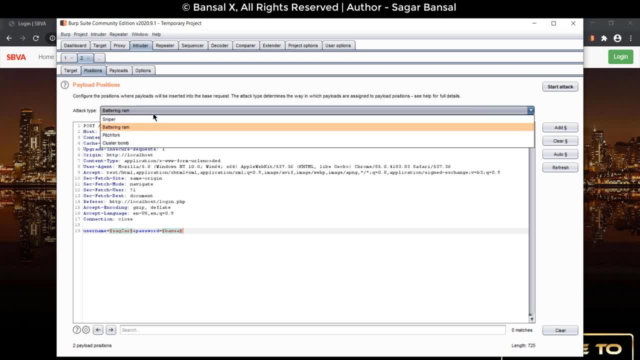 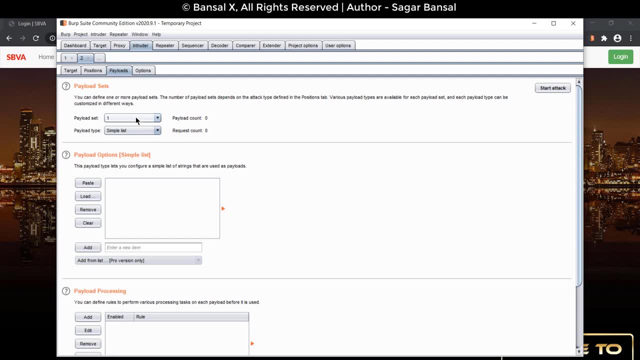 You can study more about this on Port Swigger website. It's irrelevant for this lesson. I'll just go with Sniper. In payloads, you can select the position. Since Sniper uses just one position, you can use one And there are single list and other stuff here. 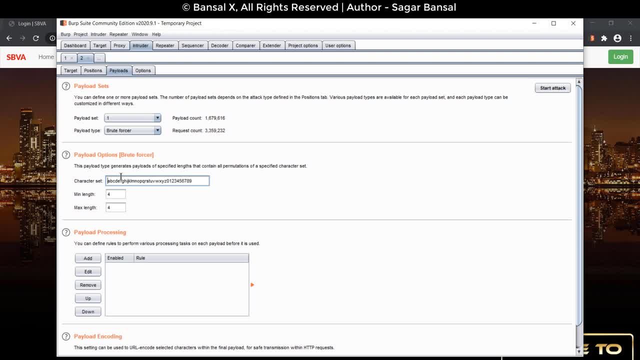 One of them is bruteforcer, where you can specify a bruteforcing combination. We can specify a character list, minimum length and maximum length, Okay, But we are not bruteforcing a password. right, Technically we are, but not through a bruteforcer. 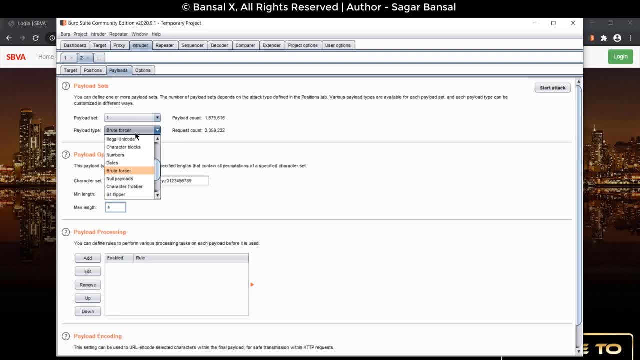 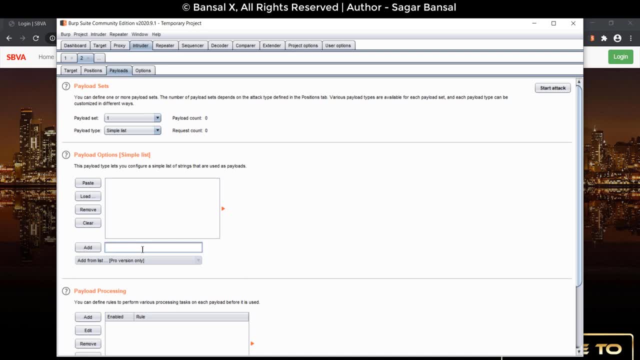 We are doing it through SQL injections. So instead let's go with a simple list and you can load a list of test cases, or you can add a list here. Now I already have a list, so I'll click on load and then load my payloads. 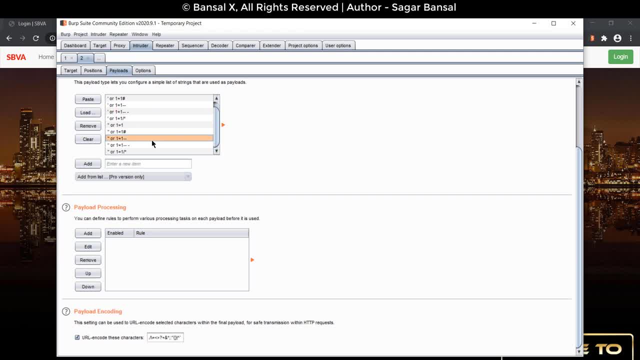 And you see we have certain payloads in this list. You can create your own, So it's just a TXT file, or you can just go ahead and add something like here. I can just click on add and that'll add it to the list. but I'll just stick with my list. 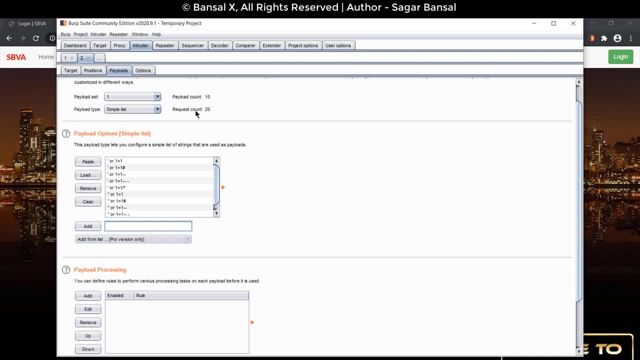 which I just loaded. Now there are 10 payloads in my list And since Sniper uses one payload at a time for both of the positions, there will be 20 requests, and 21 to be precise, because it will even generate a baseline request, which 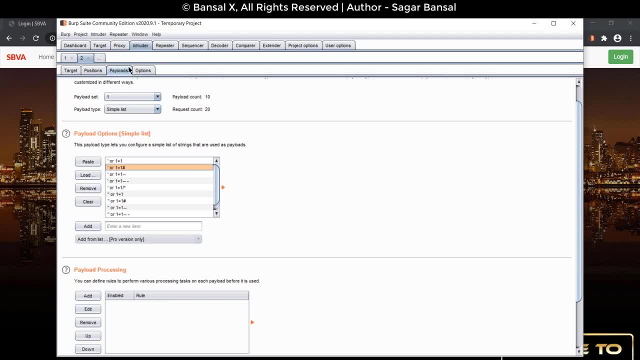 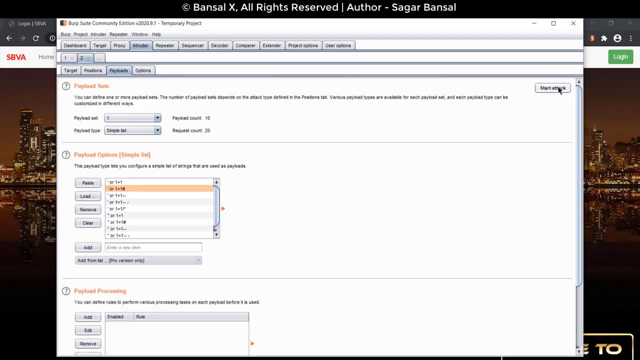 will be using both of the parameters that we provide. Okay, So it'll just go ahead and send this request as it has. That'll be the baseline request. You can go ahead and click on start attack and it gives you the warning. 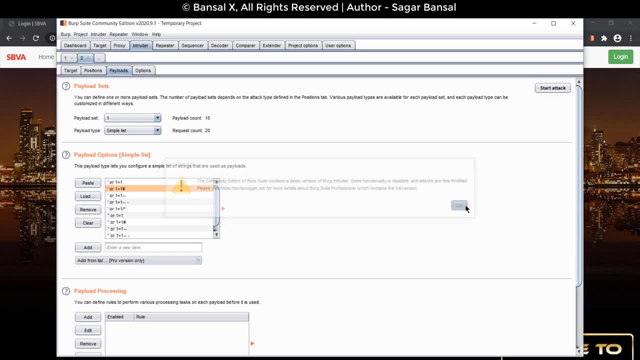 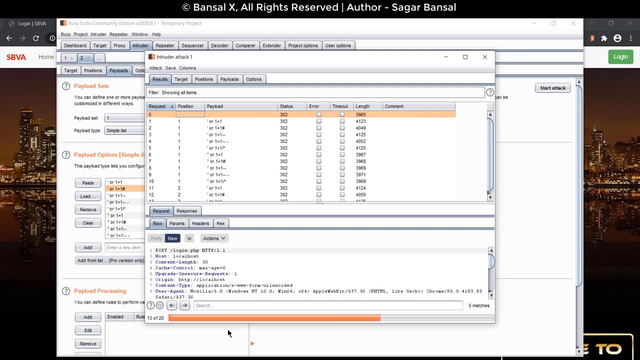 It's the free version, the community one. It'll be slow, That's fine. We just have 21 requests Now you can see. the first one is always the baseline request. There is no position used, It's like the blank request. 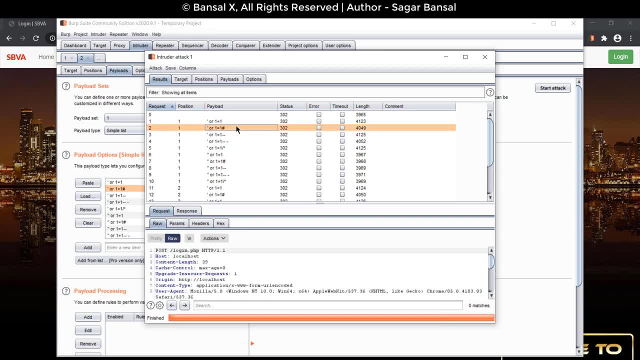 You see the one which we give, Okay, And then there are all the payloads that it has tried. For the position one it has tried this, Then for the position two it has tried this over here. But how do you define which one worked and which one didn't? 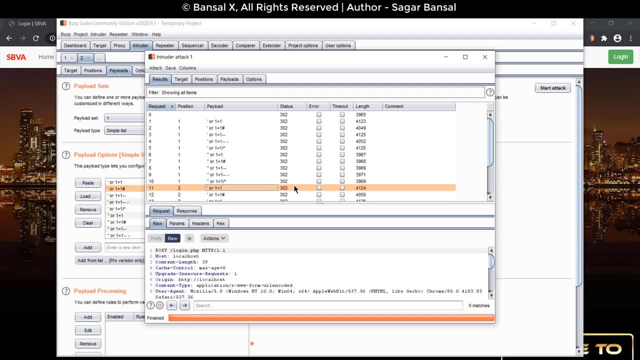 Well, you may go ahead and see what is the difference in these requests. All of them are having the same response code. I don't see any error or timeouts. but here in length, you see all of the lengths are different. You can go ahead and click on response and render and you can see what was the response. 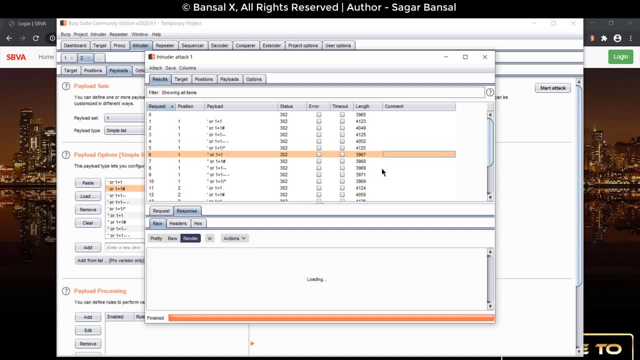 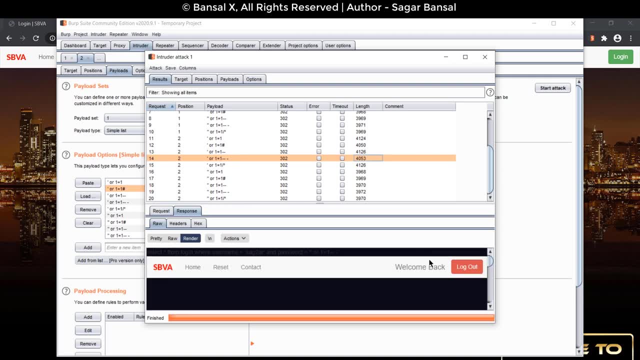 Of the request. None of these worked. However, if we see these four thousands, you see it has worked. So now these 4,000 requests are all working, but there is much cleaner way to do that. I'll just close this. 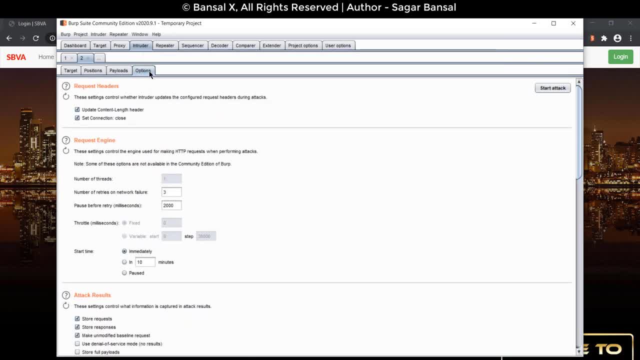 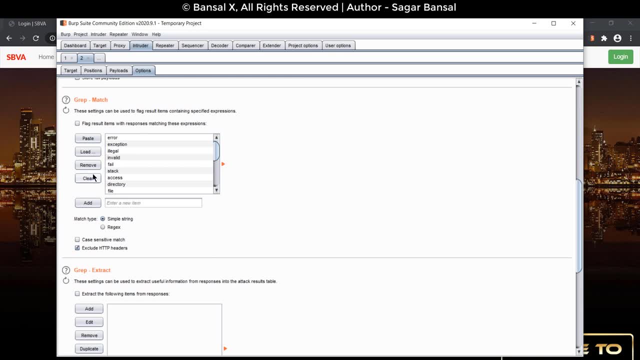 And instead there is fourth tab here, which is options. I'll click on this And options. there are many, but we can set this grep match option. Just clear all of these, Make sure this flag is ticked and add something like welcome. 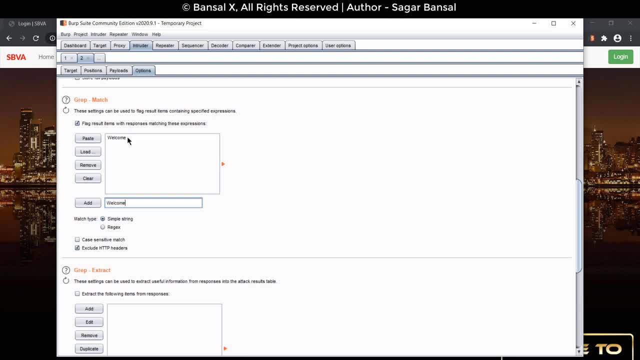 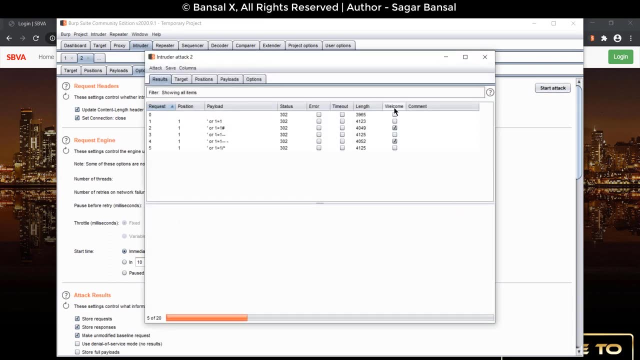 Press add And now it is set. The reason I have added welcome is I want to flag all those requests which have the word welcome. So basically, when I start this attack now, You will see it will start flagging the requests which have the word welcome. 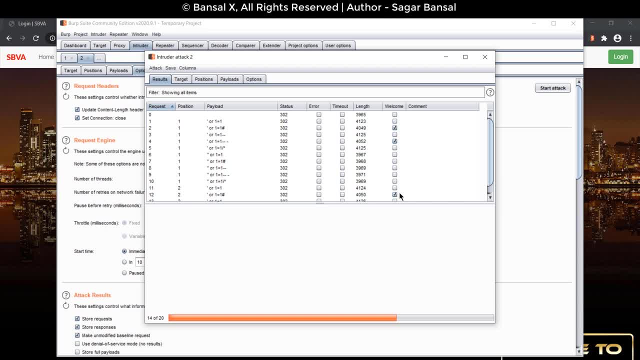 Just like this one and this one and this one. Now, once the attack is finished, which just happened, I can go ahead and filter it with the flags. So all of these four requests are the one which are resulting in a successful SQL injection. 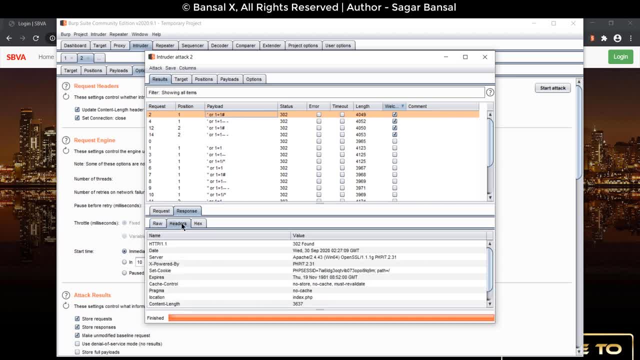 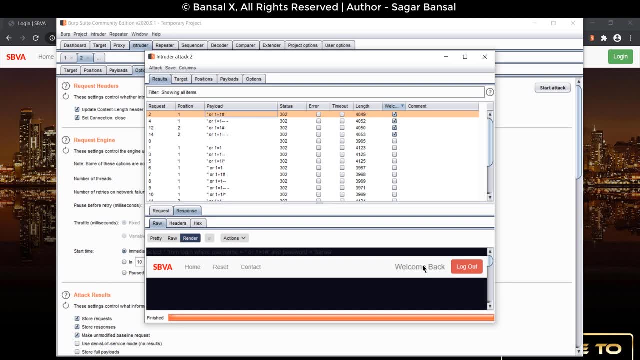 I can see if I go to response and render And render- This is the word which I just filtered for. When there is successful login, it says welcome back. So I just flagged any response which has welcome word in it. That is why we are getting these flags. 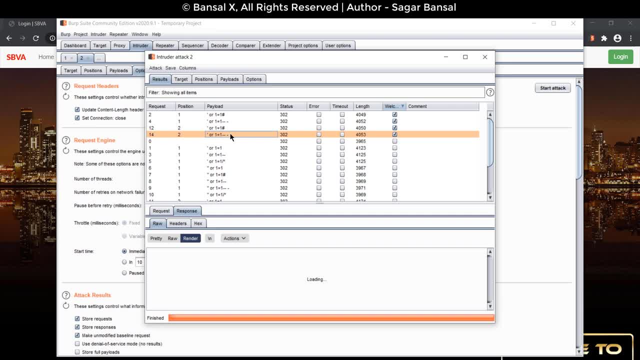 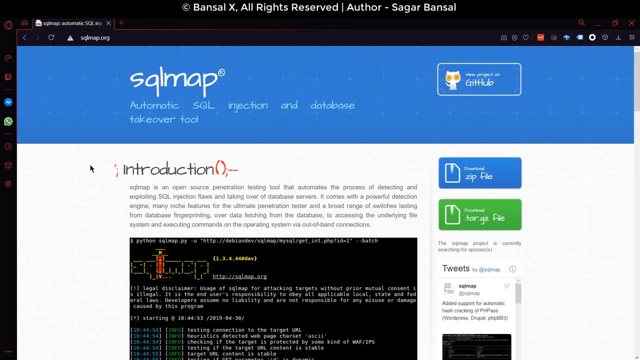 And now you know that these four payloads will work for your SQL injections. That is how you use semi-automated tools to uplift the hard work and do SQL injections, Using fully automated tools for SQL injections. Well, there are certain cases When you have to test an application which has thousands and thousands of pages. 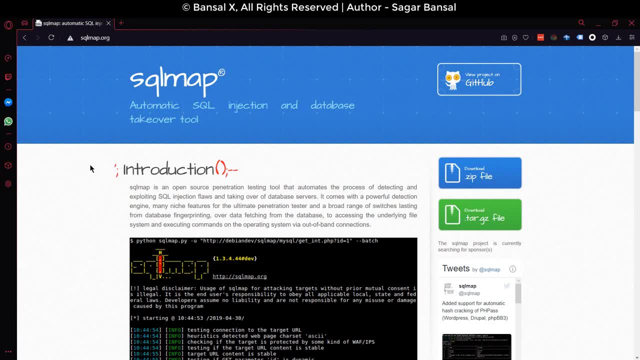 Even semi-automated tools cannot work for you. In those cases you may want to run some fully automated tools, just like SQL map. You can go to sqlmaporg and download the zip file. Once you have the file, extract it to any location you want. 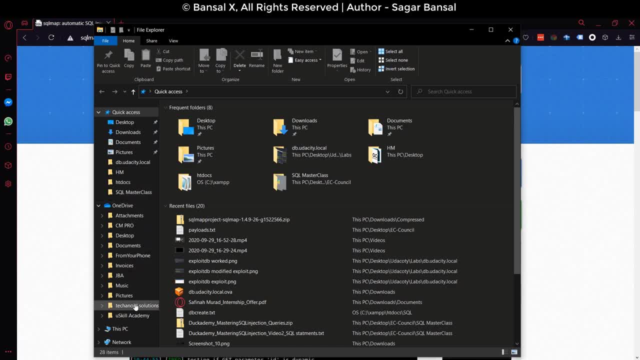 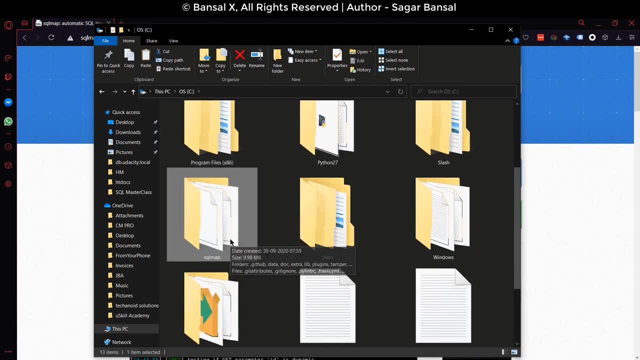 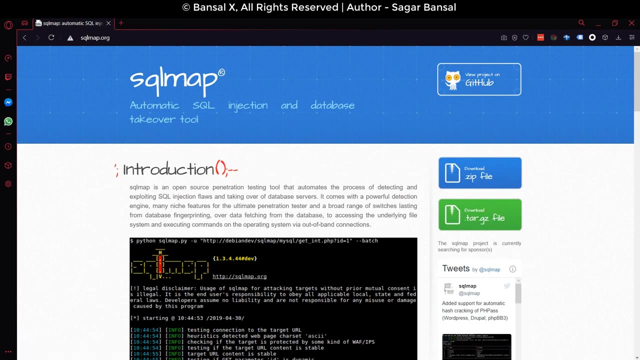 In my case, I have extracted this file on my C drive directly. Here you can see a folder, sqlmaporg, And there are all the files which you get in this zip which you just downloaded. Now just go ahead and open a command prompt, or a terminal in case of Unix. 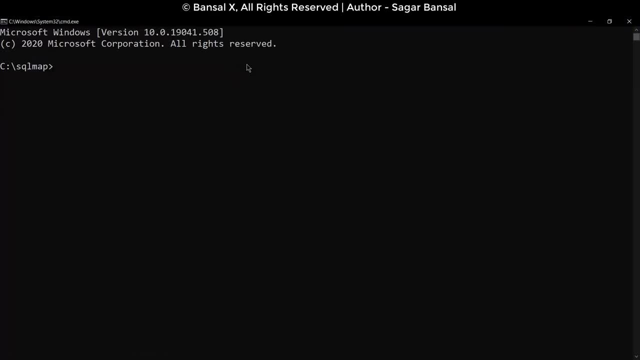 In the same folder And now you can just type python sqlmappy. Since I am using Python command, Make sure Python is already installed in your system. If not, go on Google download Python and install that. You can even do that from Microsoft store in case of Windows. 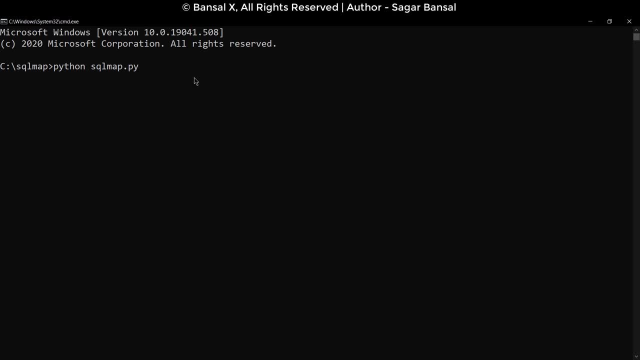 So I assume you can do that. Let's press enter And you will see it loads sqlmap and then gives me another missing mandatory options: d-u-l-m-r-g-e-c And all the other stuff. That's all fine, Just click enter. 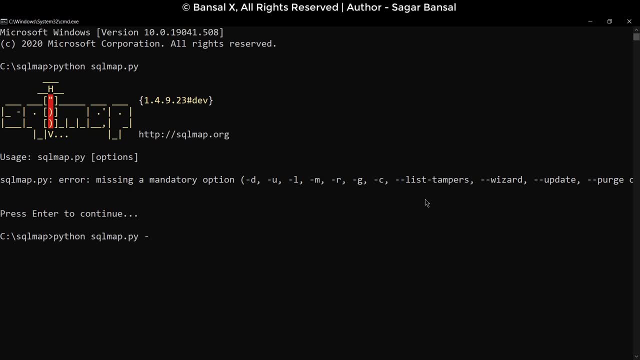 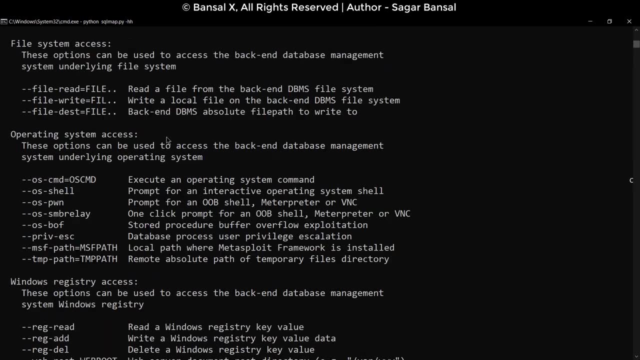 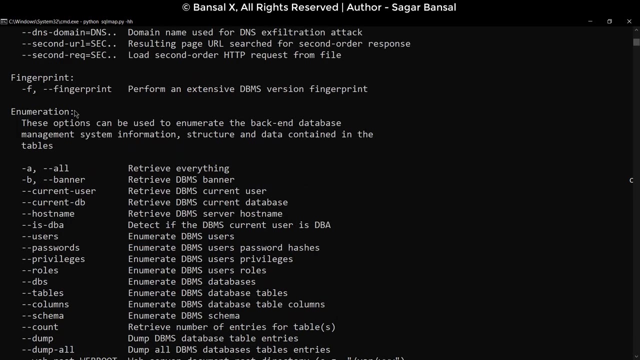 And now, instead of sqlmap, just give it an option called dash hh, which is extended help. As soon as you press that, you will see a lot and lot of options which you can use in sqlmap to do fully automated SQL injections. The first one which you need to understand is, of course, the url. 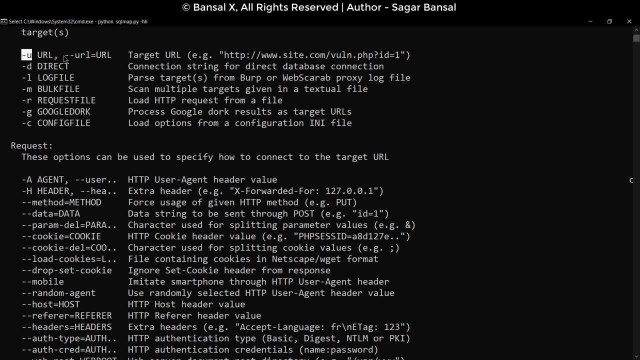 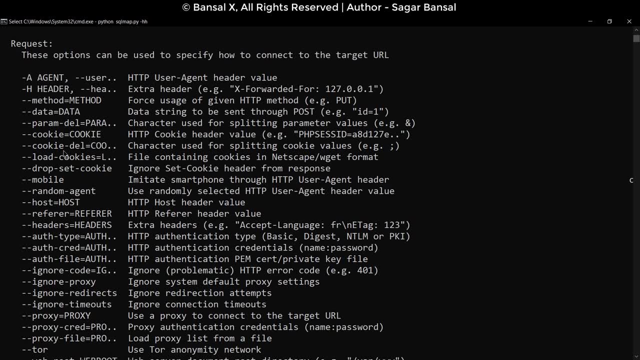 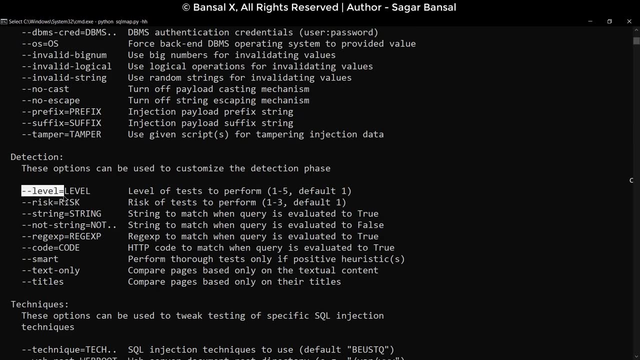 There are a lot of options. right There you go, Dash u dash url To give a full, automated SQL injection. Here you go. A specific target Then. the second which you need to understand, a minimum one, is the risk level. Here you see the level. 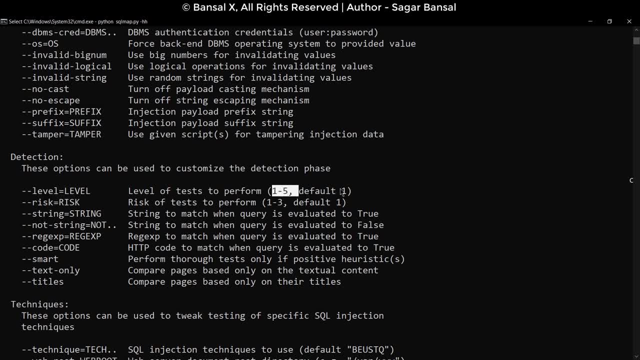 Level of tests to perform: One to five, and default is one. When you want to do complete testing, you would use the level five, not level one. The reason of having these levels is that maybe we just want to test something in a low level. 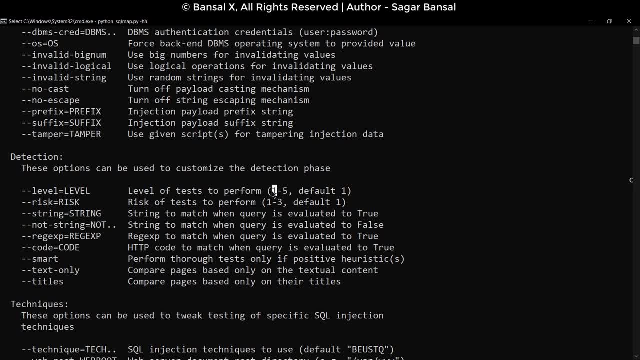 And we have a low bandwidth on our database. So if we use all the tests, we may crash the database. Same thing applies to risk, When you want to keep the risk of crashing the database, corrupting the tables and even getting caught while doing a pen test. we don't want to do all of that. 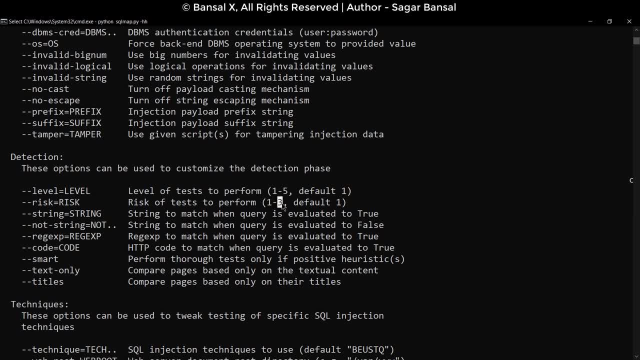 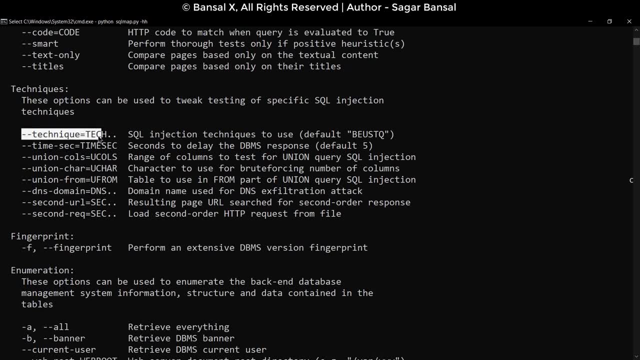 Keep it on one. However, you can increase it on three if it is a crystal ball test, Just like we are doing right now. There are many other options. You can even choose the technique, Which is dash dash technique, And you can choose between all the techniques. 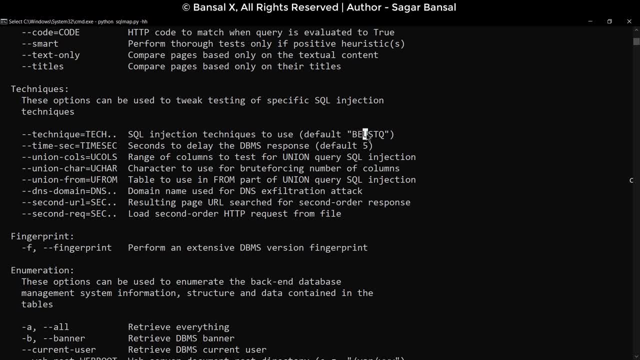 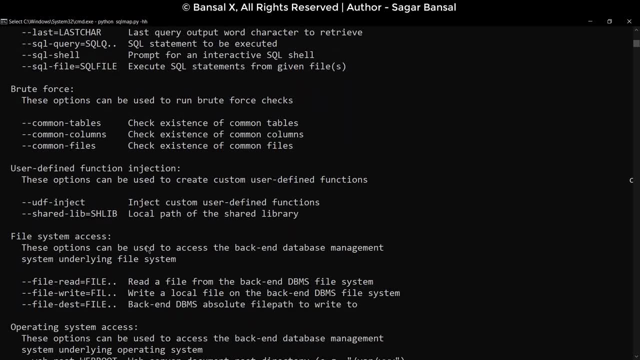 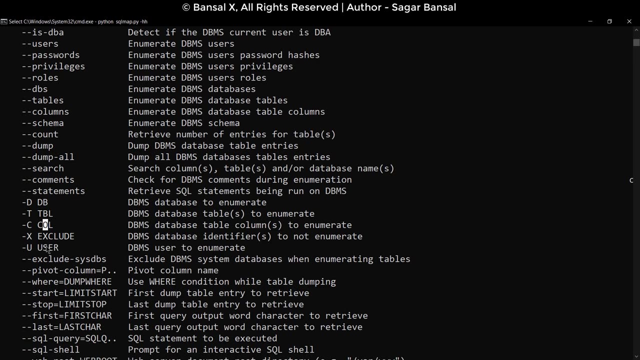 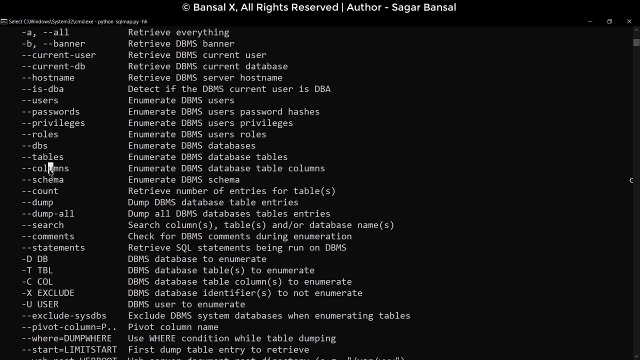 Like a Boolean based injection, error based injection, union based injection, etc. etc. Other options are also here. You can extract data if you want, Using database table column user to select the things And dash dash dps, dash dash tables, dash dash columns and dump. 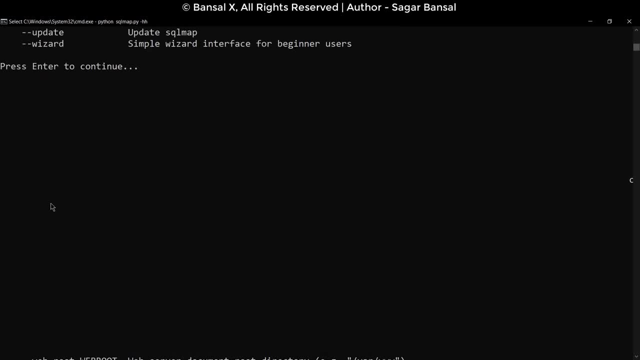 To extract the data. Let me show you an example here in practice. So I will go ahead and use dash u http localhost slash login dot php And I will give it a risk rating of 3. And level as 5.. Let's press enter. 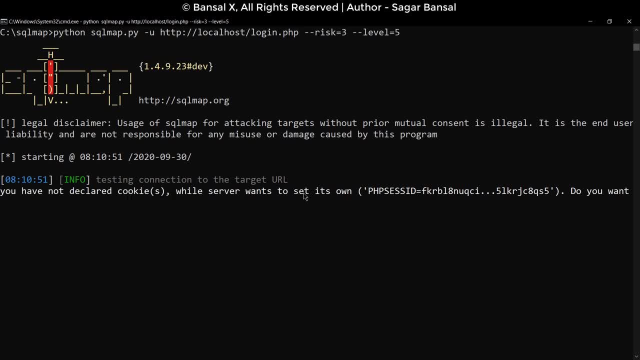 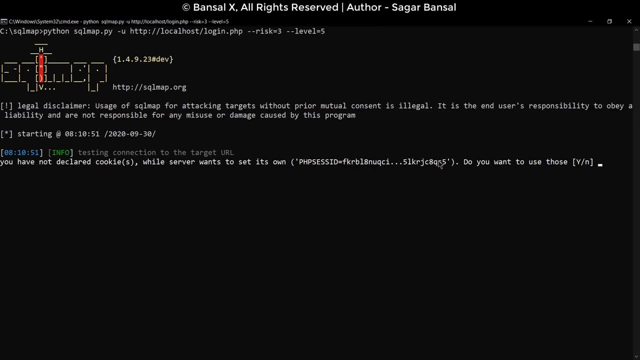 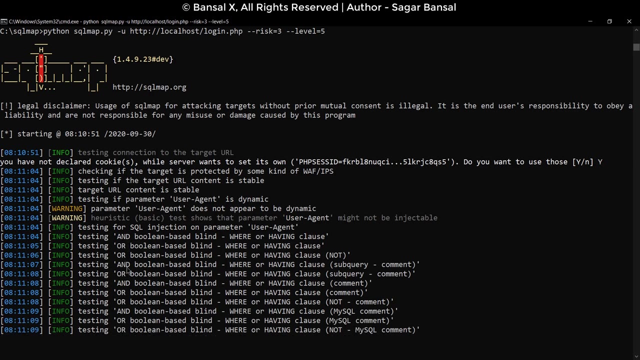 Now you can see you have not declared cookies, While server wants to set it on cookie this one. So do you want to continue? Yes, that's fine, We can take this cookie. Now it's testing SQL injection Or based. You see, Boolean based injections are being tested first. 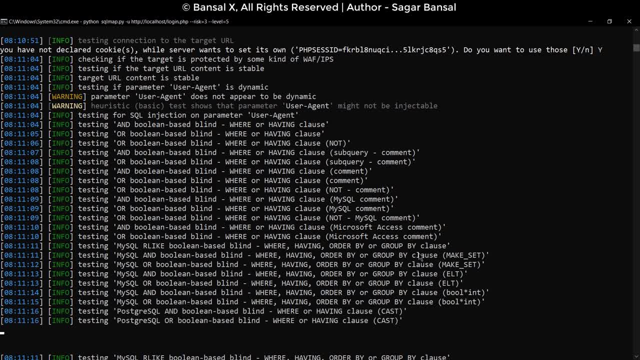 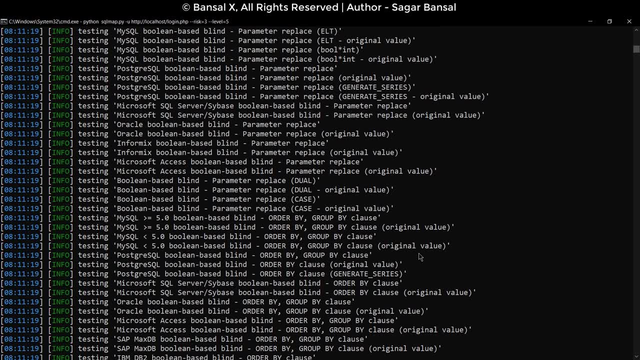 Then, once it is done with Boolean, it will start with some other tests, Like from union based. So it's going to do all the testing for us automatically. Now it's testing if the MySQL is less than this, more than this, using Boolean. 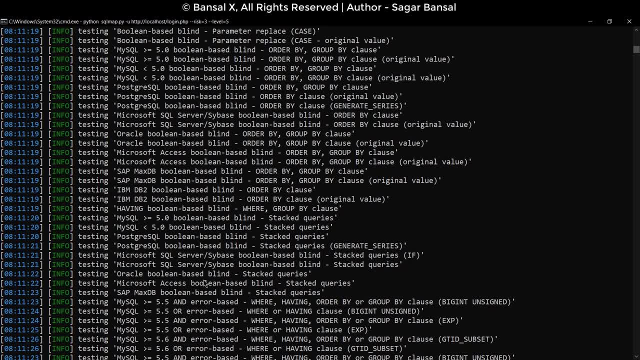 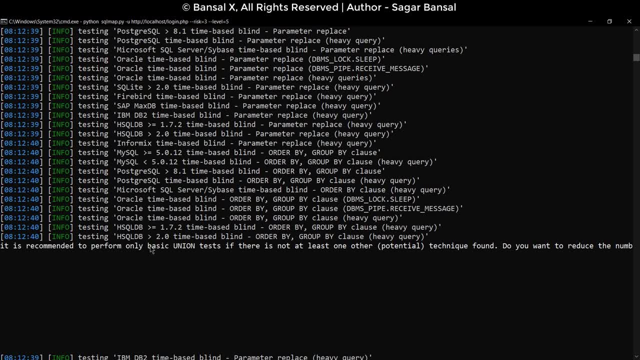 And PostgreSQL says testing the version of the database right now. It's going to take some time. Let's leave it till then And you can see it is asking us. It is recommended to perform only basic union tests if there is not at least one parameter. 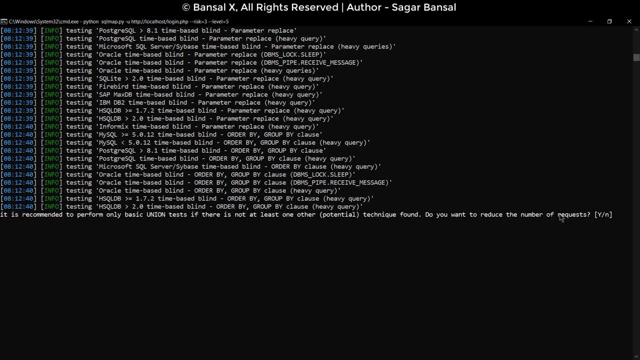 one potential other technique found. Do you want to reduce it? Reduce the number of requests? Well, this is going to reduce the number of tests which we are doing By reducing the number of level And in this case, I am going to allow this because I don't want to wait for such a long. 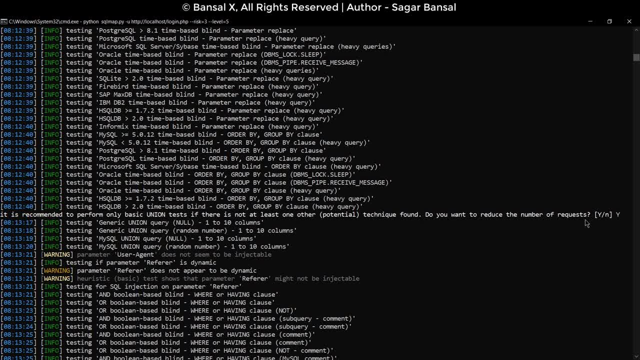 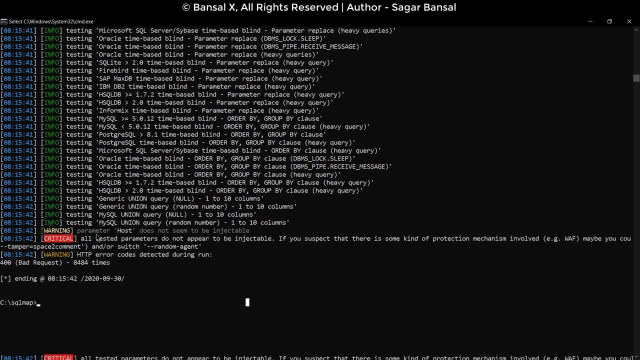 time when I know there is an SQL injection In a real life situation. you may not want to allow this and reduce the number of your tests. Now you can see SQL map ends up with an error saying nothing is injectable. It was not able to find any SQL injections with R. 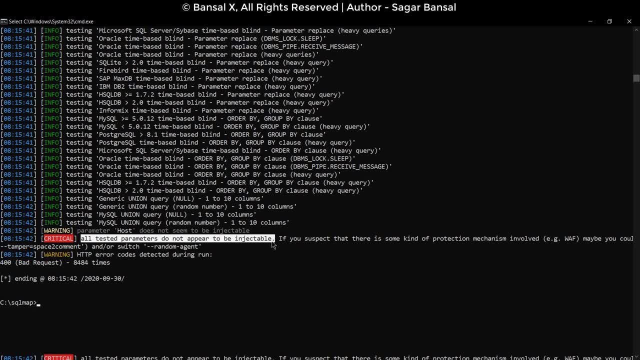 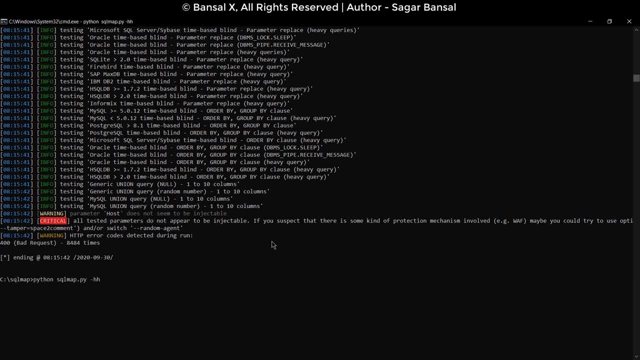 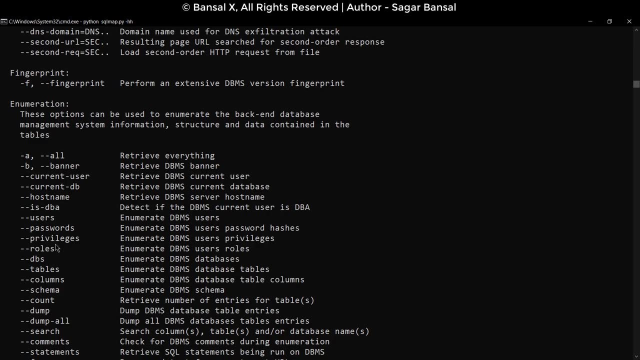 That is fine, it happens. There are many things which you can do to fix it. You can provide it with the fields to inject. So if I show you the help again, you will see there are certain fields which you can inject by putting dash, dash data. 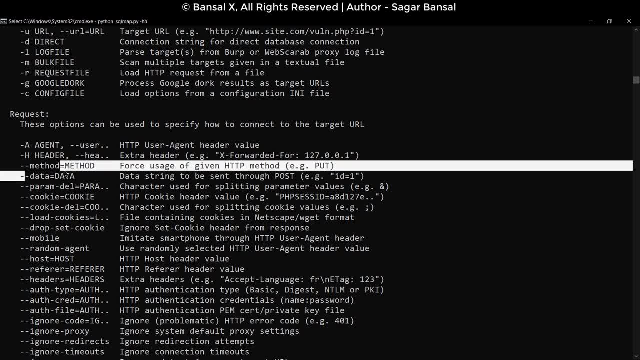 So let me see where they are. Here you go, dash dash data. You can tell it that. go ahead and inject it in this specific field by selecting dash dash data. This can be complicated for some people who do not know HTML, CSS, JavaScript, because 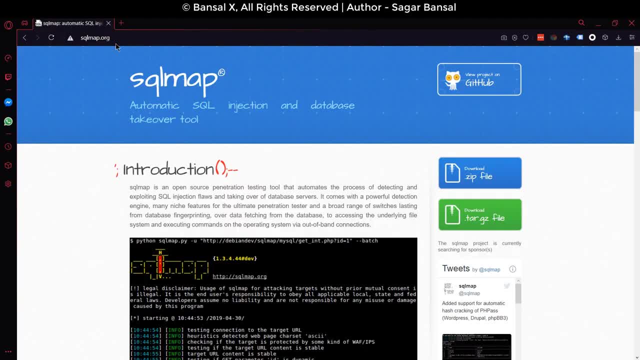 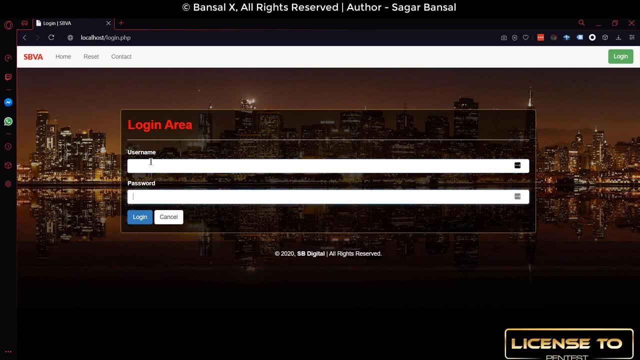 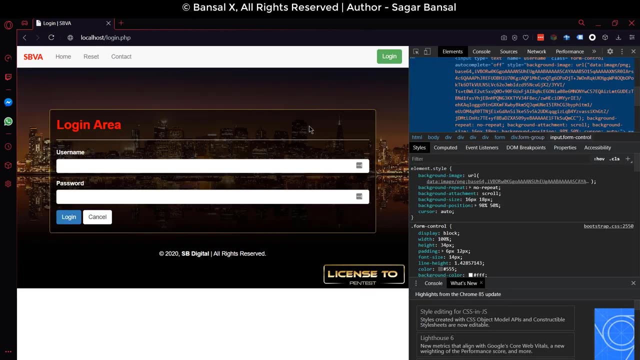 you will have to find which field are we injecting the data in. In our case, we are injecting the data in these fields: username and password. But you need to know the name of these fields So you may have to inspect the element and you may have to find that in this HTML or 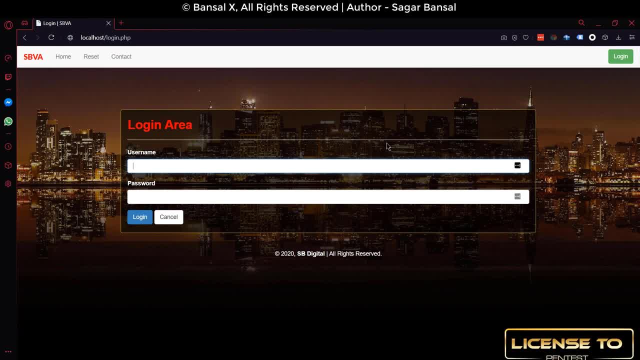 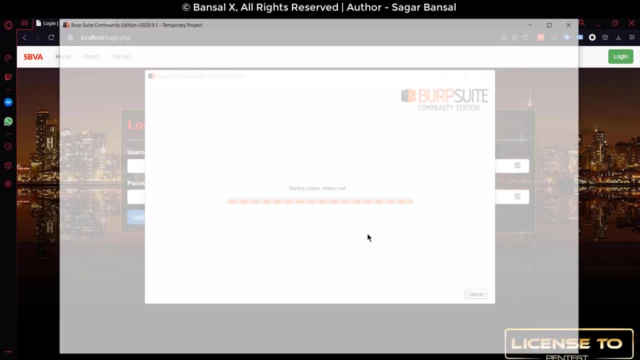 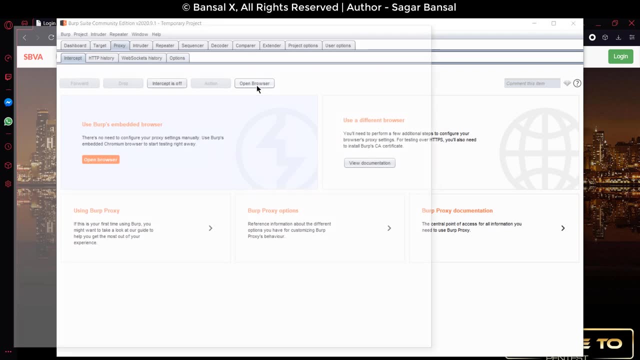 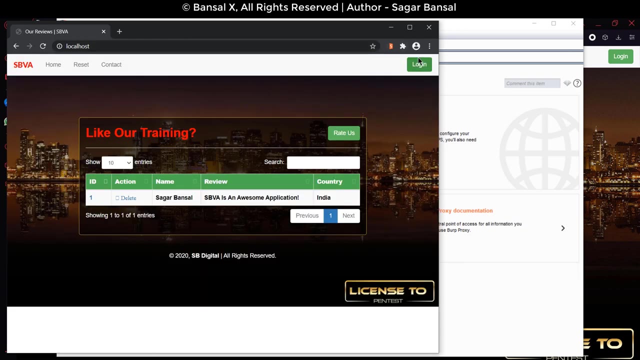 you may want to intercept the request and find it there. An easy version will be: Just use burp suite, go ahead and start a temporary project. open your proxy, start your browser, go to localhost, go to login and here, go ahead and give it something like: 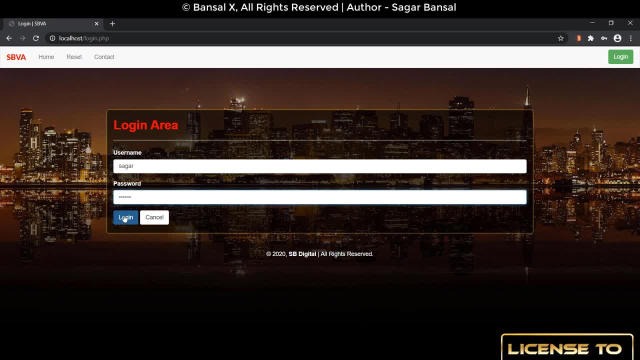 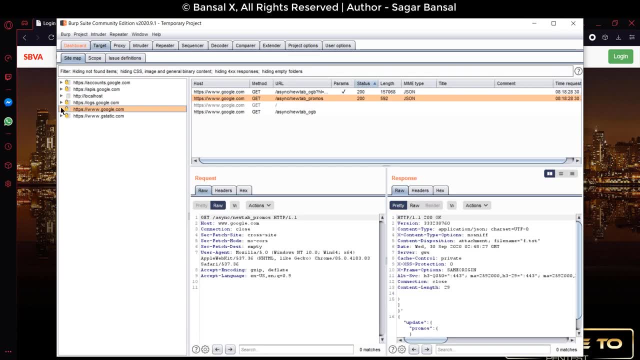 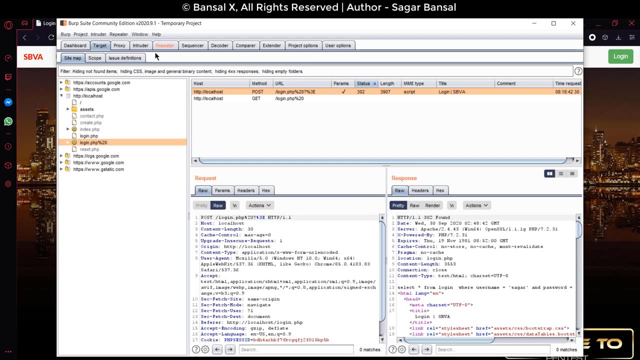 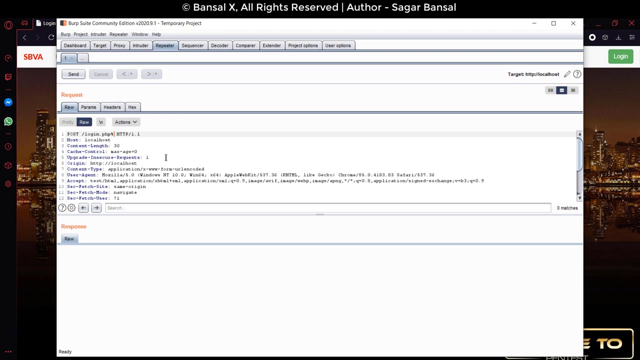 sagr. sagr1.. Login. I don't need the browser now. I will go to http history or in the target and I'll take this request, send it to repeater and I'll just clean this request a little bit because these characters may cause problems. 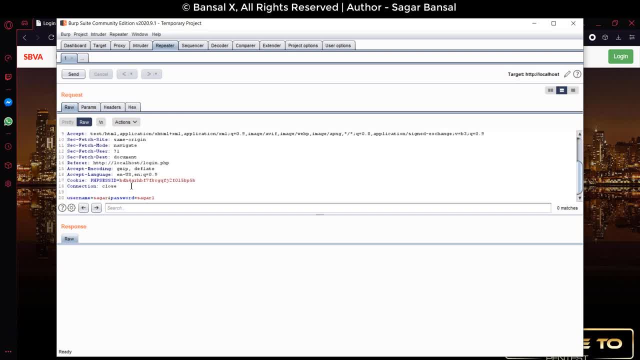 So this is loginphp request, which is taking two parameters: this one and this one. Instead of these parameters, press a asterisk sign. Now, once you add this asterisk sign, this is called sqlmap payload marking. Now I can just save this to a file. 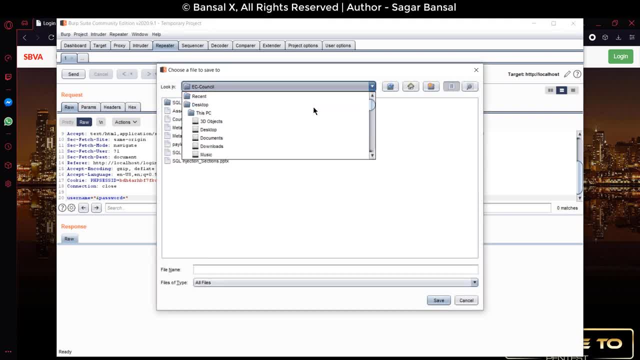 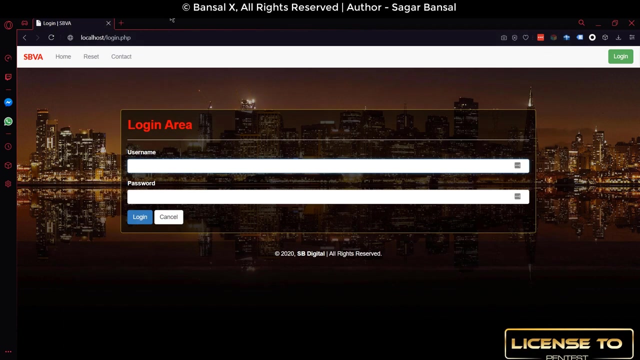 I'll save it in my C drive, in my sqlmap, the same directory where I'm running it. I'll save it, for example, any name like requesttxt. I'll just say save, Save. I'll close the burp suite. I don't need it now. 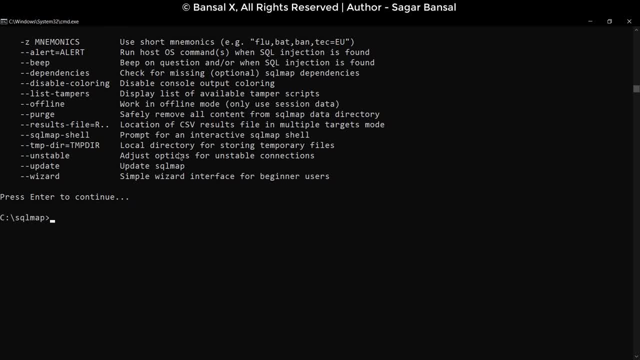 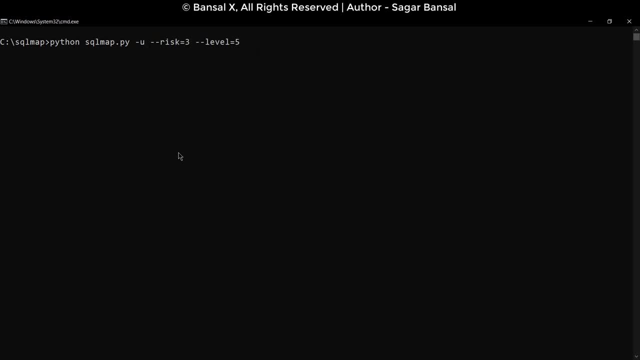 And if you go ahead and run this this time, instead of giving it a URL, you can specify the request file you created by dash r- requesttxt, And you can go ahead and give it the levels, And let's go with the default this time, because that will be faster. 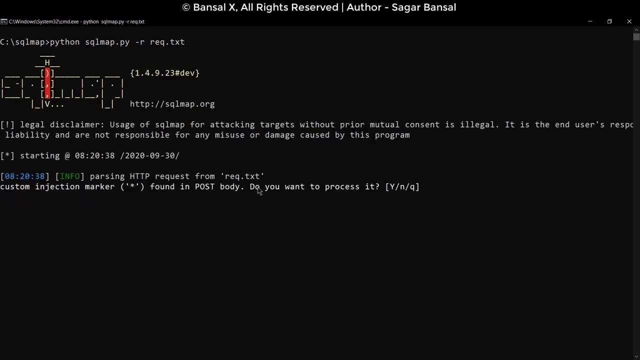 And it'll say: custom injection marker found. Do you want to process it? Of course, That's why we created it, And it says redirecting to this. Do you want to do that? Yes, we want to use http//localhostperdatloginphp. 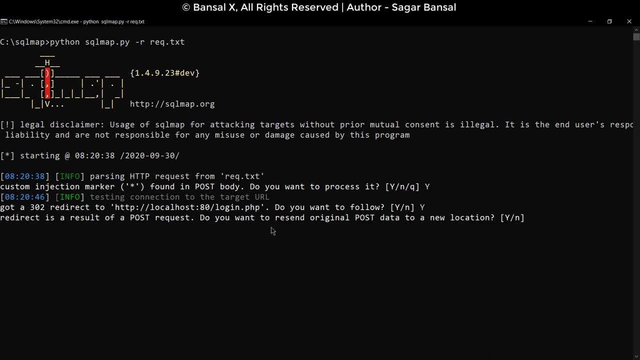 Yes, that's what we are testing. The result is a POST request. Do you want to resend the original POST request? Yes, we want to send the original POST data in the new location. Yes, we want to send the original data in this new location, which is loginphp. 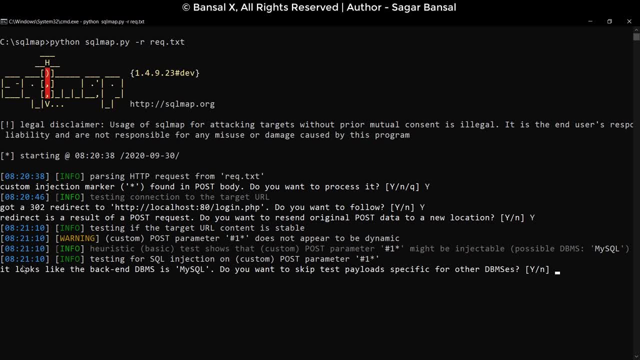 Okay, it looks like the backend database is MySQL. Wow, it just found that right. Do you want to skip testing payloads for specific other databases? Of course we don't want to test others, because if it is MySQL, then yes, let's just test. 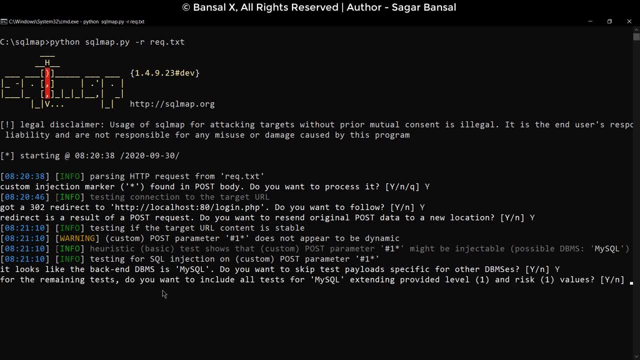 for MySQL. For the remaining tests, do you want to include all the tests for MySQL, Extending the level 1 and the risk 1?? Well, you can do that. In this case, I'm skipping it to make sure we complete this lecture on time. 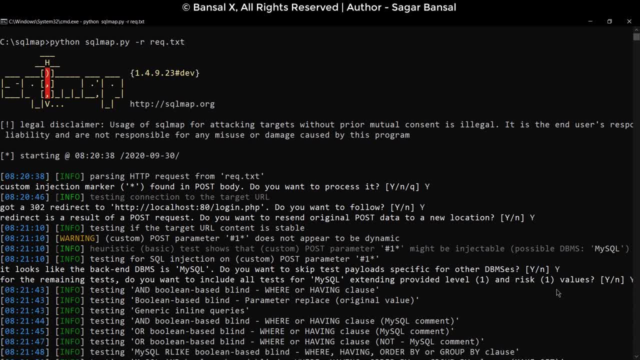 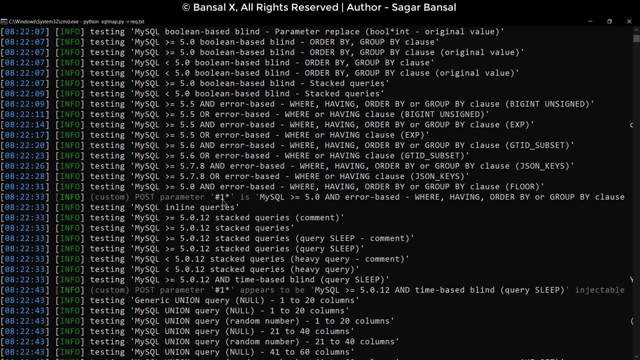 Let's see if it gets us the result this time. Now you can see over here custom POST parameter number 1.. So the number 1 marker which we put in the username. it is testing that right now And it says POST parameter number 1 is vulnerable. 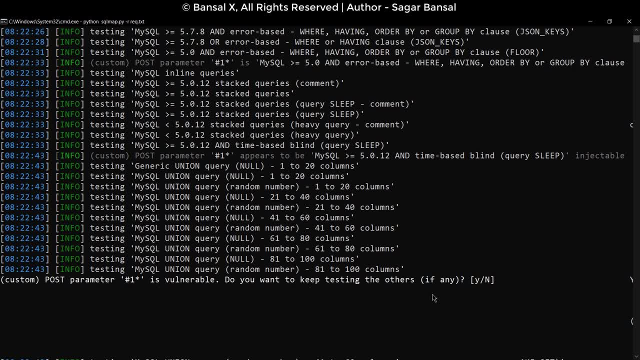 Do you want to keep testing? Yes, You can keep testing others. You know, in the real life situation you can test it. And the second parameter is also vulnerable in our case, but I'm going to skip it right now because I found a vulnerable parameter. 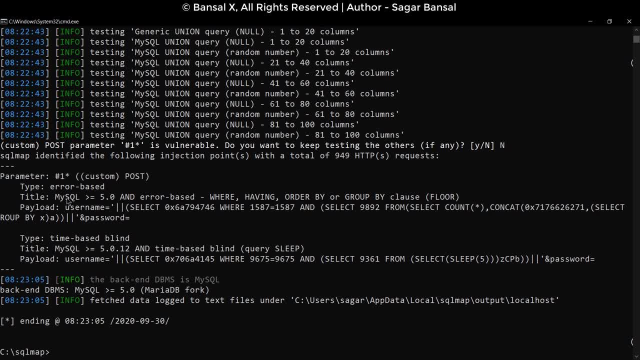 So that's all good. Now these were the payloads that it has used for number 1.. You can see username and then a single quotes and then select something, something, something where something subselect something from, subselect count. 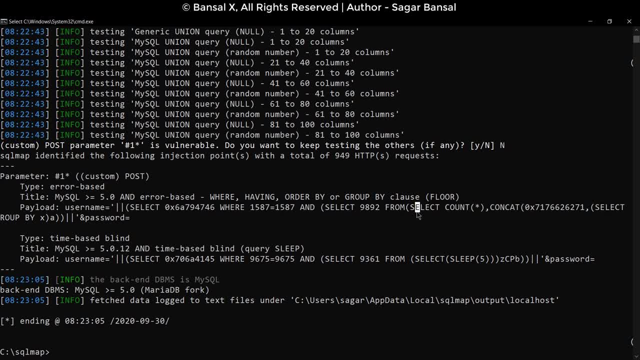 It's a long payload. I don't think I would be ever able to write this count. It's a kind of complex payload from my hand And that's where the automated SQL injection really stands out. You can copy this as it is and take it and find whatever data you want in the real website. 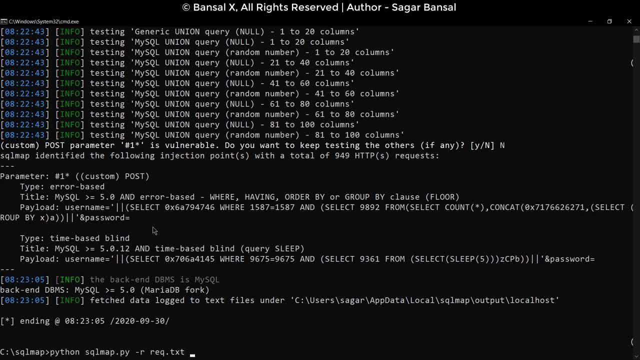 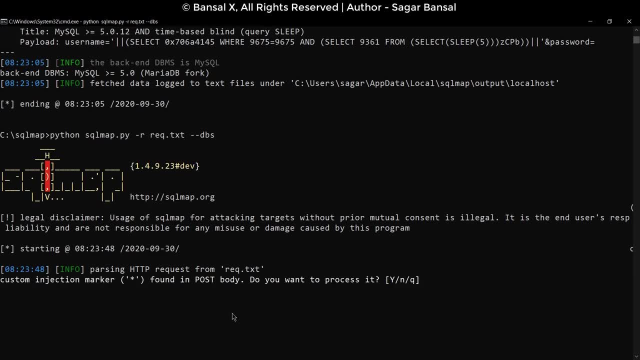 Or you can use a SQL map to do that work for you as well. So this time I'll say: you know what? find me the databases DBS. It'll find me the databases this time And it says: do you want to use the marker? 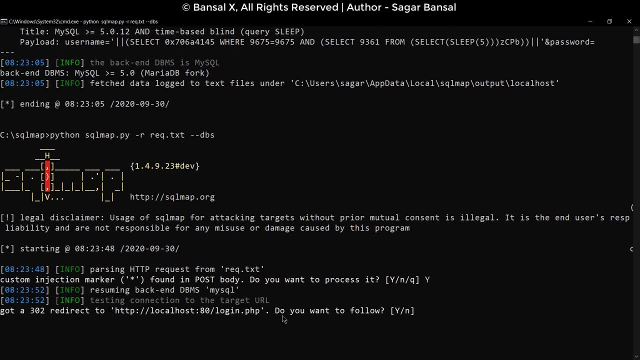 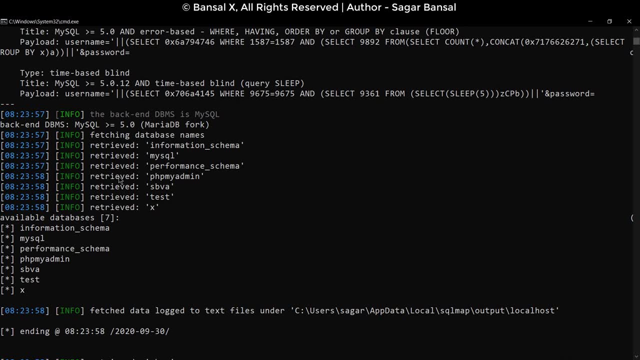 Yes, I want to use the marker And we got to redirect. That's fine. Yes, Use the data. And now it'll just give me the databases, because it knows that the first parameter is vulnerable. It has already saved all the data. 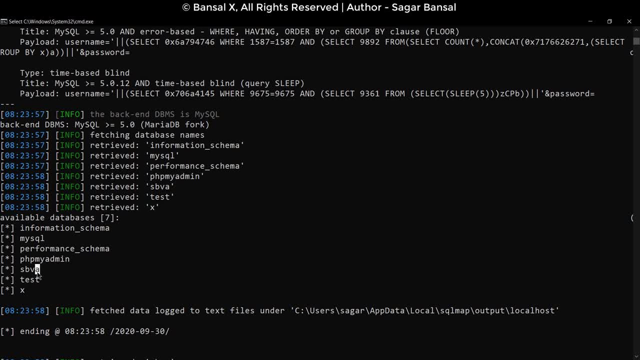 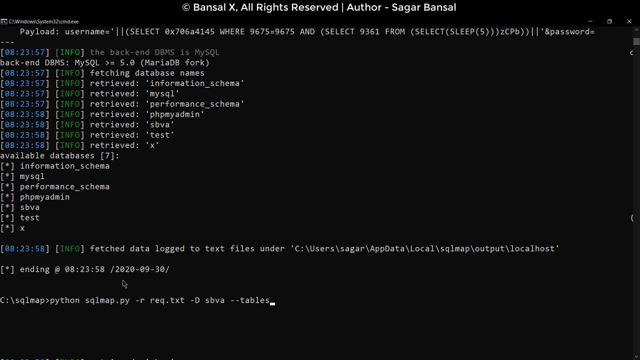 And here are all the databases I can find. let's say, I can select the database SBVA and I can find the tables Again. yes, yes, yes, And you see, we've got the database, We've got the database. 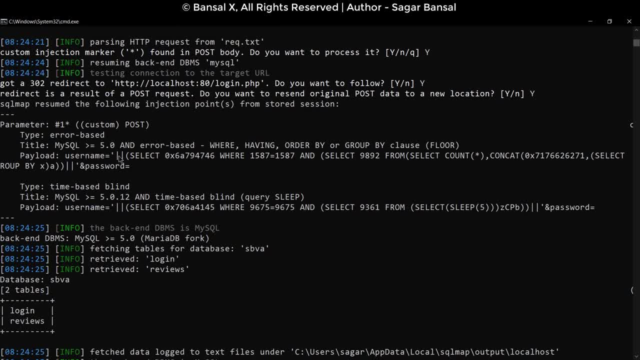 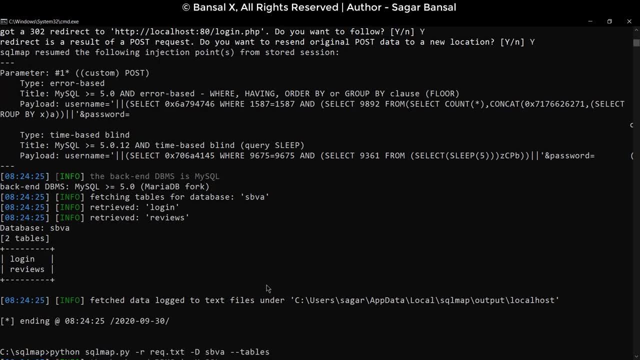 We've got the database, We've got the tables And these are the payloads that it is using, starting from here, ending here. Again, super complex stuff. I cannot write that Now. let's select the table, Let's say login. 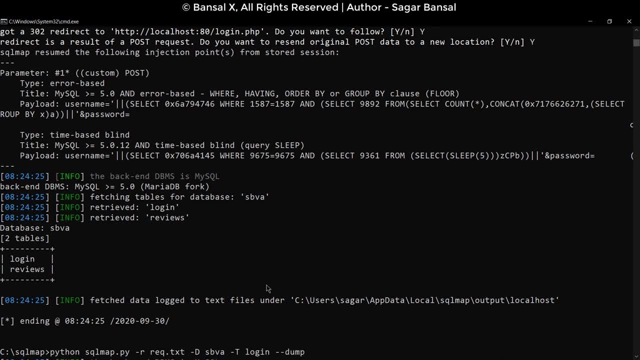 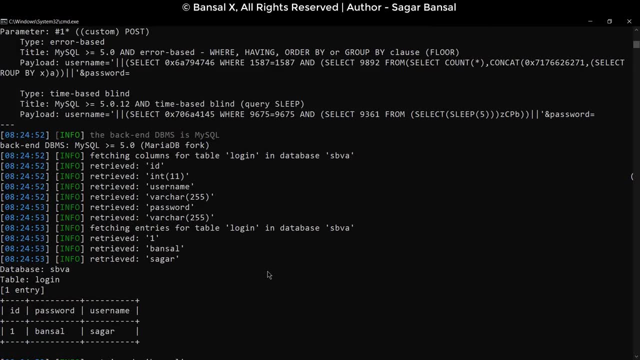 And let's say you can find the columns, but I'll just dump it as it is. So, yes, yes, yes, And there you go. We just dumped the whole table as it does, Instead of finding one column. we just dump it as it is. 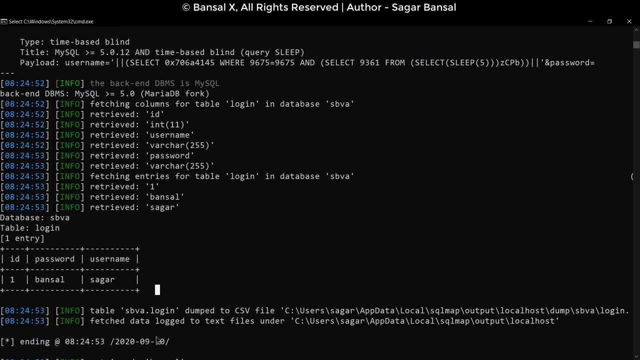 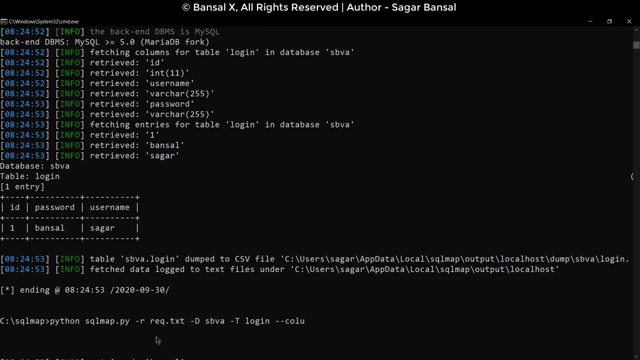 Instead of finding one column at a time, I dumped the whole table. If you want to find the columns also, you could have done that by pushing dash, dash columns, And then it'll just, you know, go ahead and find each column for you. 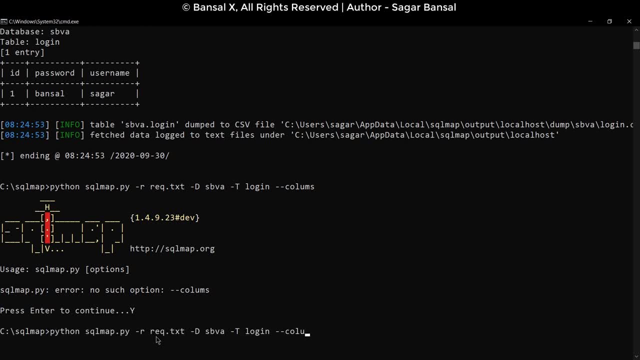 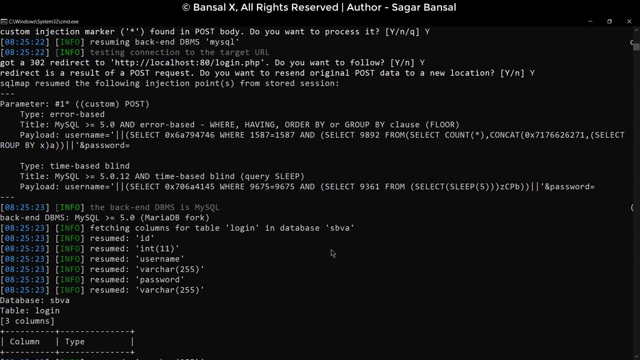 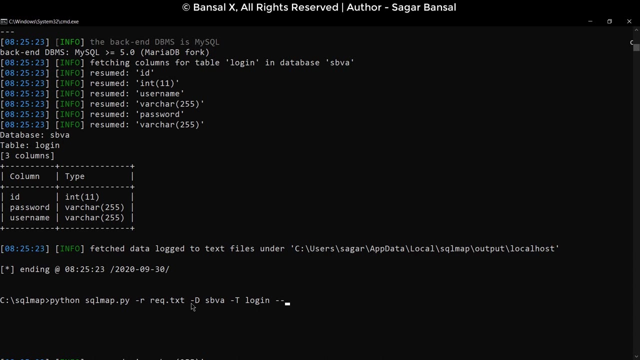 Okay, Invalid character. c o l u m n? s. There you go. Now it finds the columns And you can select a column and dump that. So you know, really depends like dash C and you know, like ID and dash, dash dump. 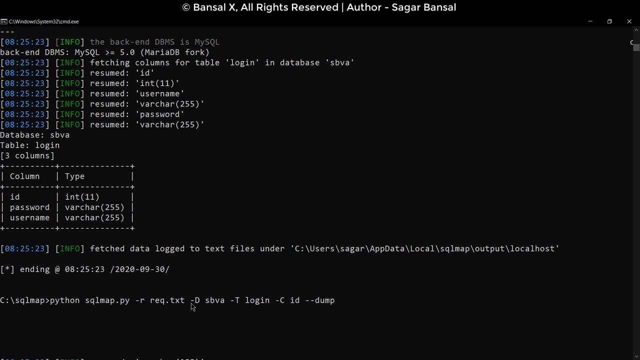 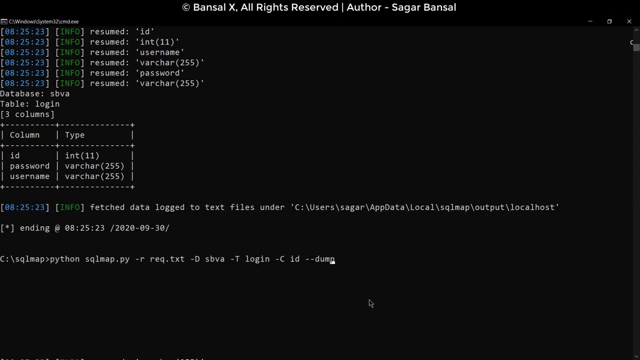 So in this case it'll only dump the column, or you can just dump the whole table by just ignoring this columns thing and just say, dump over here itself. So it really depends, you know. if the table is too big you may want to do column wise. 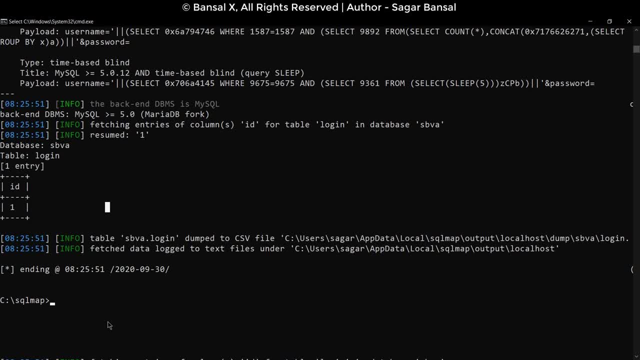 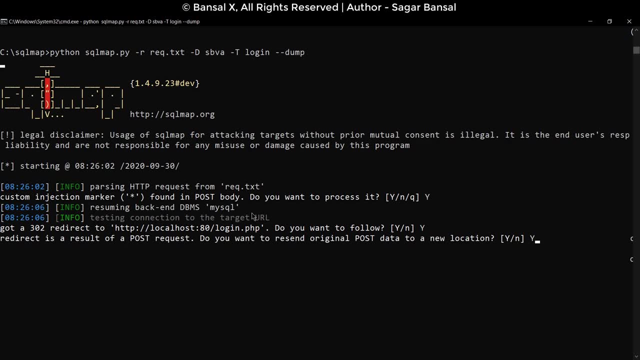 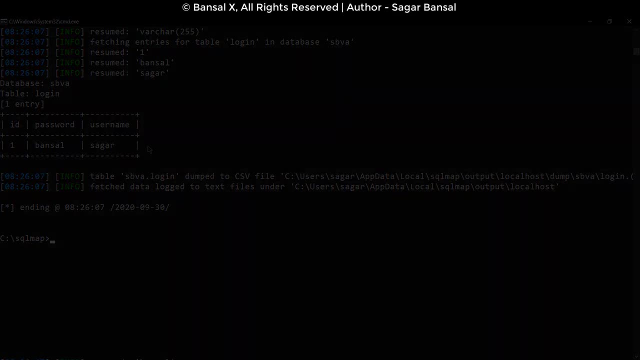 And here this will only dump the first column, as I said, but again, you can always dump The whole table. no need to dump column wise If you know that the table is small. So that is how you use SQL map to do automated SQL injections. 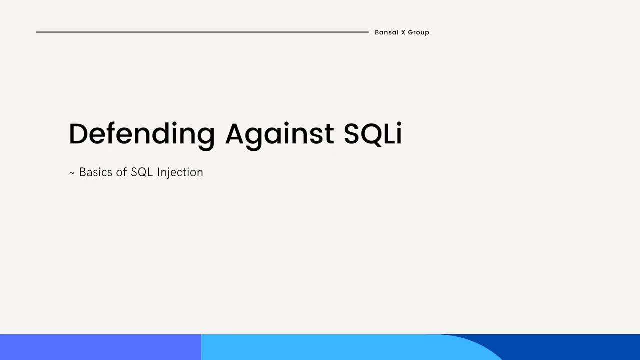 Defending SQL injections is not an easy task. That is the reason this old technique is still prevalent in the market. There are so many websites which daily get attacked due to SQL injection. There are many methods to do that Most of the security practitioners will go with. 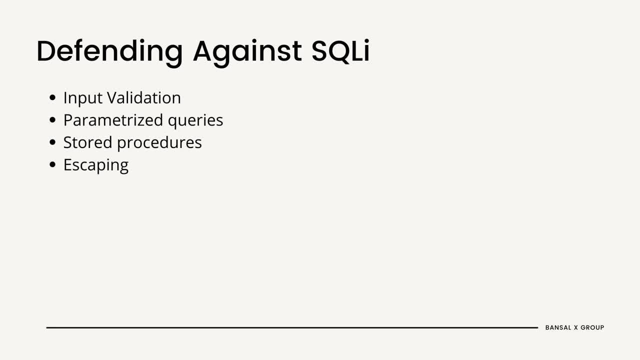 Code sanitization, which will include things like input validation, parameterized queries, stored procedures, escaping, avoiding administrative privileges, those kind of secure coding practices. Since this is not a coding course, I will not cover how all of these actually works. 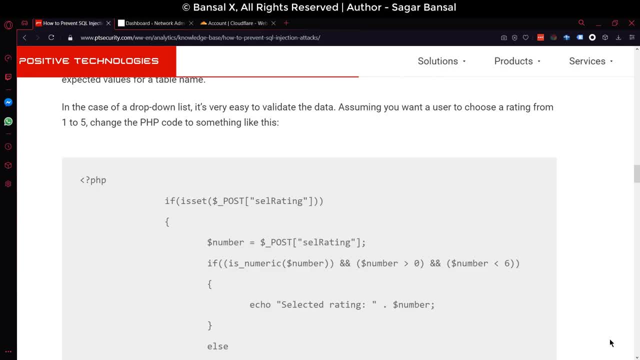 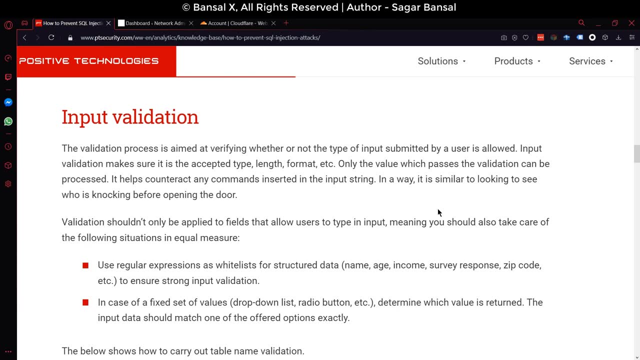 I can give you a reference to ptsecuritycom and they have a really good guide explaining how to securely code all of these things which I just mentioned. You can see input validation- They talk about it- and the code which you have to put and how do you have to put that. 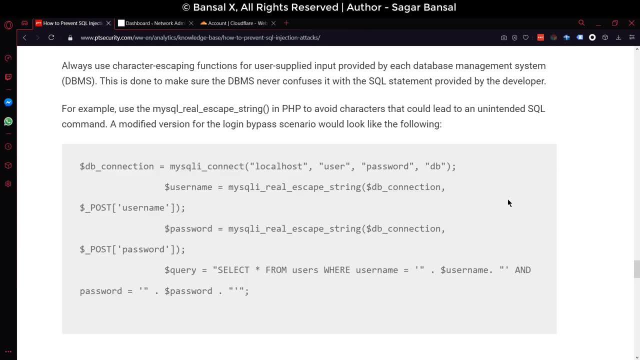 Parameterized queries, the code and how you have to put that. However, I will tell you my specific approach, which is also one of the best industry practices: Instead of just focusing on the code and focusing on the development side, you should focus. 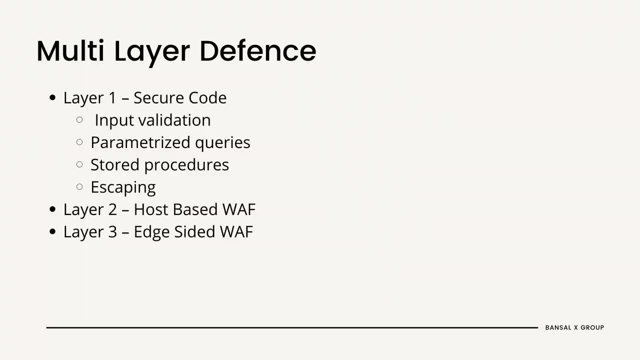 on a multi-layer defense. Now, the multi-layer defense works in a minimum of three different layers. The first layer, Of course. You see right now Which is the code, All of these techniques You put that You do, secure coding. 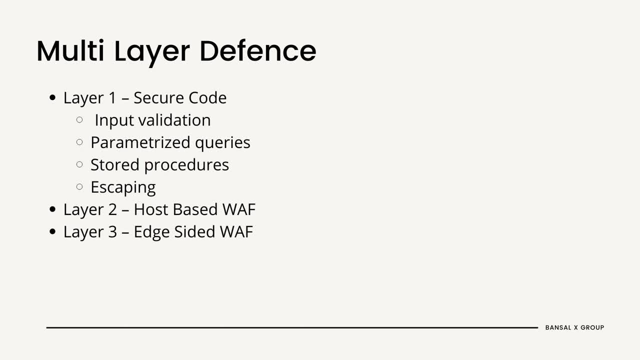 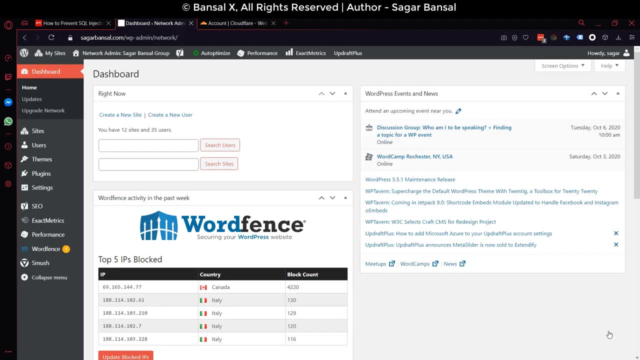 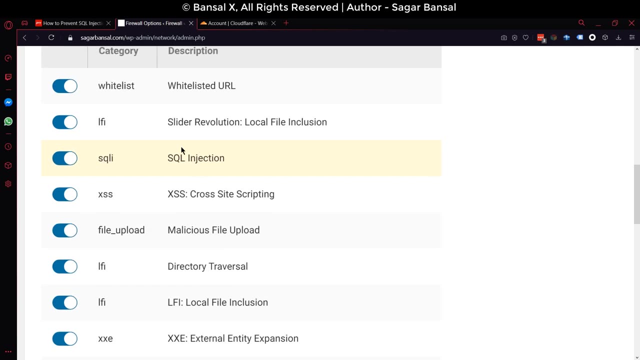 That is your multi-layer defense. layer one: Secure coding practices. Layer two is including a web application firewall. This is a WAF which runs on WordPress CMS. You can scroll down and I'll show you all the available attacks which you are defending against. 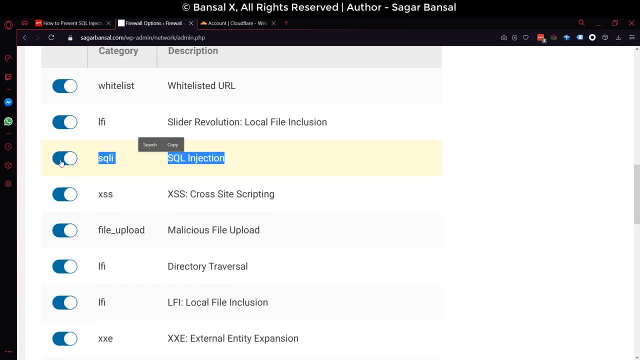 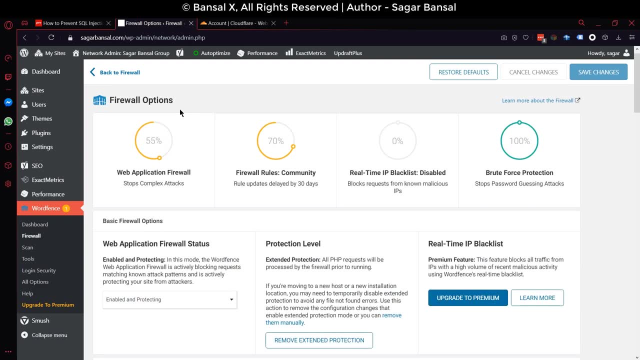 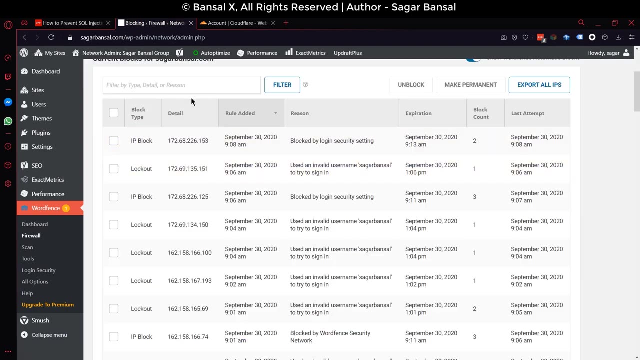 In my case, SQL injection is set on enable mode, So this WAF is going to stop any SQL injection attacks. Let me show you my logs, which will reveal a lot of IPs who have been attacking my site every single second. You can see there are a number of IPs and this is the current date, and I believe it's. 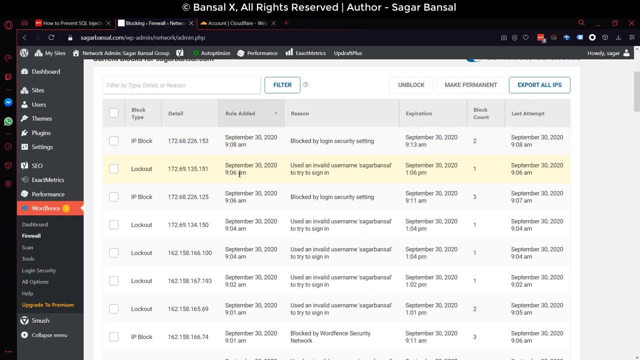 like, eight minutes ago, someone got blocked. 10 minutes ago, someone got blocked 10 minutes ago, 12 minutes ago, 14 minutes ago. This happens when you have a huge website and actually a network of websites just like mine. So all of these are being blocked due to certain reasons and the WAF is protecting that. 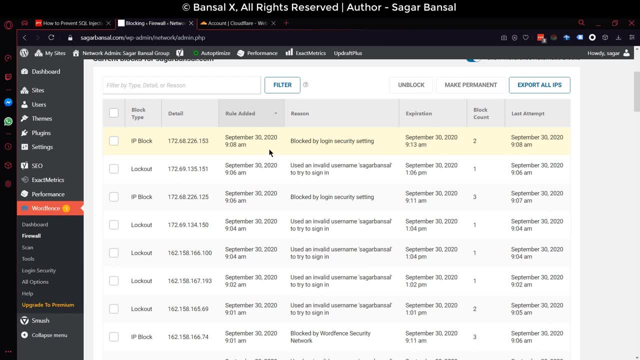 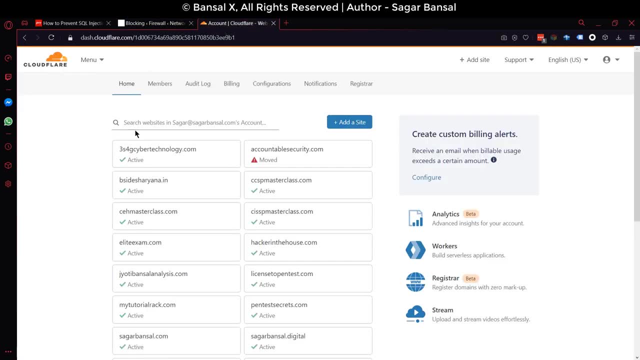 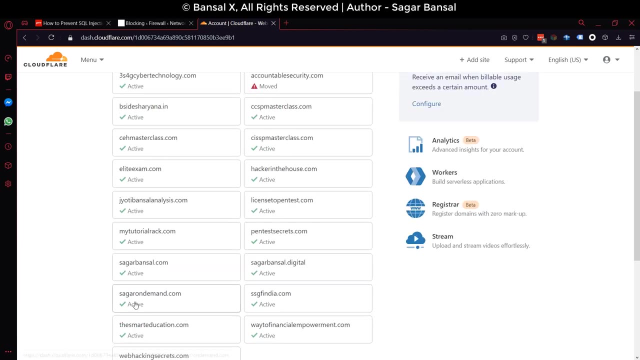 Well, that's your second layer of defense. The third layer of defense is having a WAF placed on the edge, which is normally the DNS. In this case, I use Cloudflare. On Cloudflare, you can add a new site by clicking on this button and configuring the DNS. 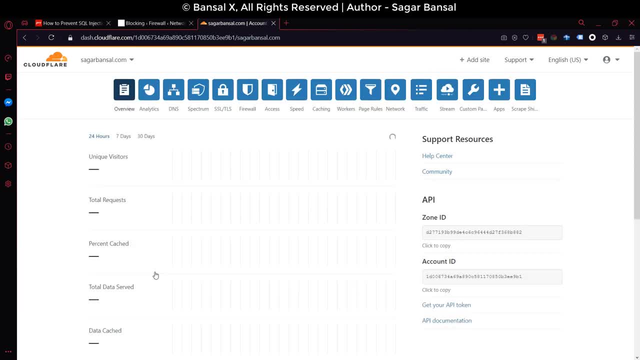 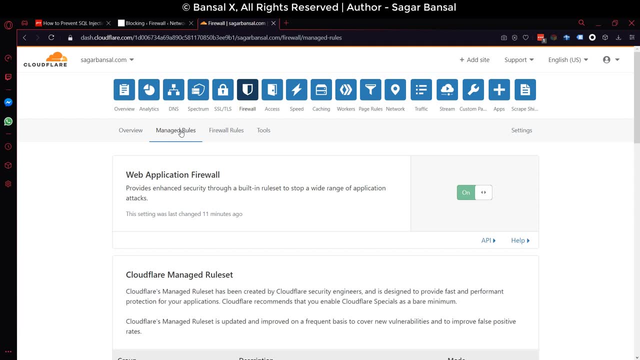 And in this I will open my site. Here I can go on firewall And I can go on the manage rules. Now again, this web application firewall is a paid product. It's not available in the free version, but I'm still showing you because that's how you. 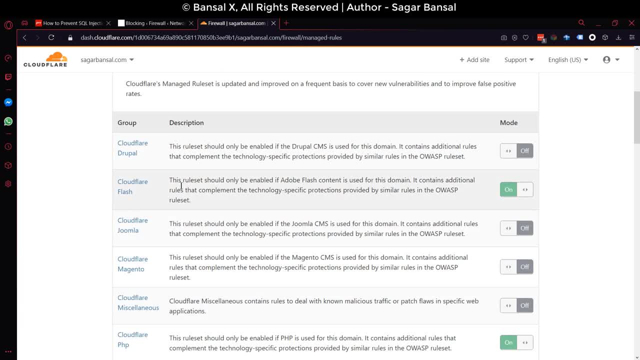 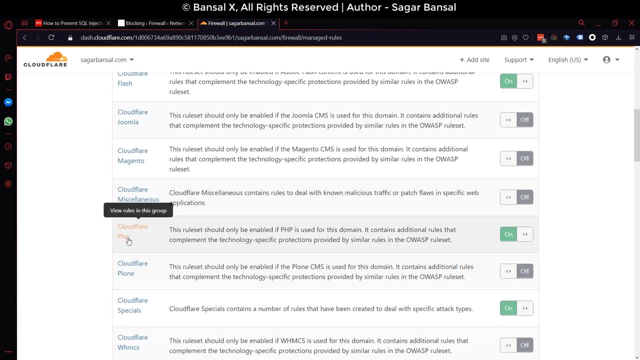 have to do it in the real industry. I can go ahead and see these rule sets and you can see I have selected some of them, which applies on me. So because my website runs on PHP, I have applied this rule and you can see over here. 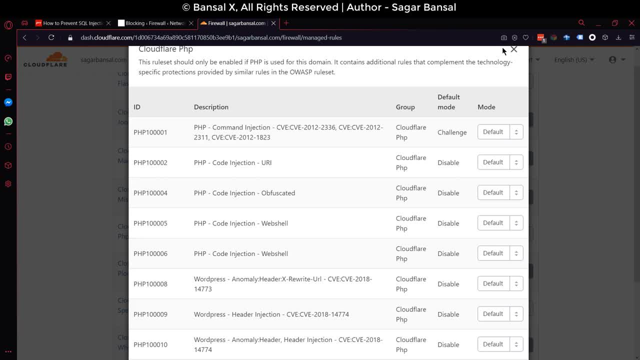 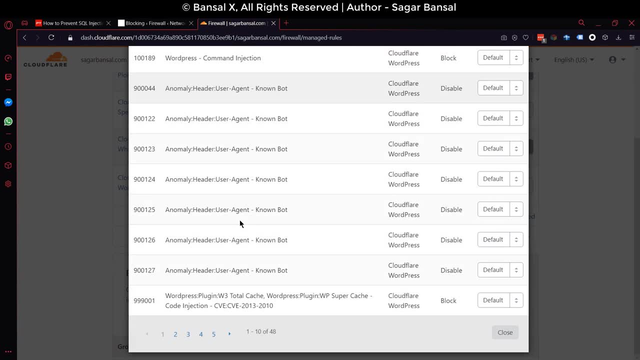 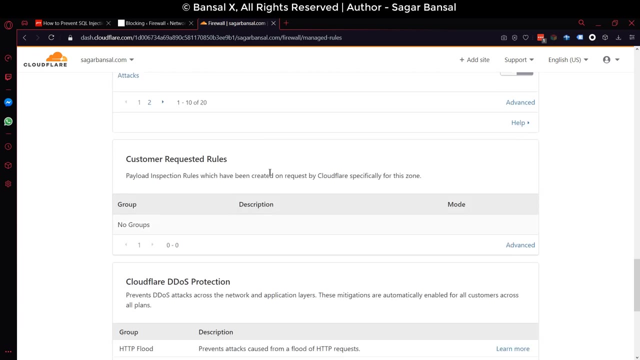 all of these rules are being protected against. Okay, Then I have applied WordPress specific configurations, which are all of these rules being applied on my website? Similarly, there are flash rules, and there are other stuff as well. You can see, it goes on and on, and on. 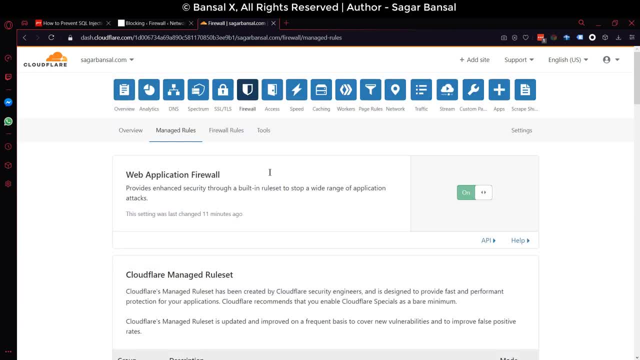 This is how you protect a device in a multi-layer defense. There are many more layers you can add. You can add an intrusion detection system, intrusion prevention system, an application delivery controller, a security orchestration automation response system. You can add a security orchestration automation response system. 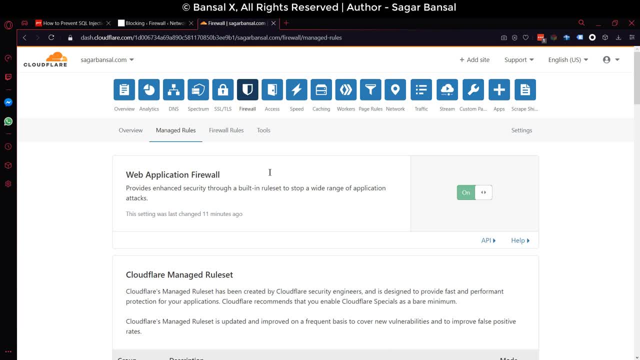